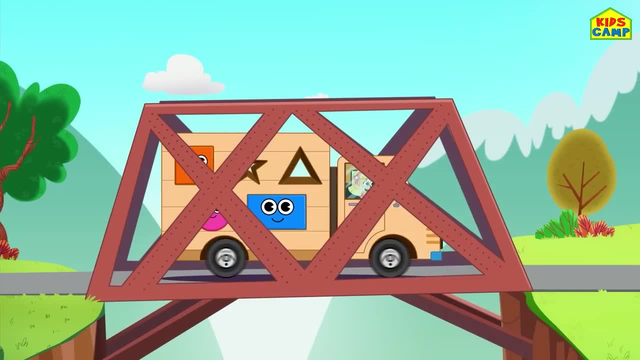 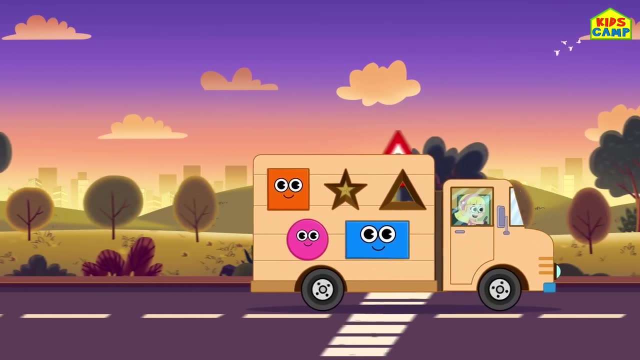 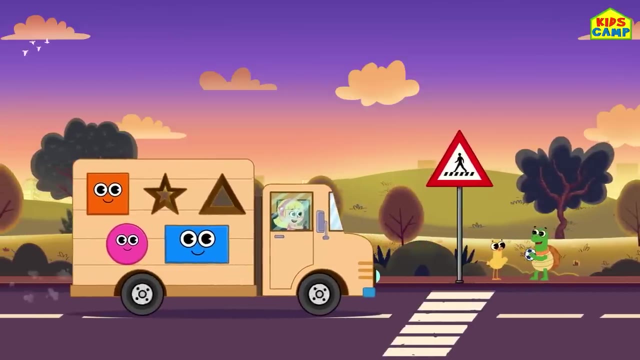 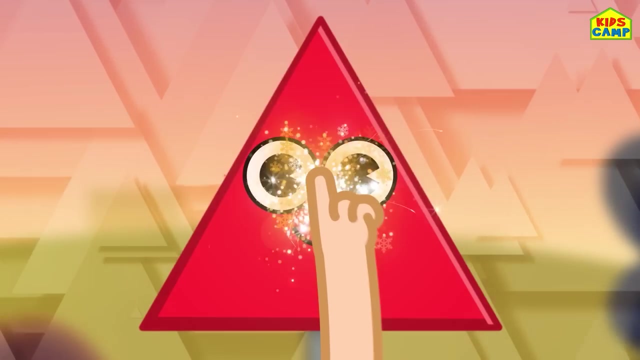 Woo-hoo Over the bridge, Here I go. Honk, honk, honk, Here I go. Oh, we almost missed that. Hmm, Is that a triangle? Yes, it is. Wow, Let's place it on my wooden truck. 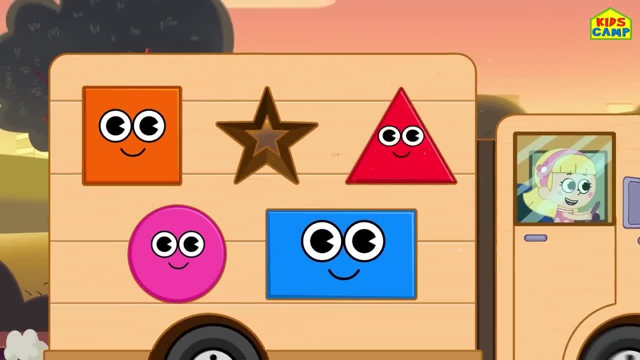 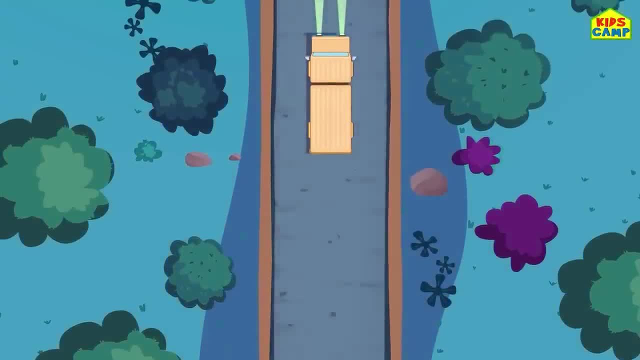 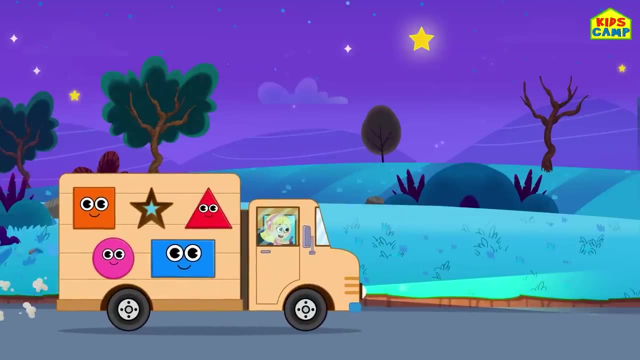 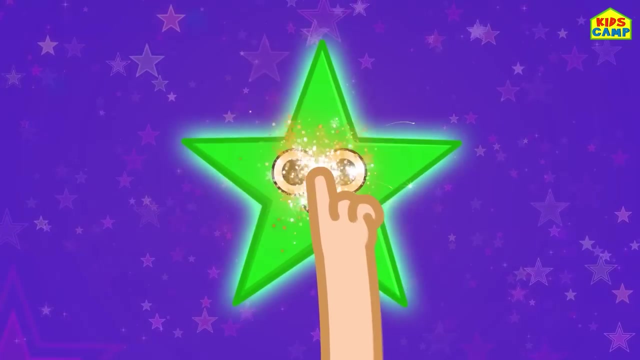 No, Uh-huh, It fits. Let's look for another shape. Where could it be? Wow, I see it, It's a star. Let's place it on my wooden truck. Oh, I see it, It's a star. 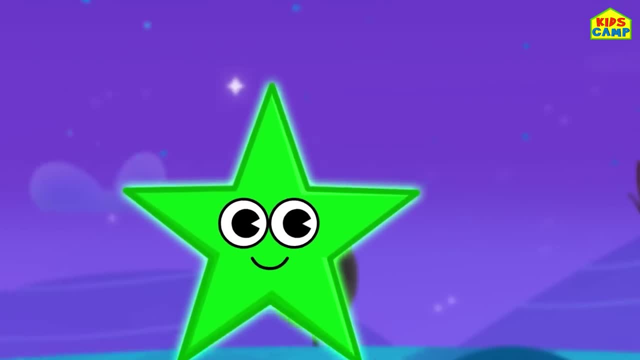 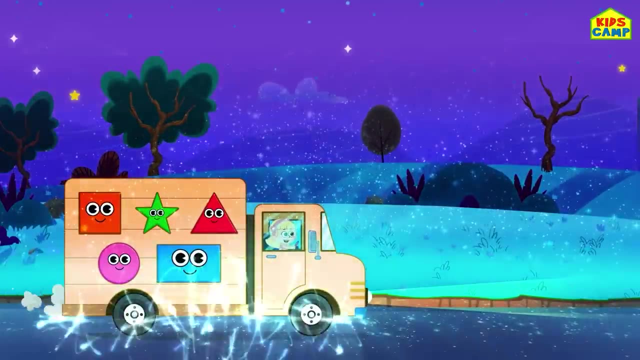 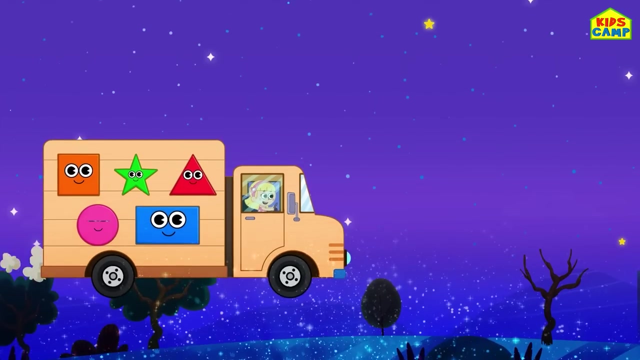 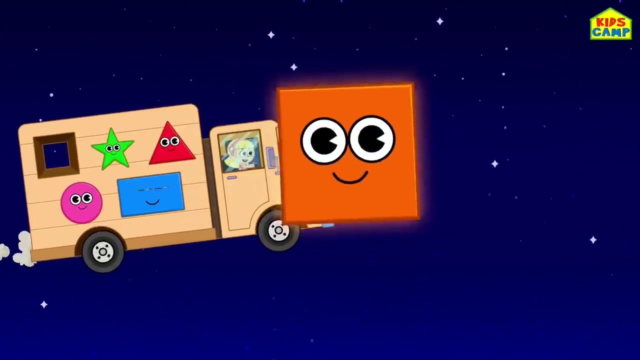 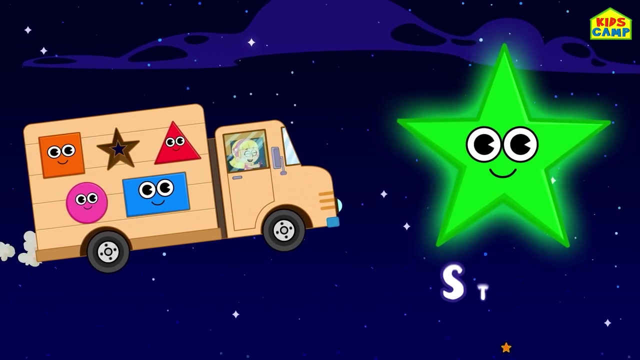 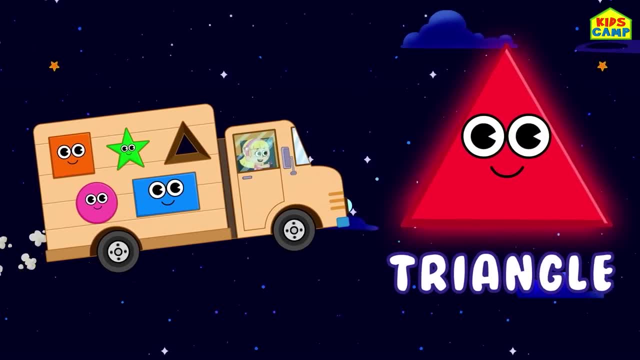 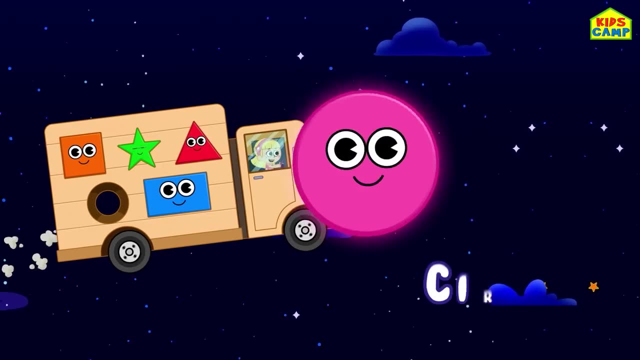 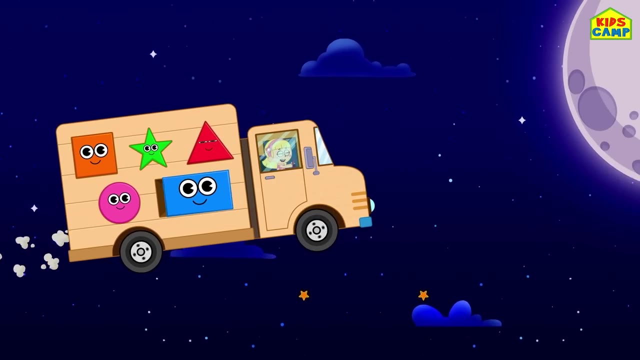 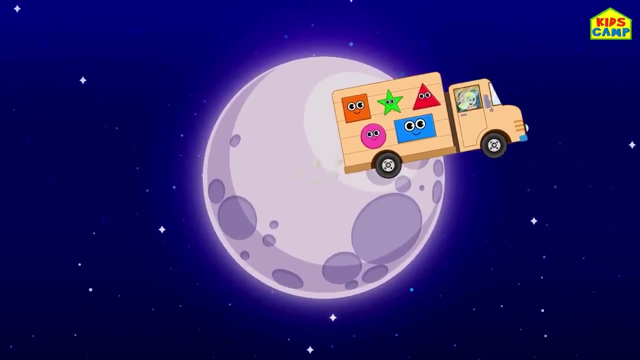 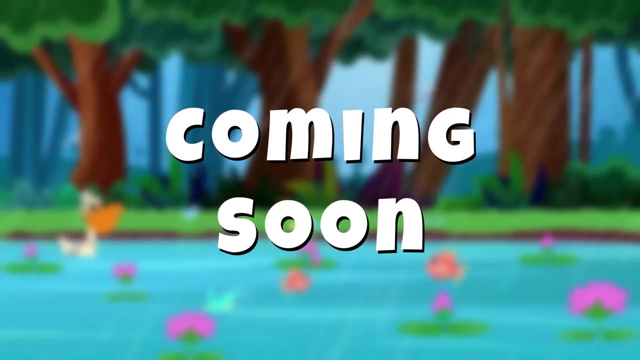 Here I go, Here I go, Here I go. Triangle Circle Rectangle- Here I go, Here I go. Let's place this here. Wonderful Over the moon, here I go. Coming soon is Baarish Aai by Choti Aur Bari. 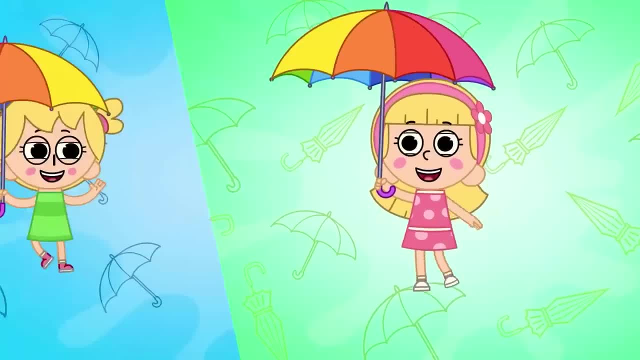 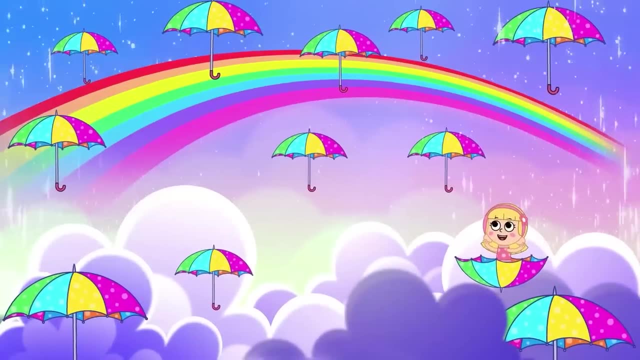 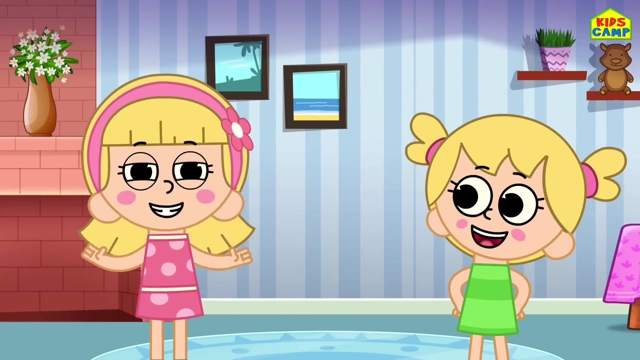 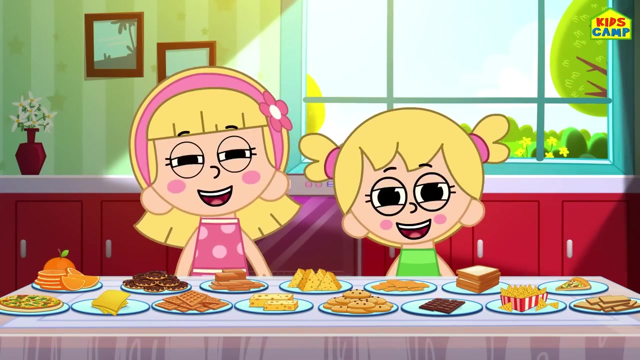 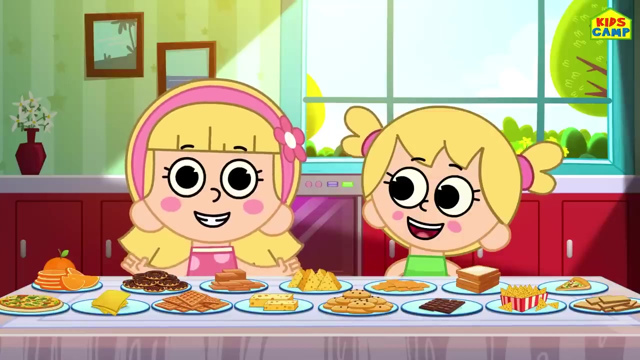 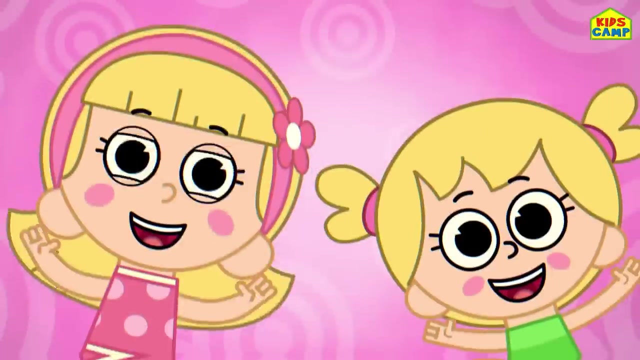 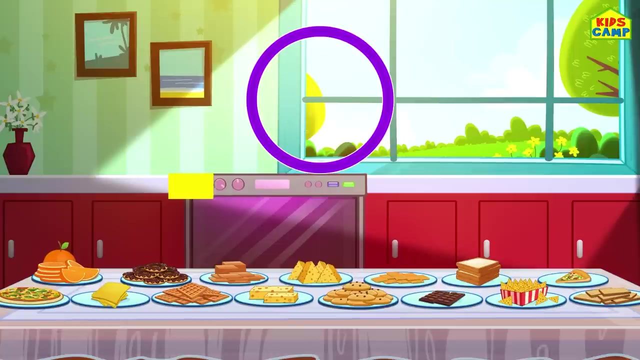 Baarish aai. baarish aai. chhum, chhum, chhum, Lekar, chhata saath nikle, hum, hum, hum. Coming soon is Baarish Aai by Choti Aur Bari With the food Circle. Can you find a circle? 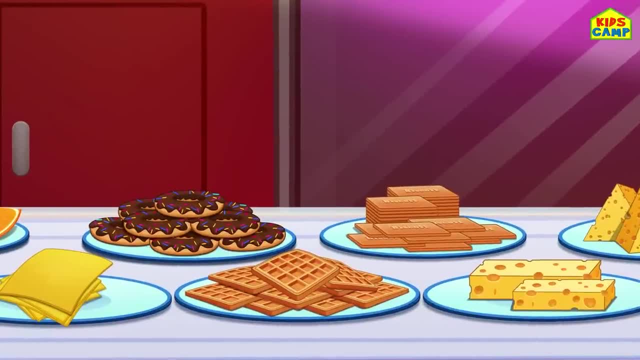 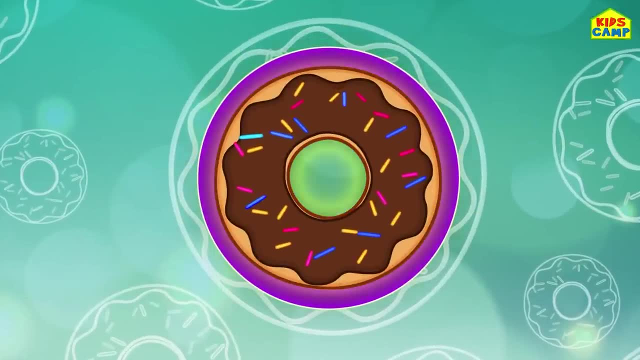 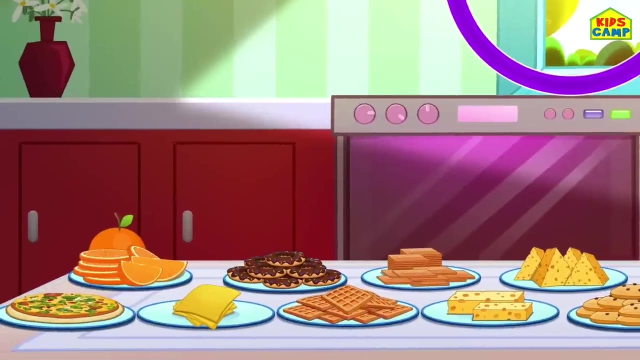 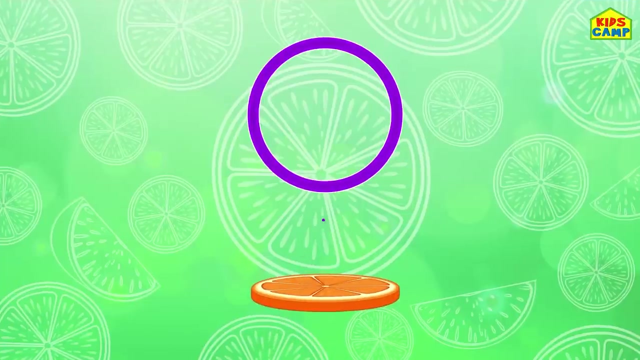 Where's a circle? What food is the shape of a circle? That's right, A doughnut. A doughnut is in the shape of a circle. What else? Hmmmm, That's right, An orange slice. Woohoo, An orange slice is also a circle. 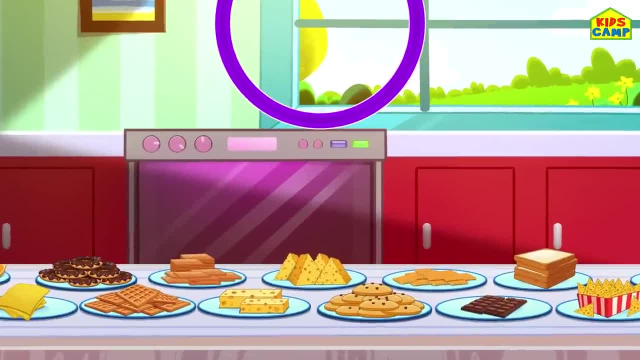 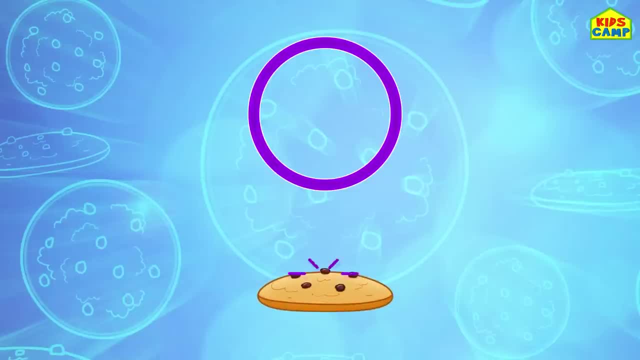 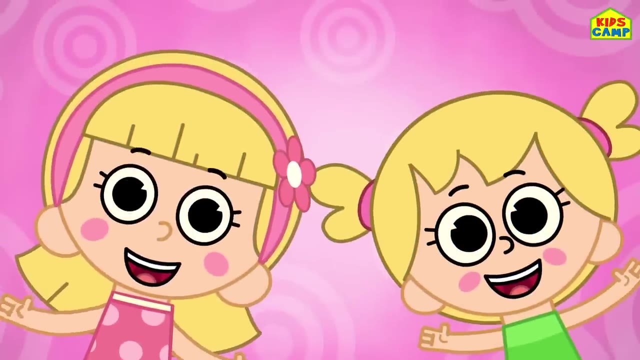 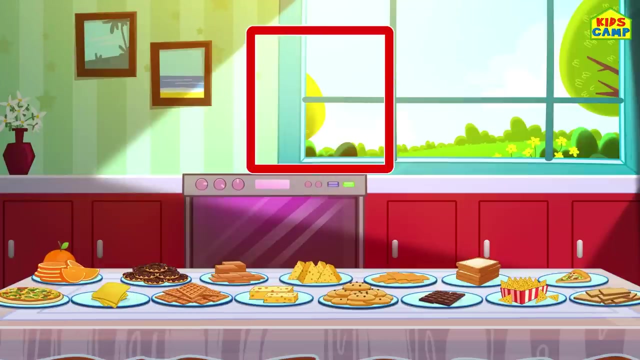 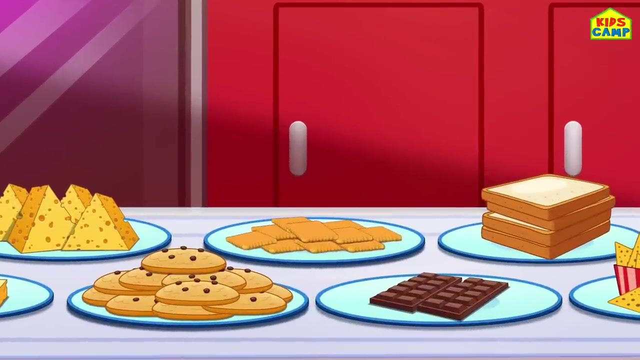 What else can we find? That's a circle? Hmmmm, A cookie. Yummy, A cookie is also a circle, Yay. What's the next shape? A square, Hmmmm, Can you find a square? kids? What food is in the shape of a square? 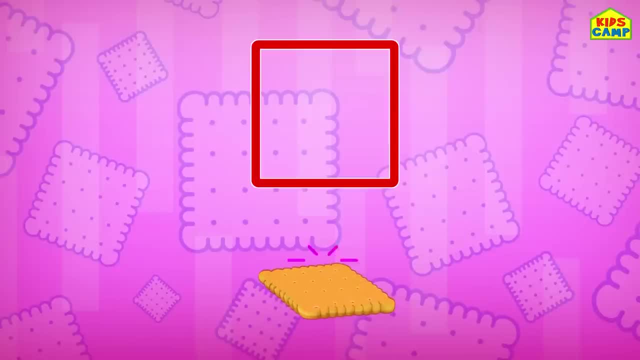 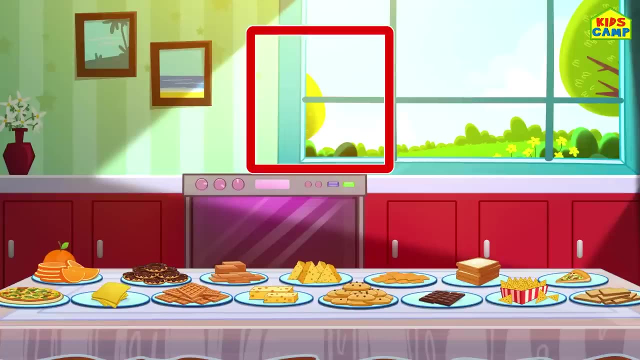 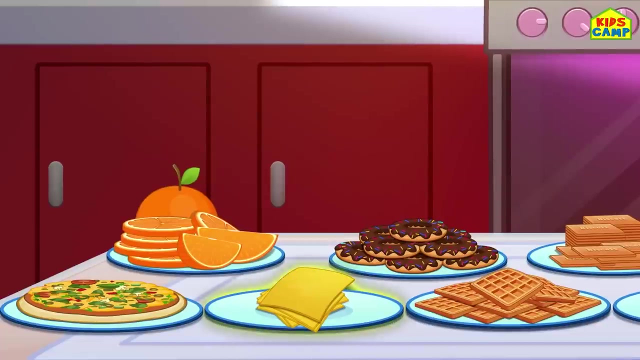 Hmmmm, That's right. A craggle, Yummy, That's the shape of a square. What else can we find? that's a square. Aha, A slice of cheese. That's right, A slice of cheese is also a square. 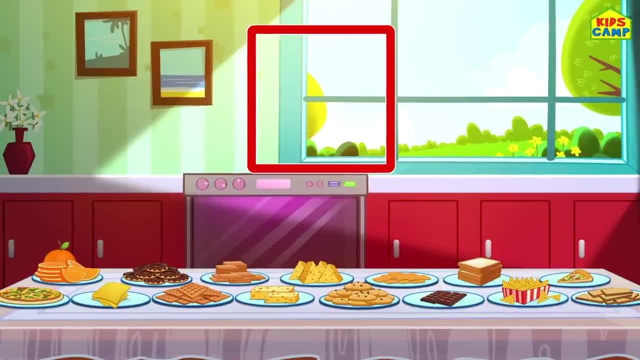 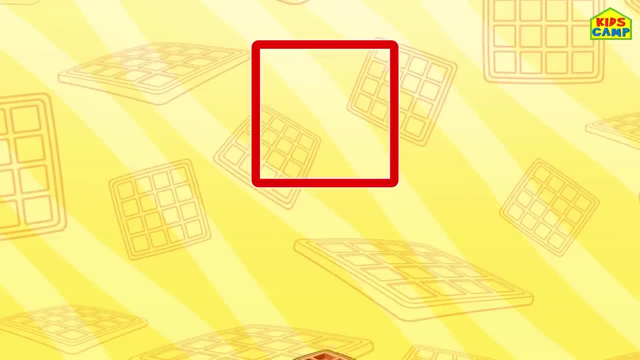 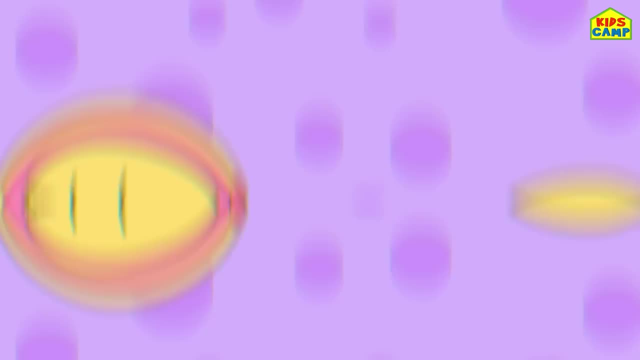 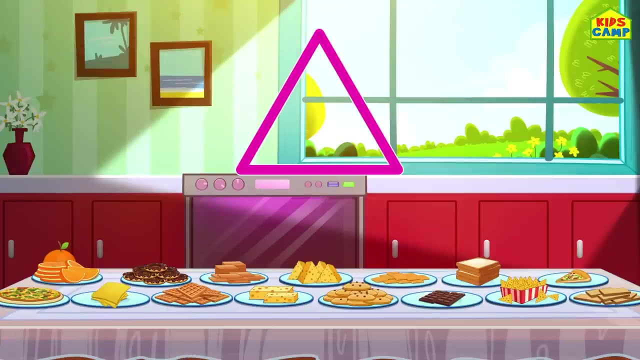 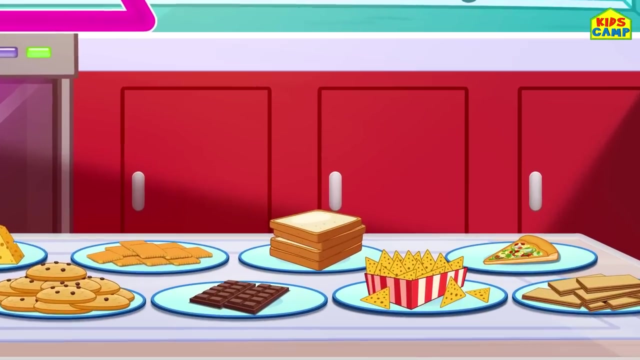 What else is a square? Aha, I see it: A waffle. A waffle is in the shape of a square. Yay, What's the next shape? A triangle. Can you find a triangle? Hmmmm, Do you see it? 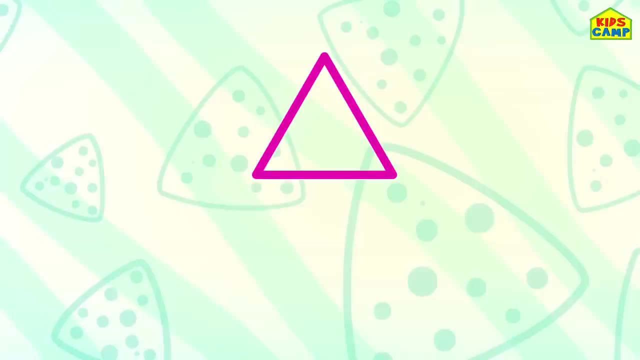 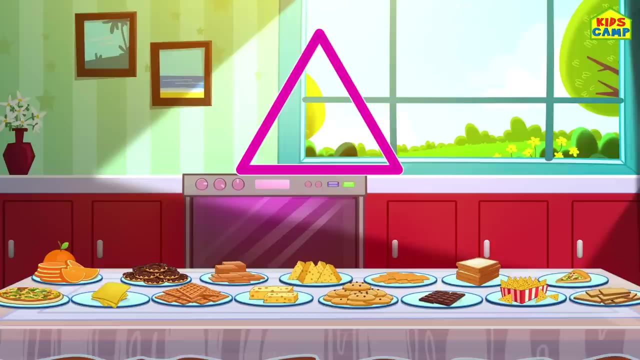 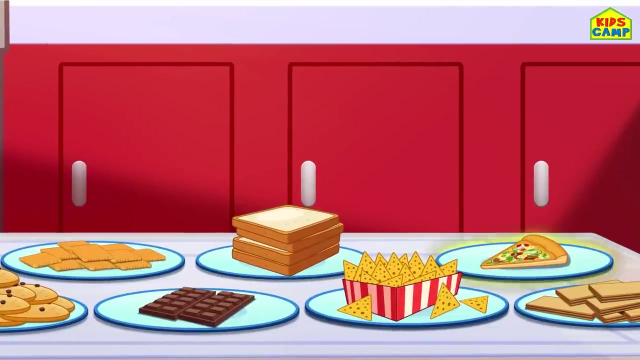 I see it too. Nachos- Yay, A nacho is in the shape of a triangle. What else That's right, Everyone's favourite. A slice of pizza- Yay, Woohoo, That sure is a triangle. 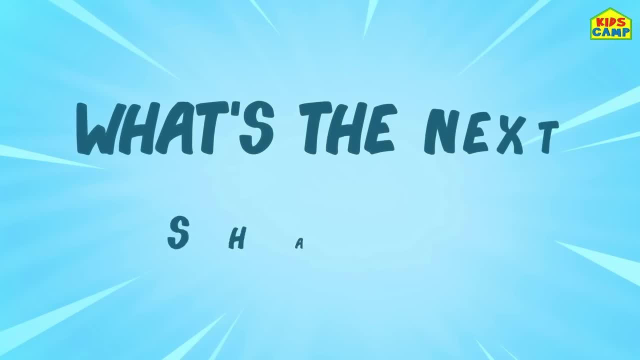 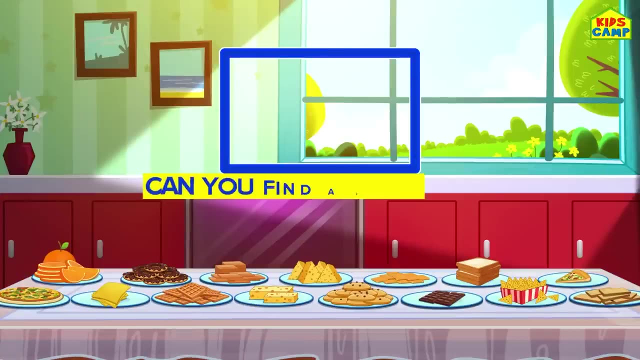 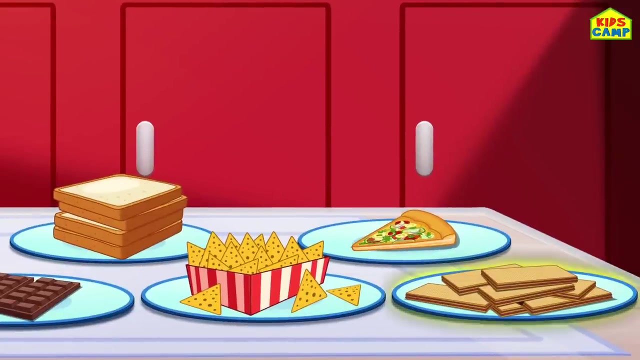 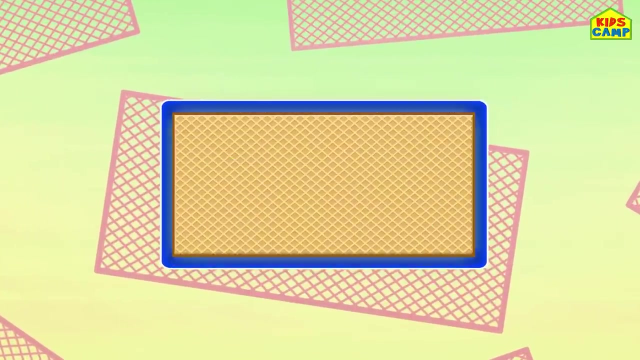 Yay, What's the next shape? A rectangle. Can you find a rectangle, kids? Hmmmm? Ah, I see it too. A chocolate wafer, That's right, That also is a rectangle. Yay, What else? Hmmmm. 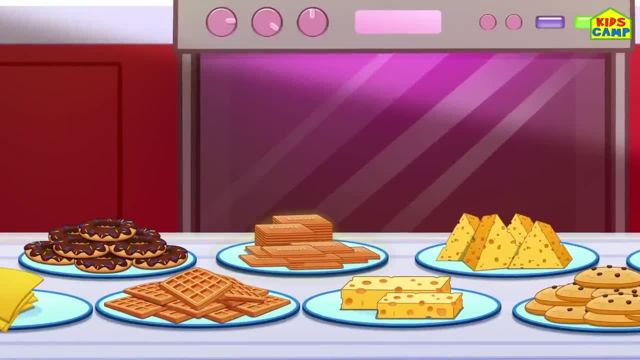 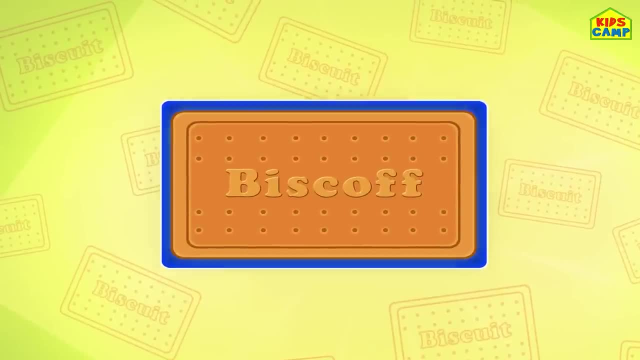 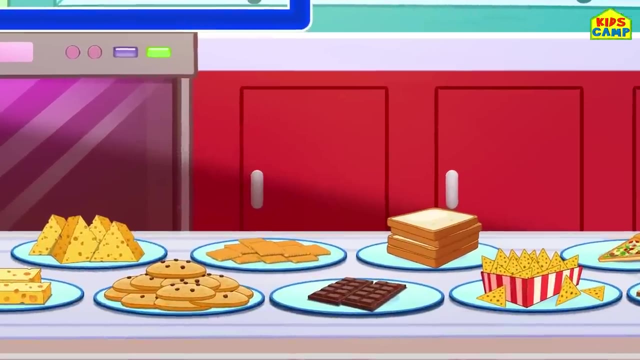 What's that? Yummy Biscuit, That sure is the shape of a rectangle. Anything else? Uh-huh Chocolate, Woohoo, A bar of chocolate. That's right, kids, We did it. This all looks so good. 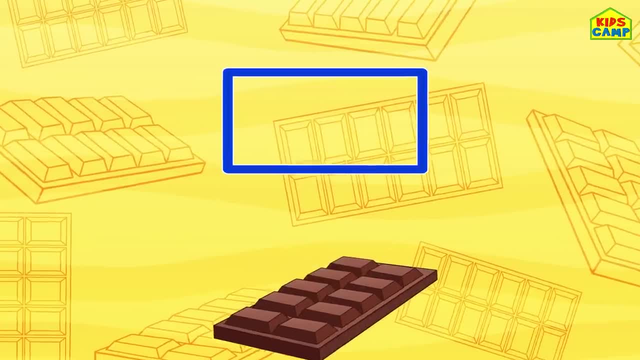 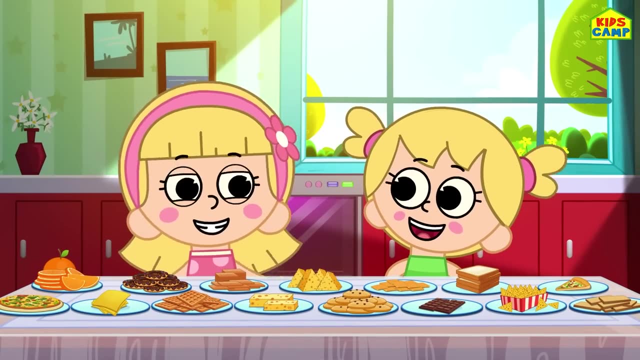 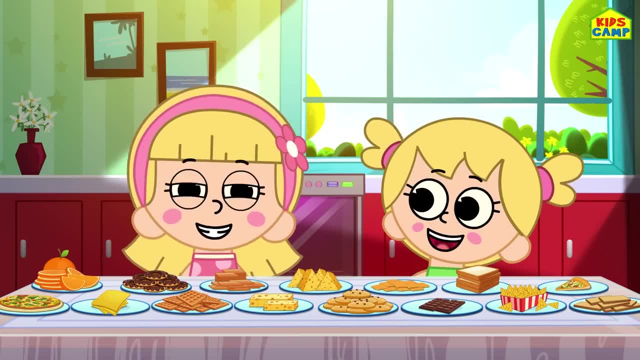 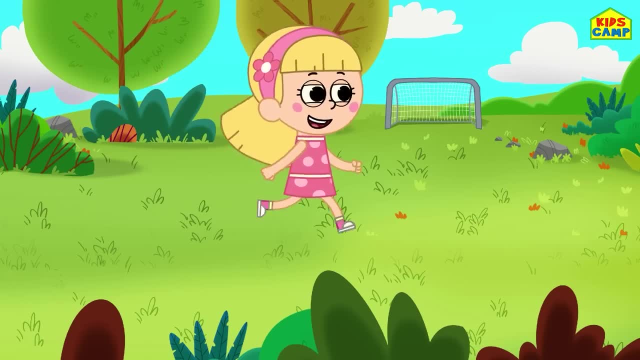 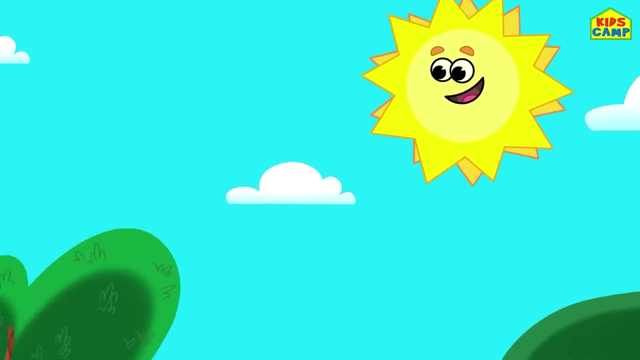 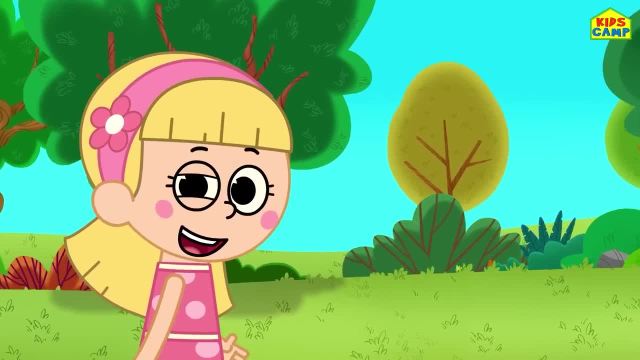 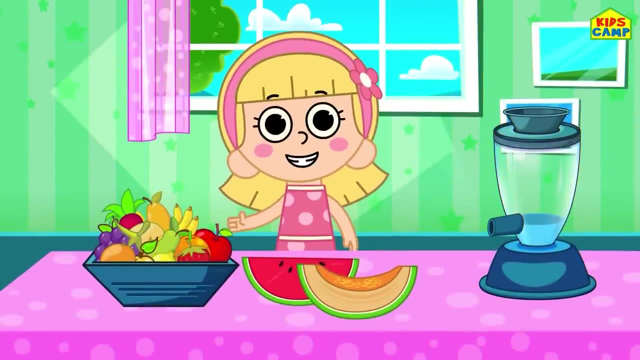 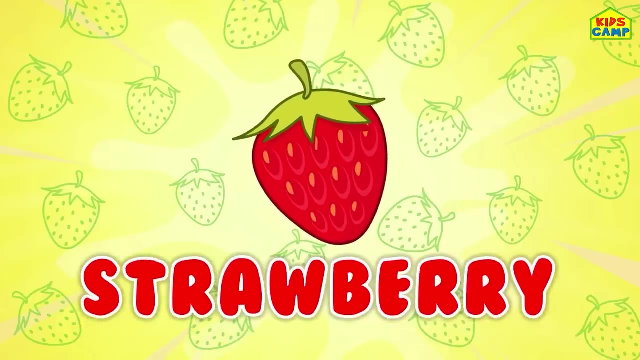 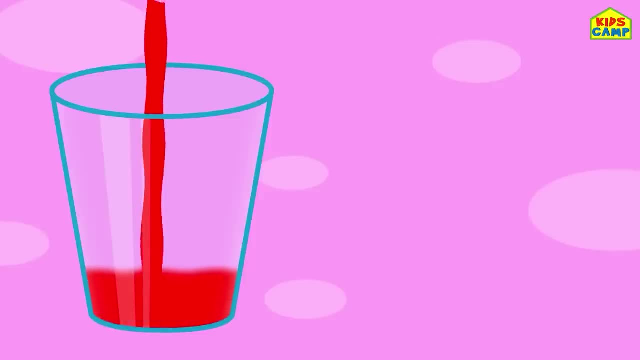 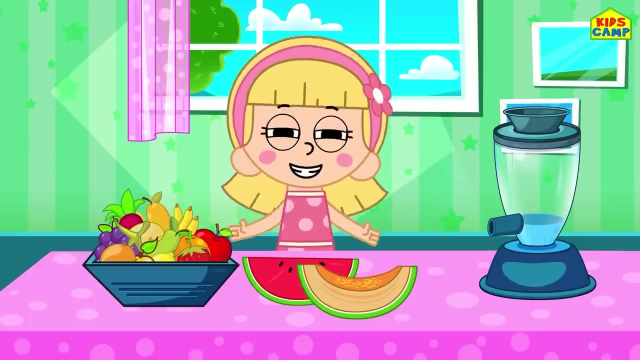 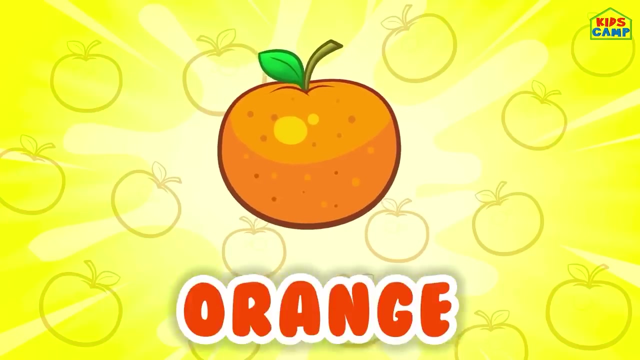 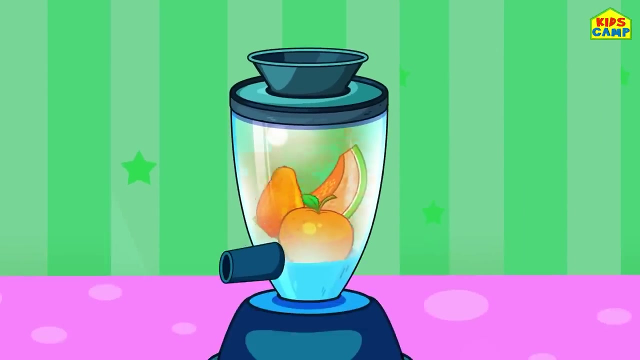 Yay, A red cooler. Let us give them another go. I'm going to take A yummy papaya, An orange And a juicy melon. In they go. Let's mix them up. Woohoo, An orange cooler. 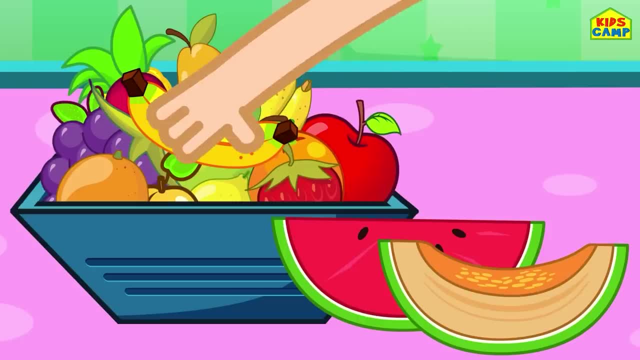 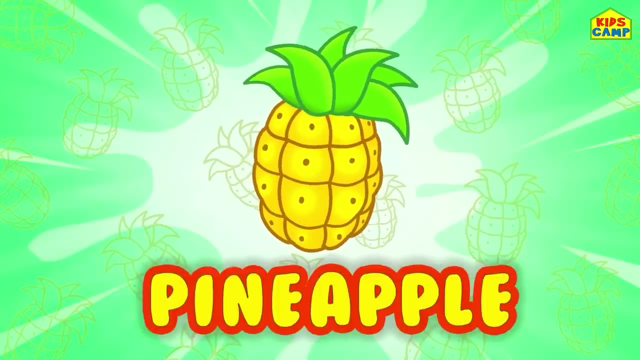 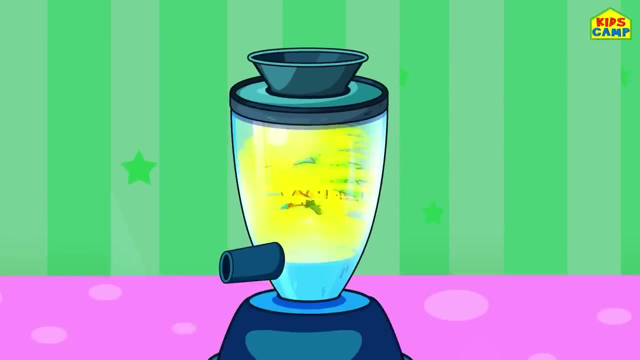 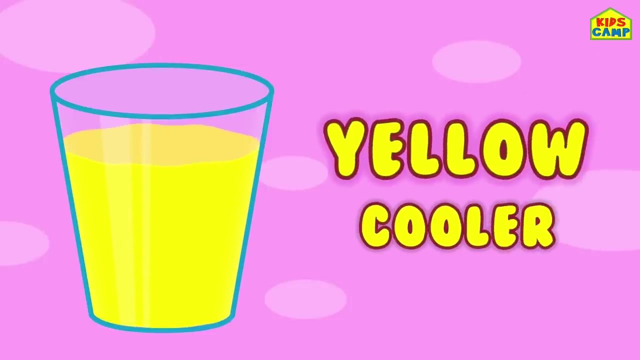 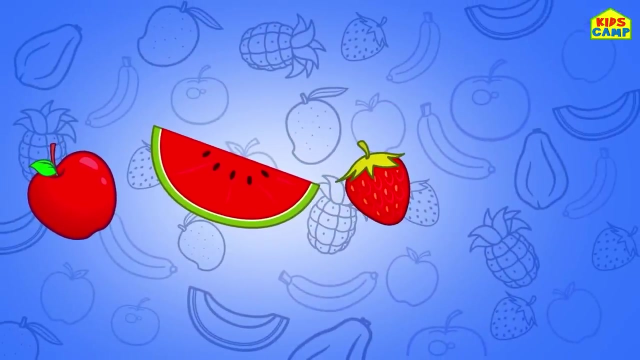 Let's try another one. This time I'm going to take a banana And a pineapple And a yummy mango. Woohoo, In they go, Let's mix them up. A yellow cooler. Wow, Today we learned that apples, watermelons and strawberries are red. 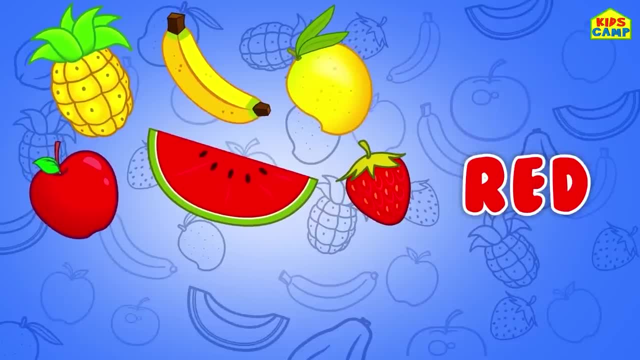 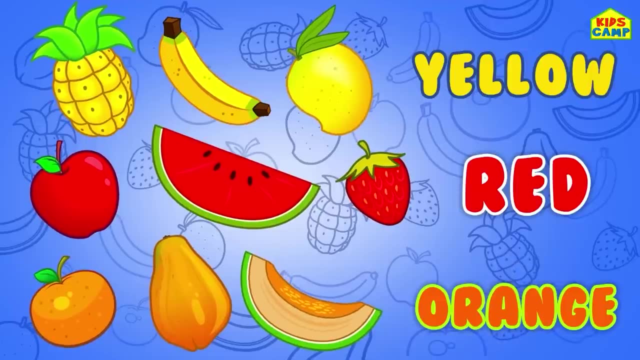 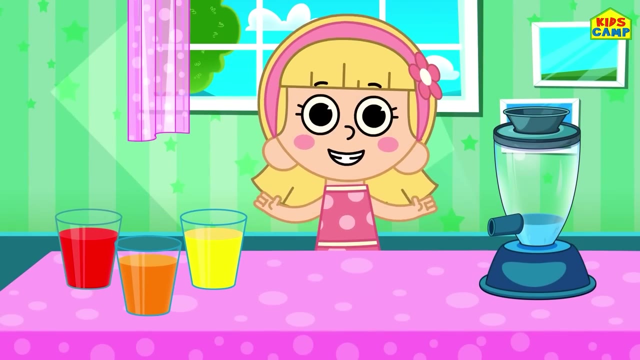 Mangoes, bananas and pineapples are yellow Oranges, papayas and melons are orange in color. We had a fun learning day And delicious. We only had two days to go. We also had a wonderful training session. 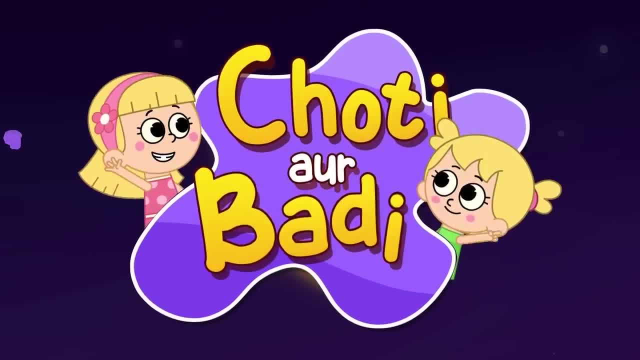 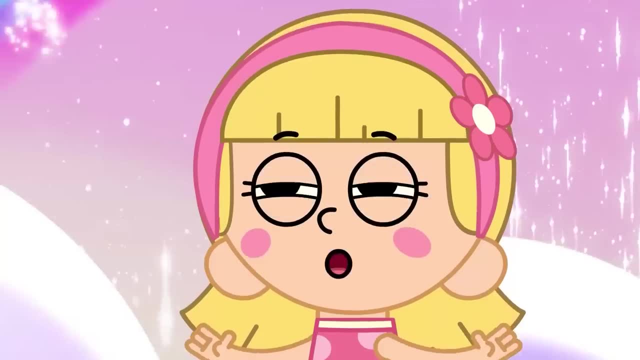 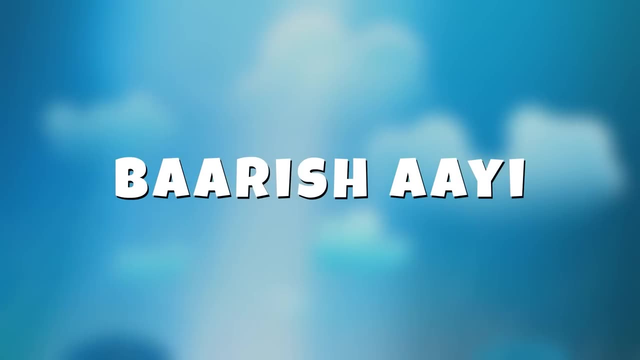 So much fun today, So sleep well, Come home and have a nice day. Bye Rules. Hi, We are all familiar with A delicious Anda c Fusion sweet. I bought this here at experiment, And the cool one I bought for you is: 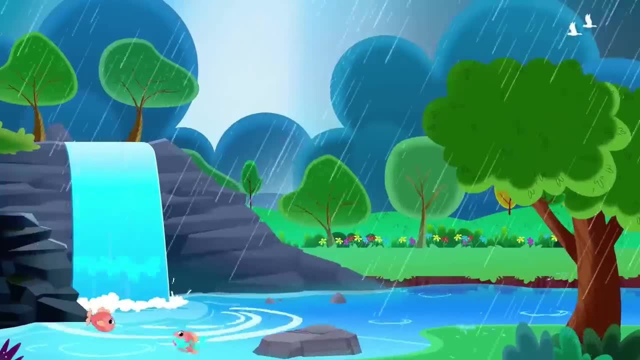 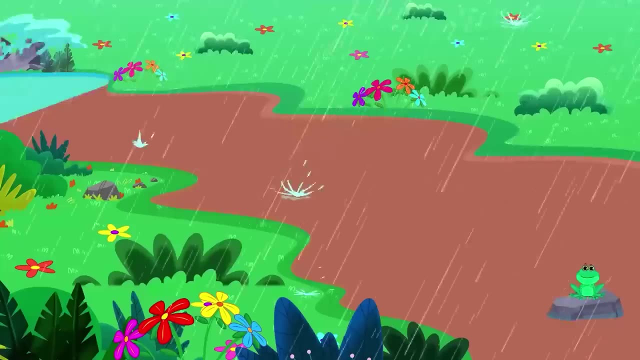 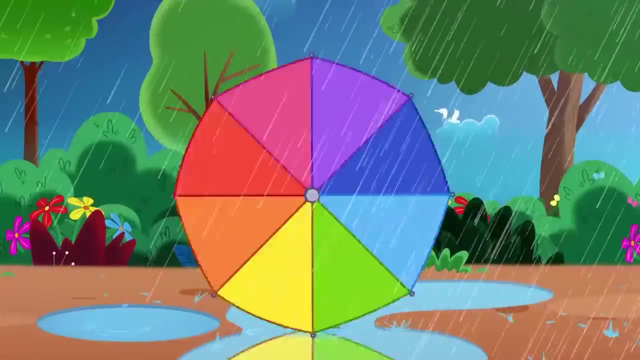 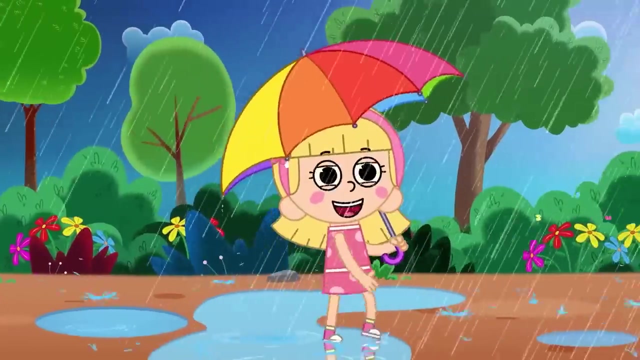 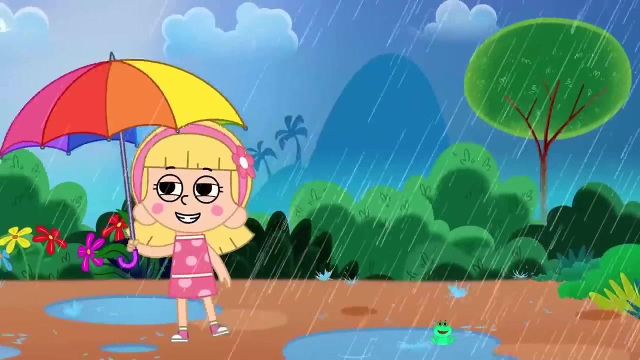 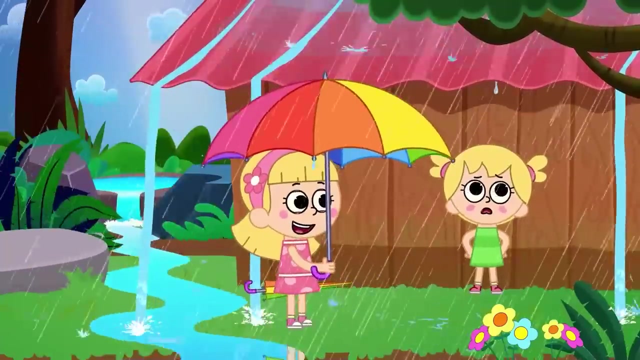 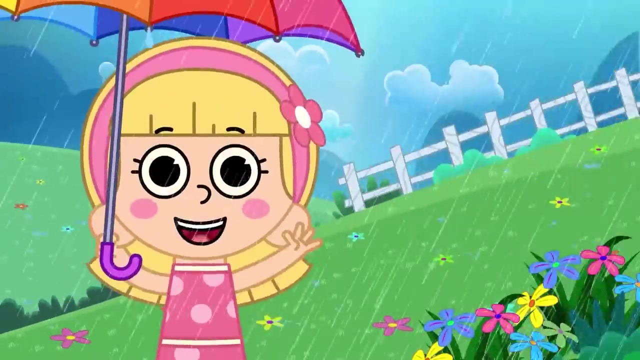 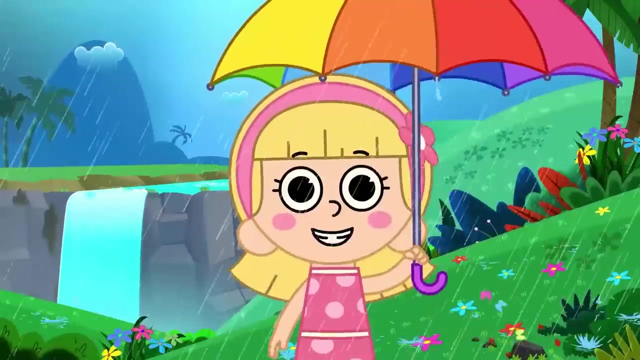 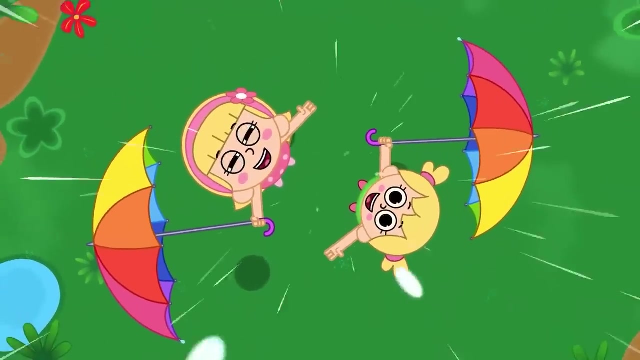 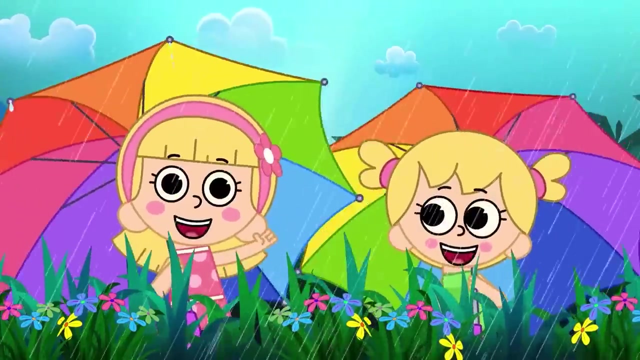 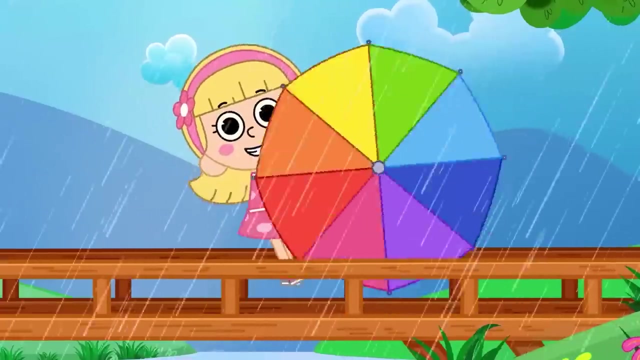 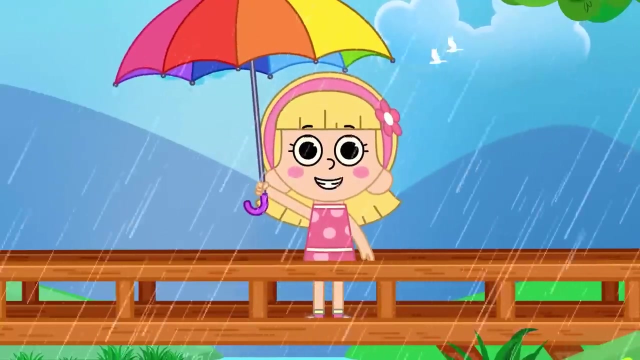 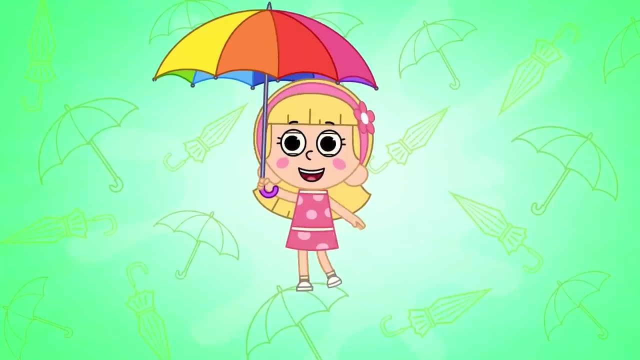 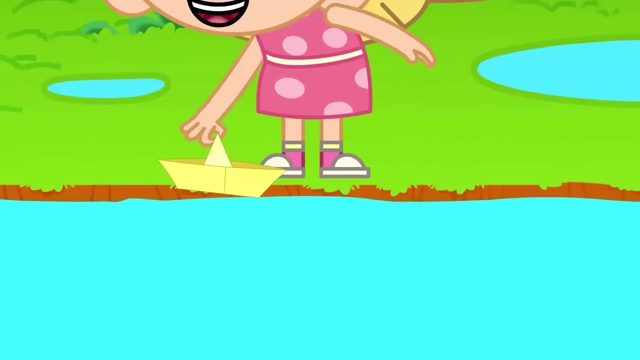 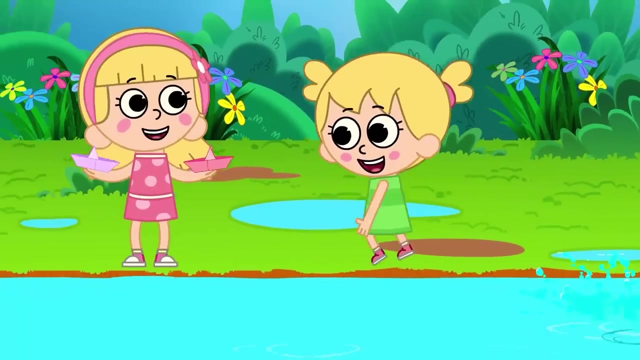 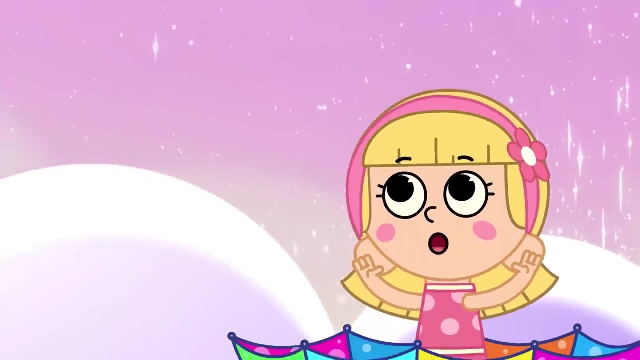 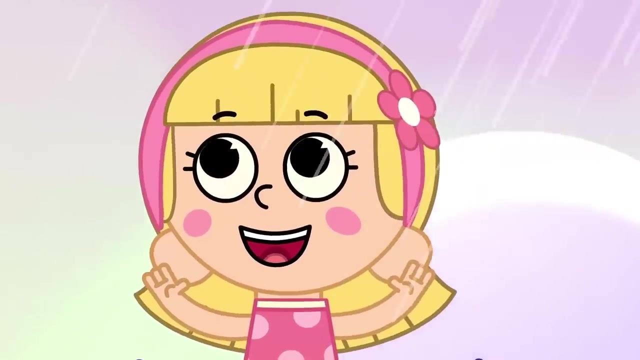 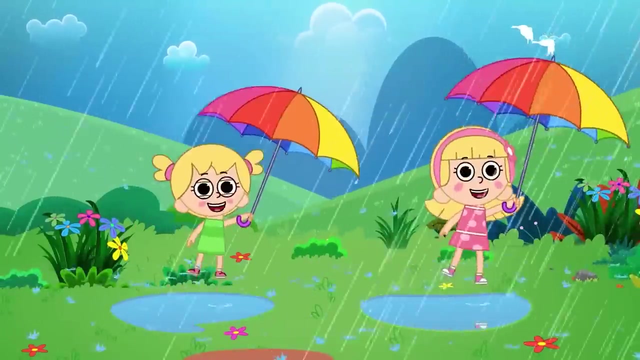 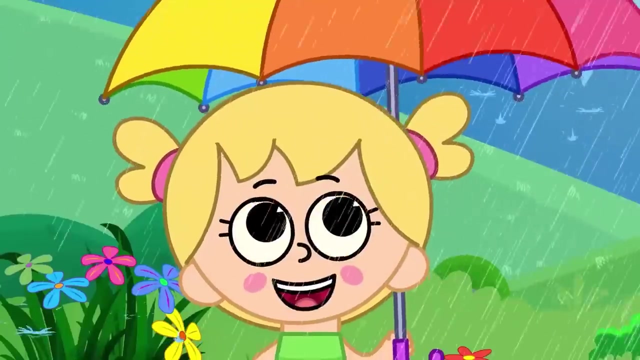 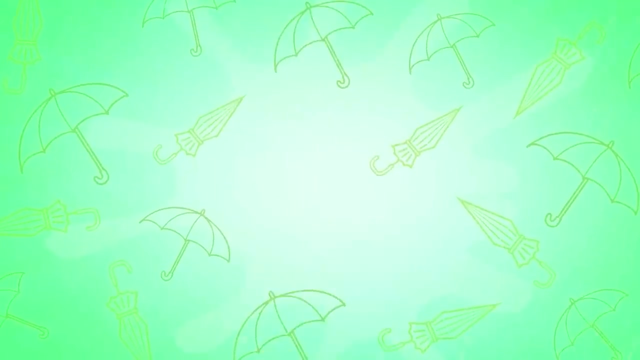 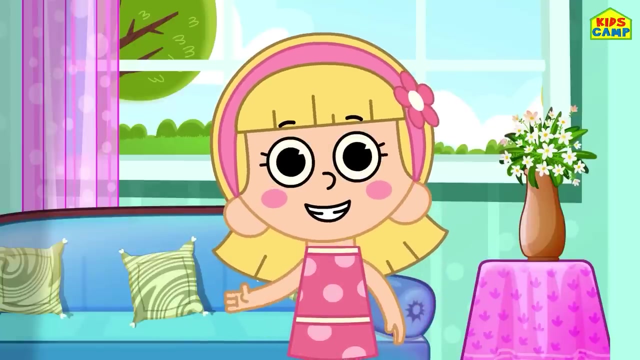 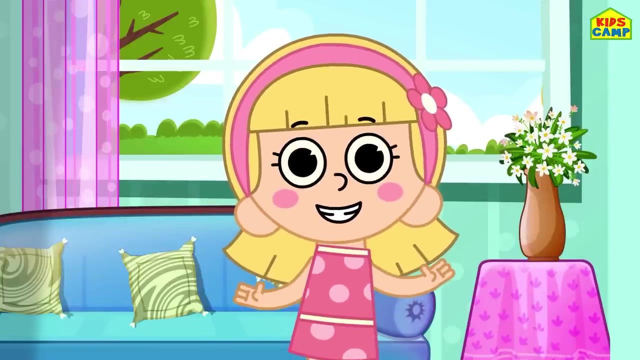 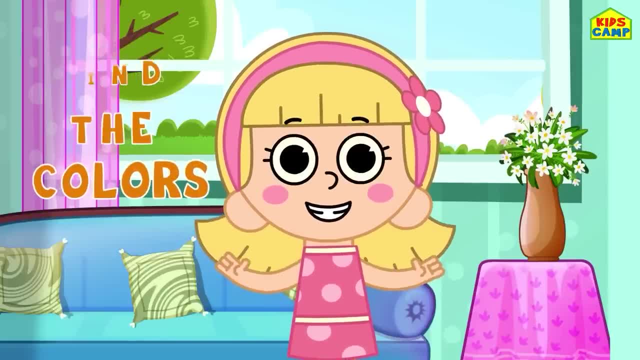 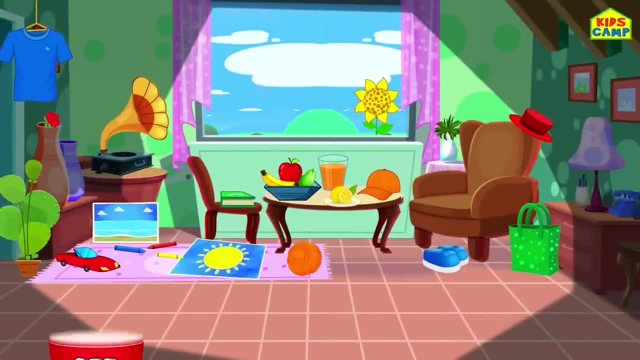 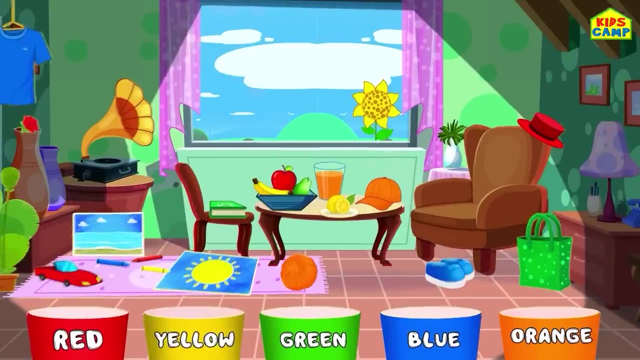 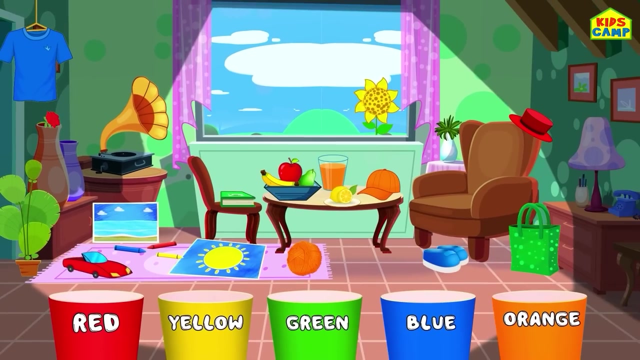 The first color that we have to find is red. Can you spot everything red? Let's get started. Can you find anything red? That's right, a toy car. Yes, it's red. Let's add it to the red bucket. 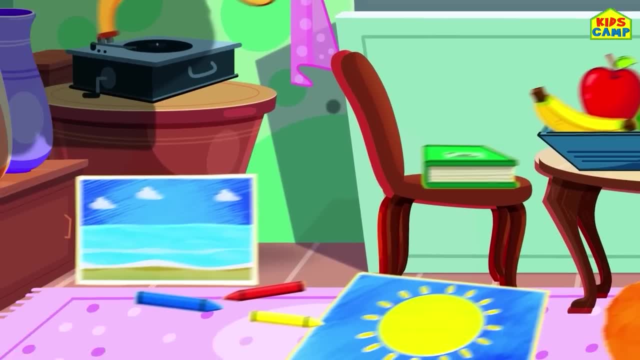 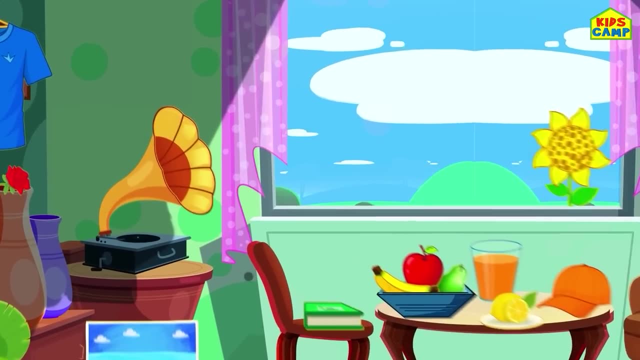 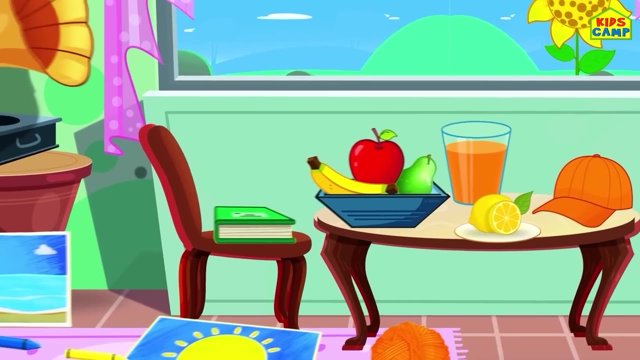 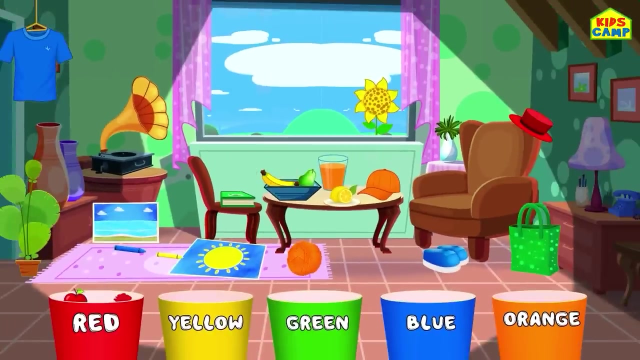 What next? What else is red? Uh-huh, I see a red crayon. That's right. Wow, a red rose. What else is red? An apple. We'll add that to our red bucket. Keep looking for something else that's red. 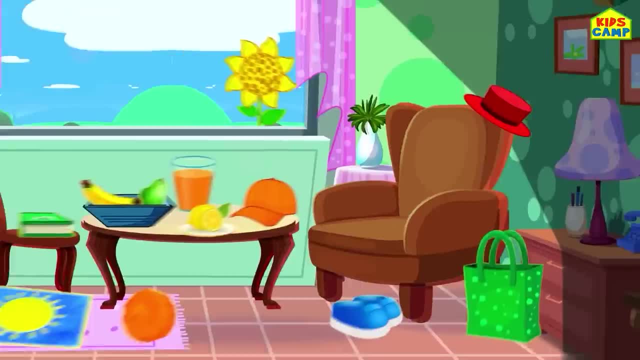 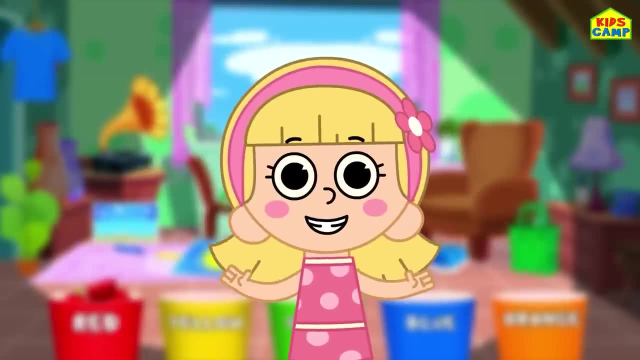 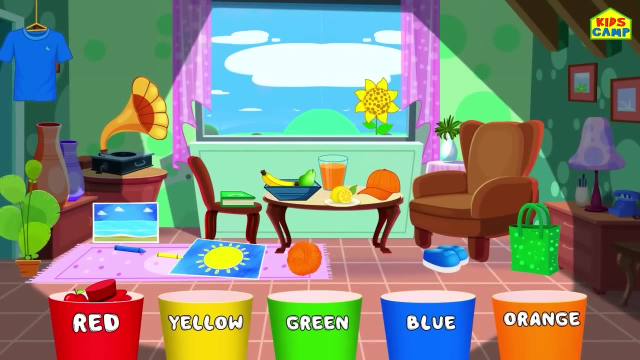 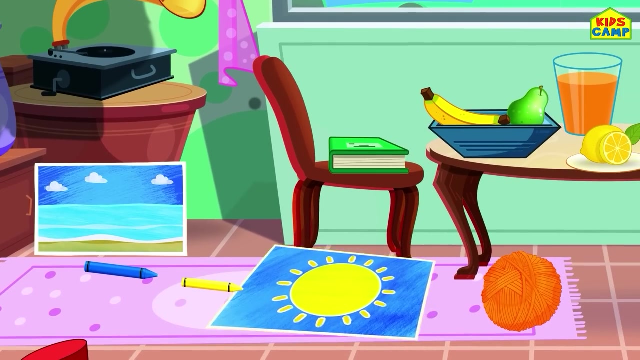 That's right, a red hat. Woo-hoo, We found everything that was red. What's the next color? Yellow, My favorite. What do you see? that's yellow. Uh-huh, my drawing of the sun, The sunflower. 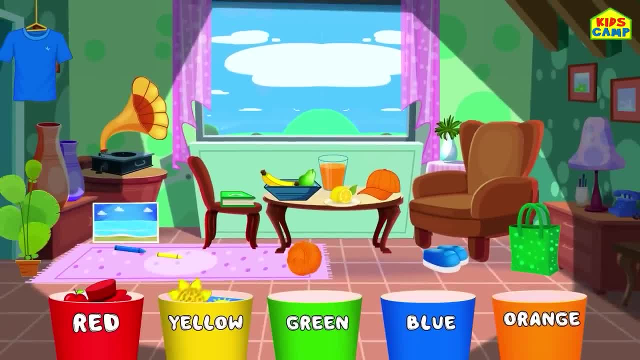 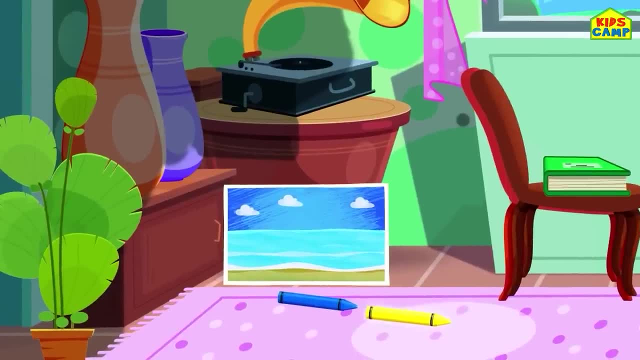 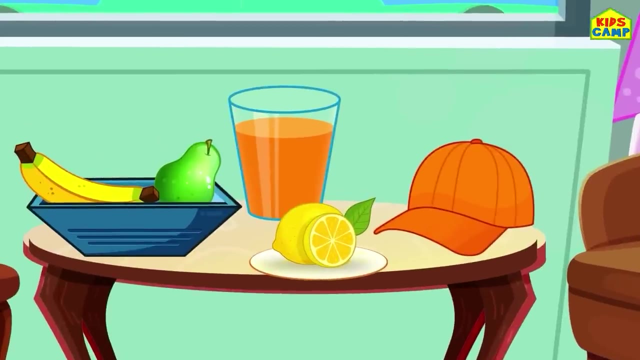 That's yellow too. Into the bucket, Into the bucket. Good job, friends. What else is yellow? A yellow crayon, That's right. What else do you see? Uh-huh lemons, Wonderful. What else? Uh-huh, a banana. 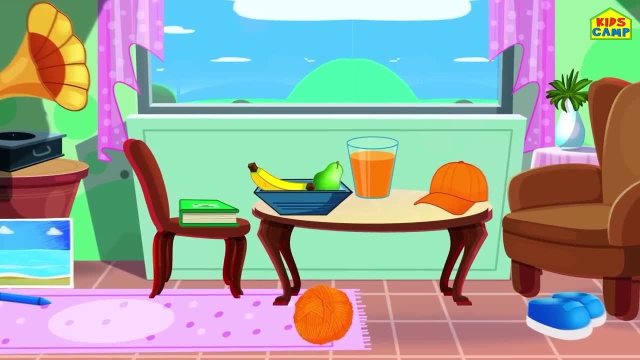 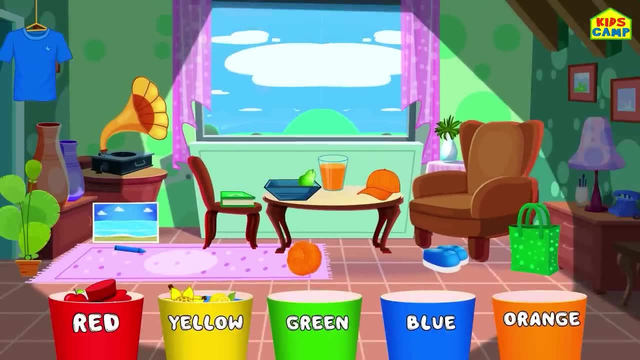 The banana is yellow. Into the yellow bucket, it goes. Let's add some more yellow. Uh-huh a banana. The banana is yellow. Into the yellow bucket, it goes. Let's go to the next color, which is green. Can you look for something that is green in my room? 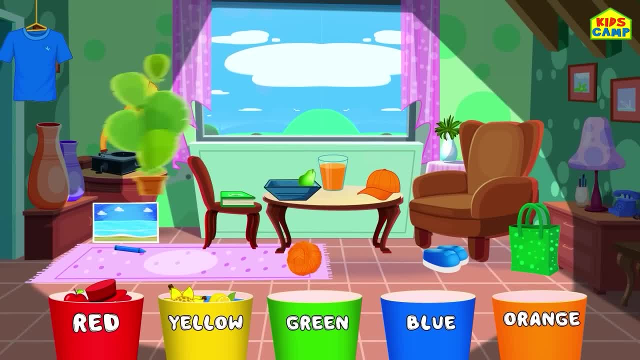 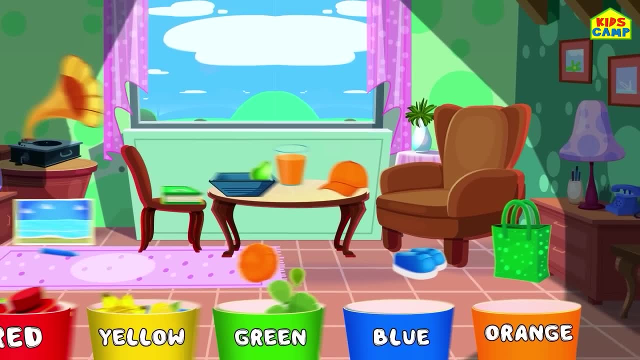 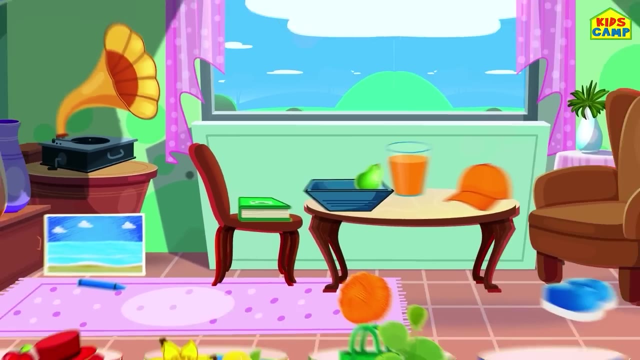 Uh-huh, I see it. The plant Into the bucket, it goes. What else is green? That's right, the green bag. Anything else? I see it too. the green book, Woo-hoo, What else? The pear? 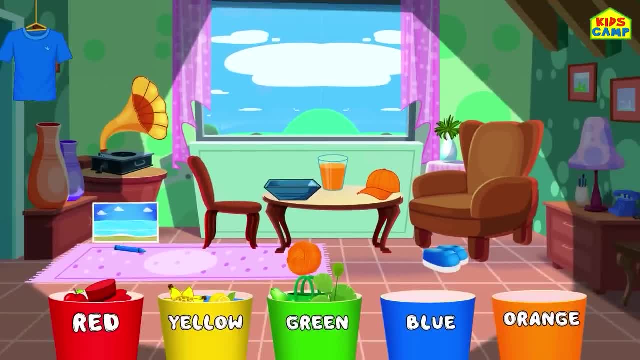 That's green too. Into the green bucket. Yay, Let's move on to the next color. It's blue. Woo-hoo. What's blue colored here? The blue crayon, Anything else. My drawing of the blue sky. 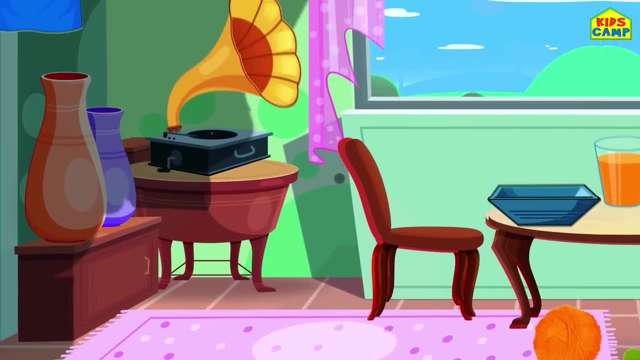 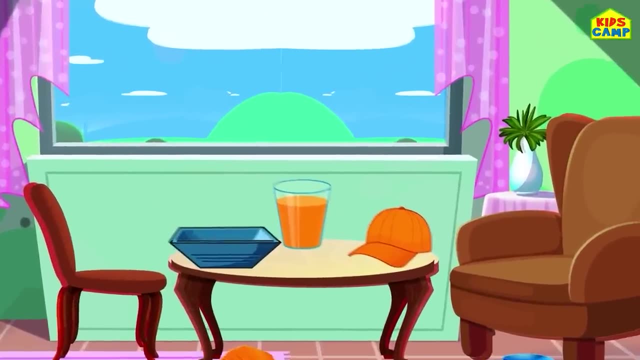 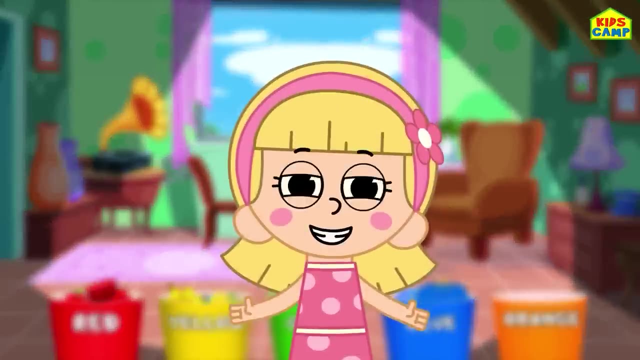 What else? The blue T-shirt Into the bucket? Uh-huh, I see My pair of blue shoes. We found everything blue. What's next? It's orange. Yay, That's right. Can you spot something orange? 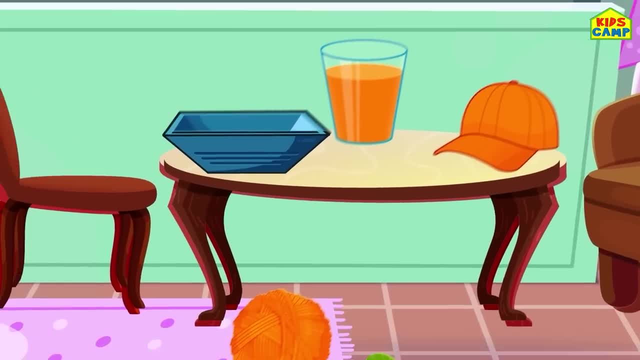 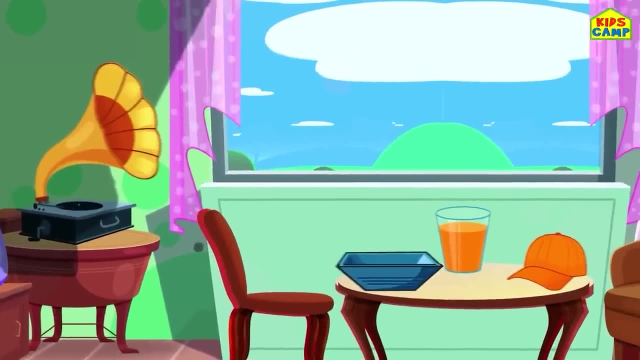 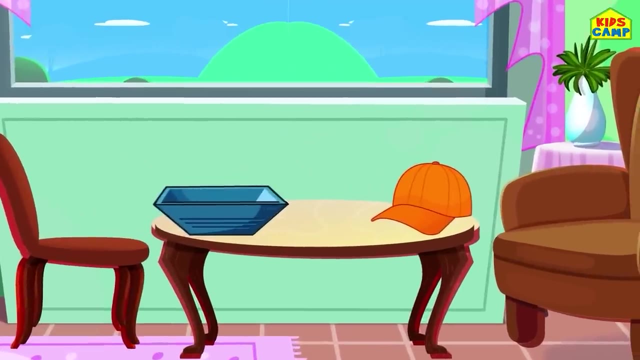 An orange yarn of wool, That's right. Can you spot something green? An orange yarn of wool, That's right. What next? I see it: A glass of orange juice And an orange cap. Yay, Into the orange bucket, it goes. 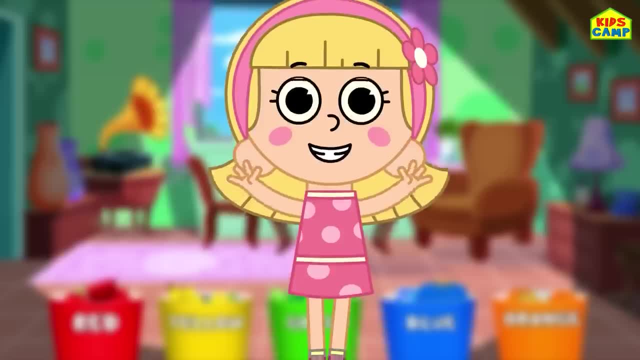 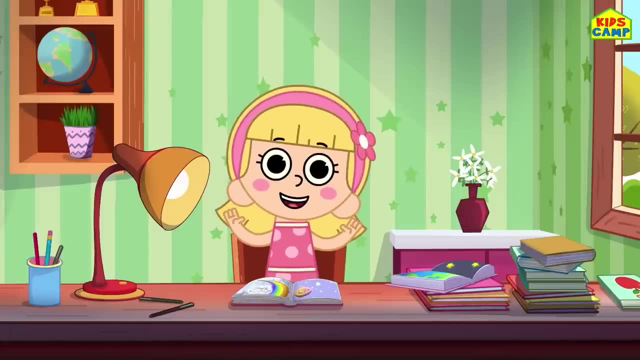 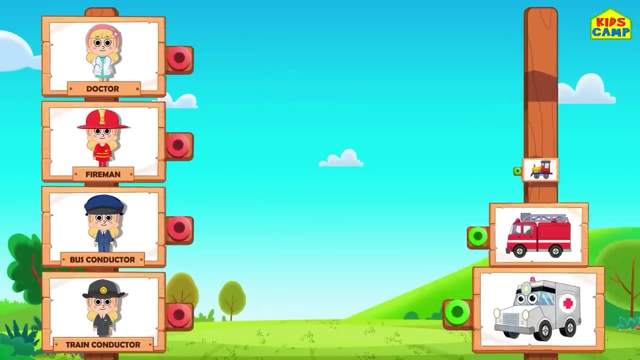 Wonderful kids. We found all the colors. Bye, Hi friends. I'm Ellie. This is a fun game where we match the pairs. Let's match the professions to their vehicles. Let's match the professions to their vehicles. Let's match the professions to their vehicles. 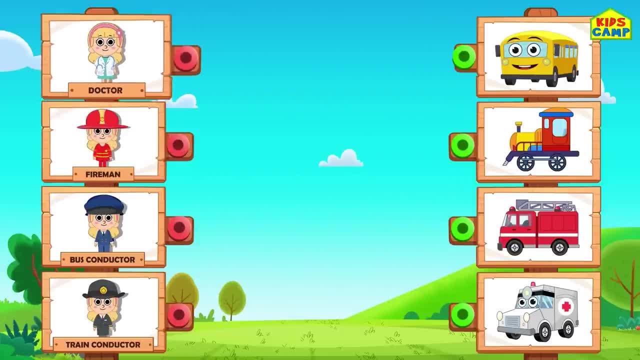 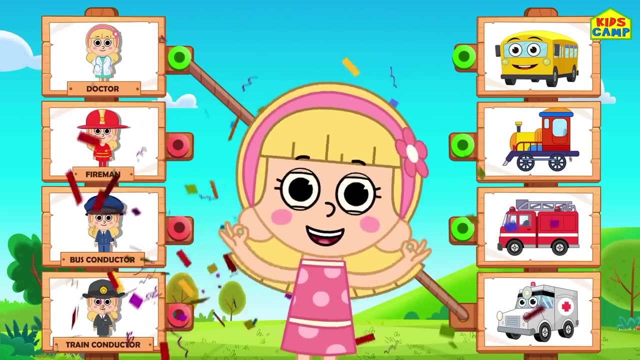 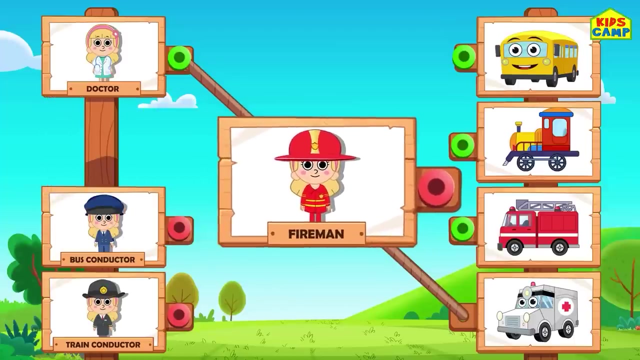 What vehicle will a doctor use? What vehicle will a doctor use? A fire truck- No. A train- No. A train- No. Hmm, I know The doctor will use an ambulance, That's right, Yay, A firefighter will use. 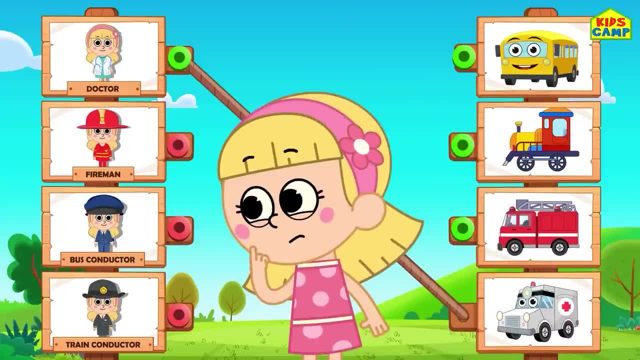 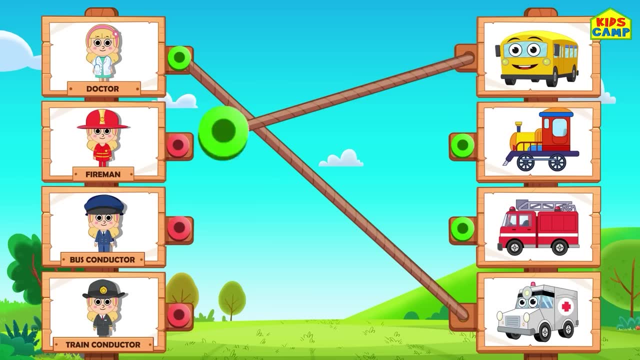 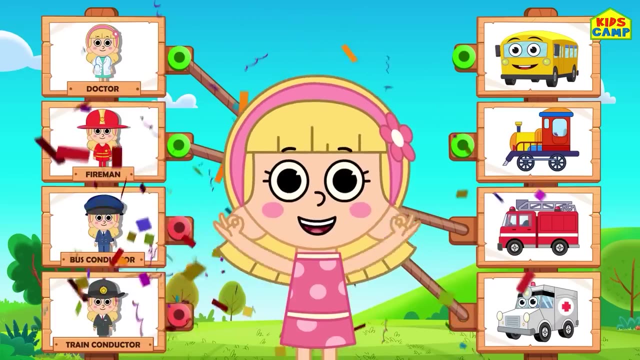 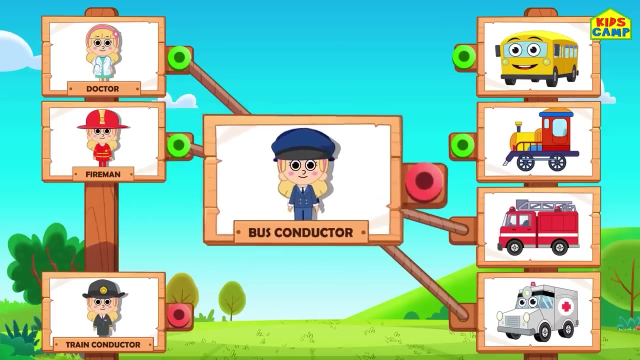 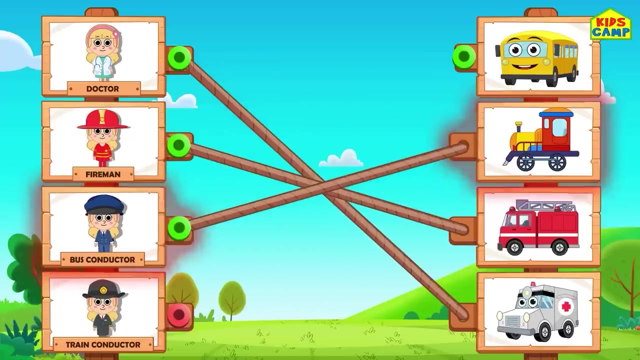 A firefighter will use Which vehicle? Which vehicle? A bus? No A fire truck- A fire truck, That's right. Yay, Come on. A bus driver will use a train- No A bus, That's right. 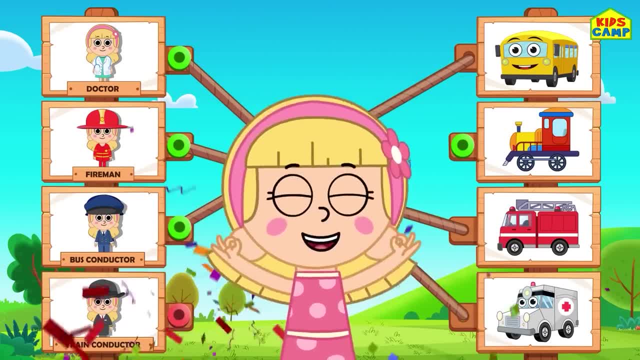 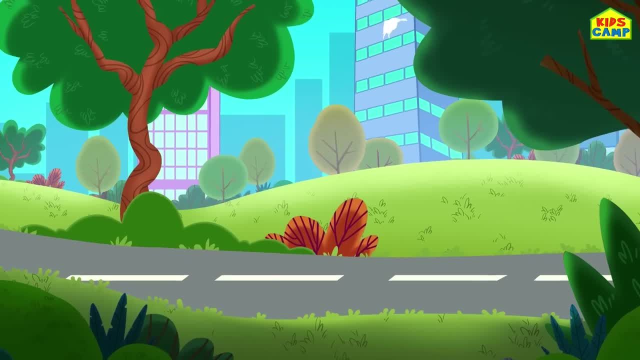 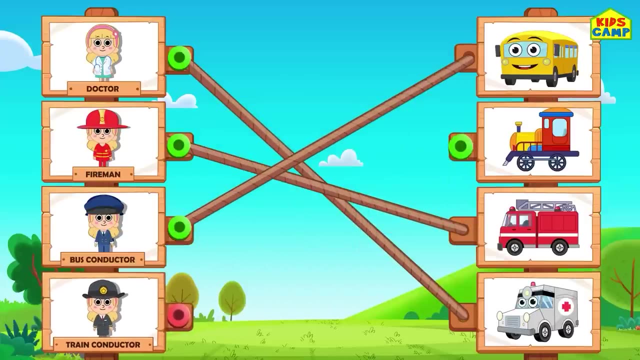 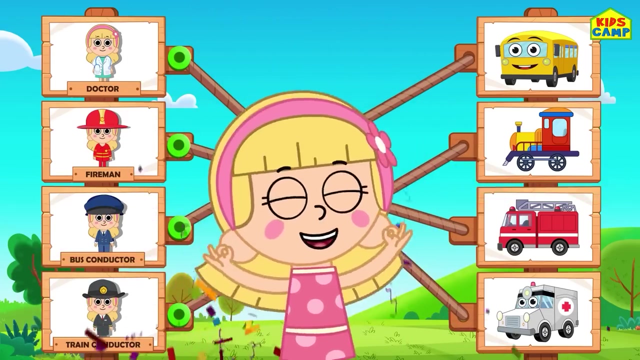 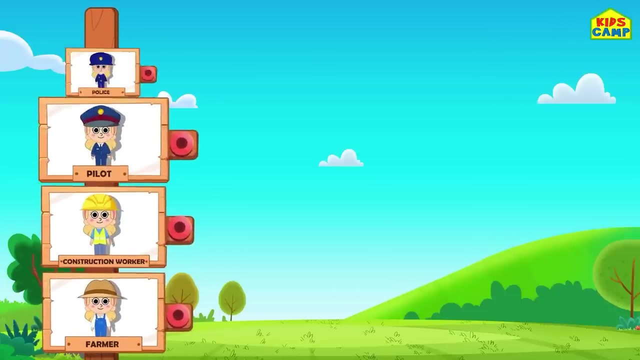 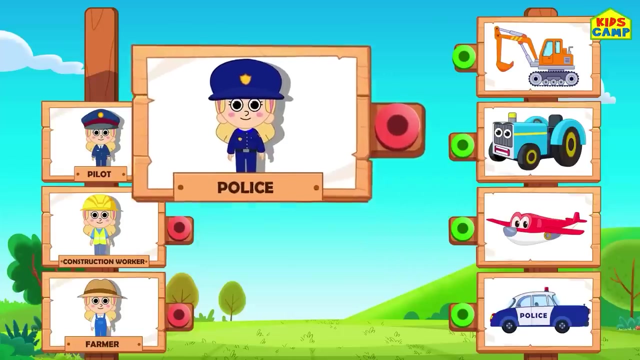 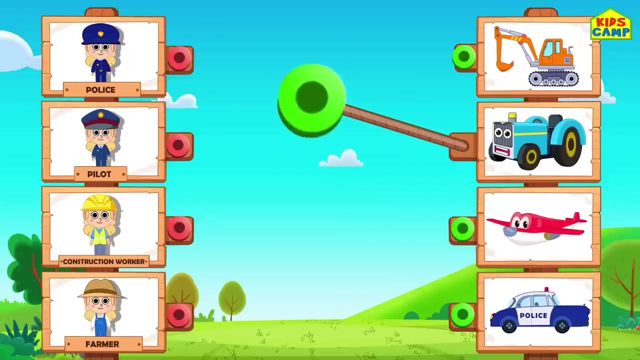 Good job, friends. Yay, What's next? A train conductor? Which vehicle will he use? The train, That's right, All aboard, All aboard. Ooh, Which vehicle will the police use? An airplane, No, A tractor. 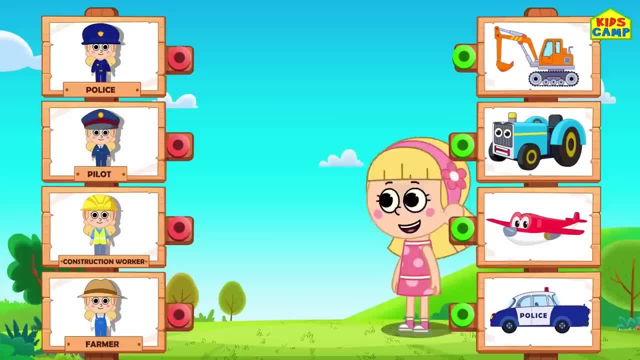 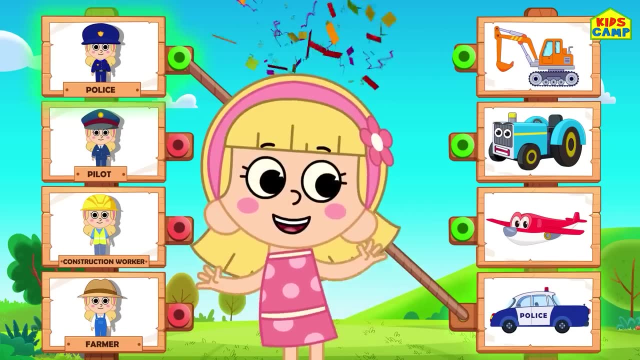 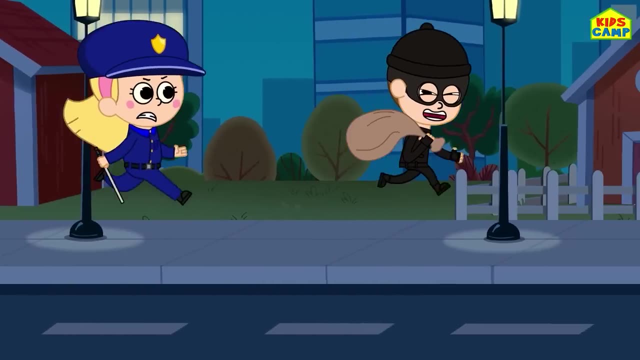 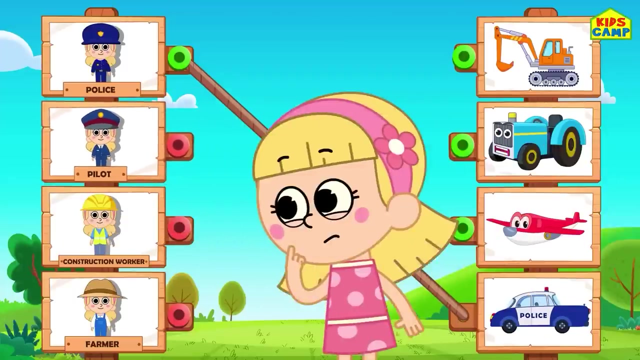 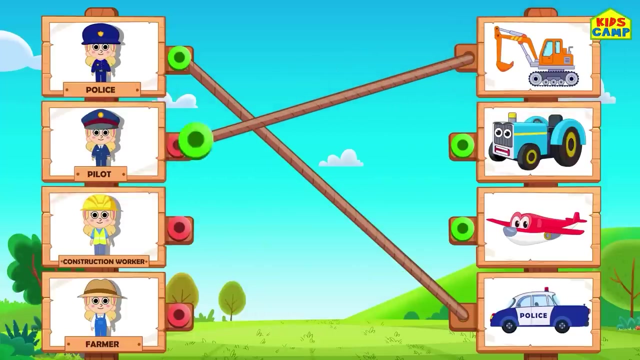 No way. Hmm, I know A police car, That's right. Yay, A pilot will use Which vehicle? Hmm, A train, A digger? No, An airplane? Yes, Fly away. Yay, A construction worker will use which vehicle? 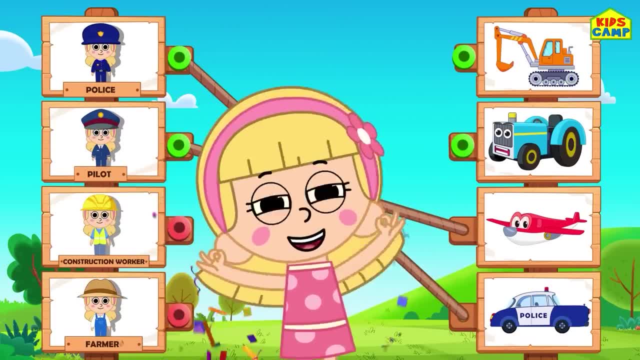 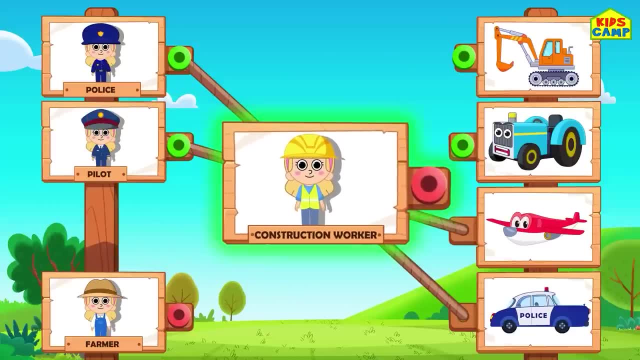 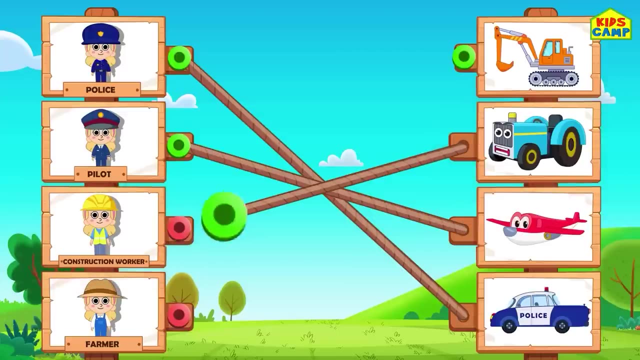 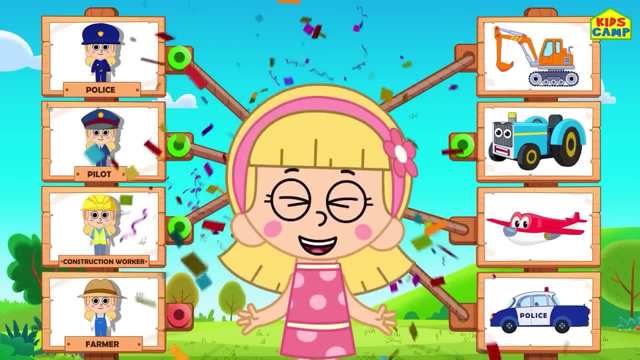 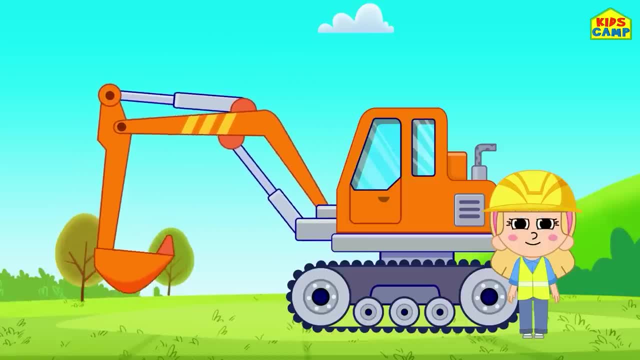 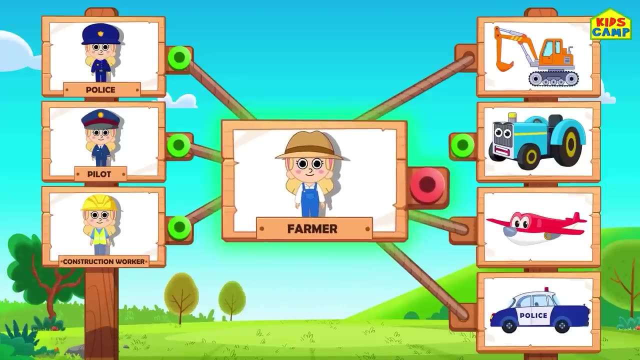 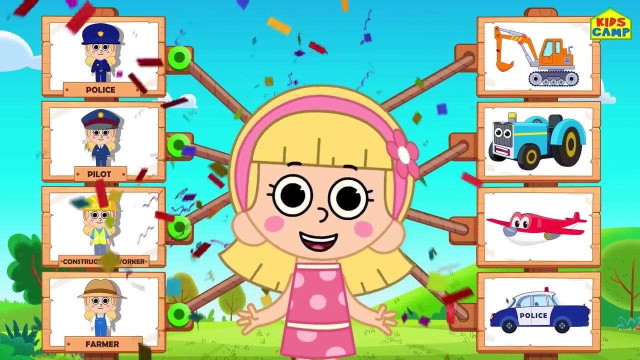 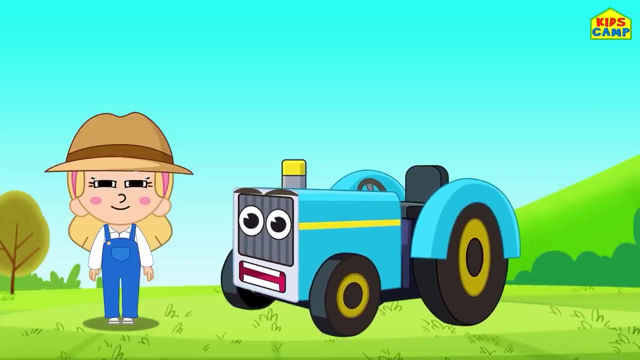 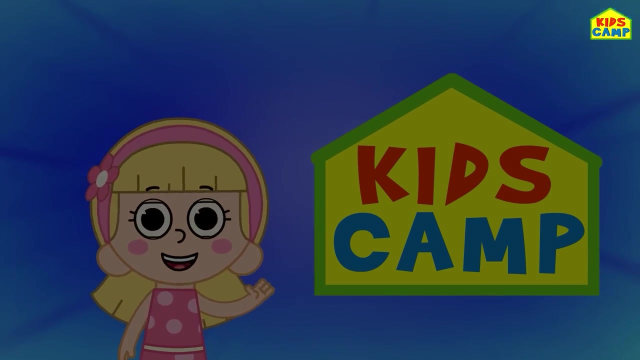 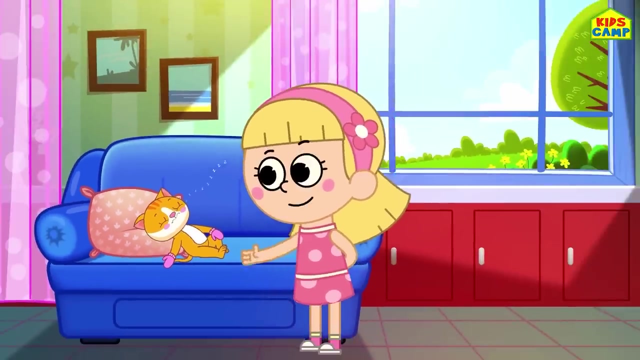 A esos? No, That's right. Yay, Yay, Superb. What vehicle will a farmer use? A tractor, That's right. That was so much fun. Keep watching Kids Camp Bye. Good morning, Kitty, Wake up. 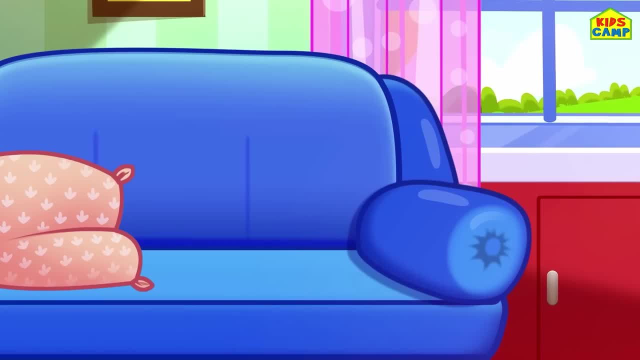 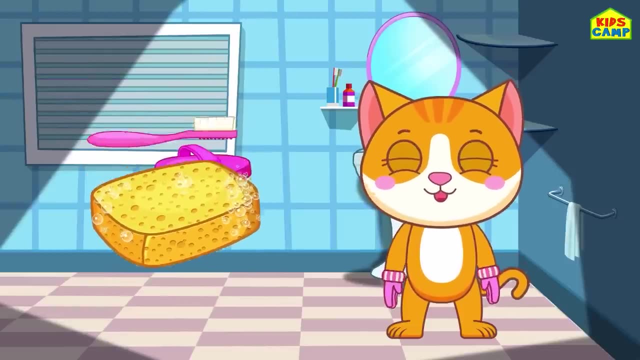 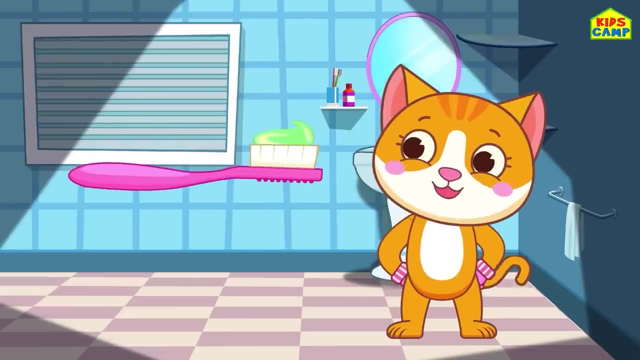 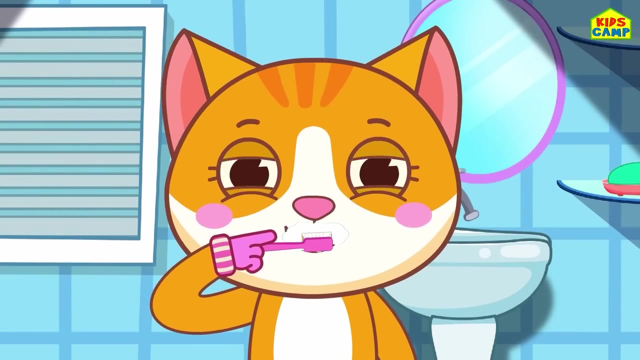 Let's brush your teeth Ready. What do we brush your teeth with? Is this a toothbrush? No, Is this a toothbrush? No, no. Is this a toothbrush? Yes, it is. Yay, Wow, Your teeth are sparkling white. 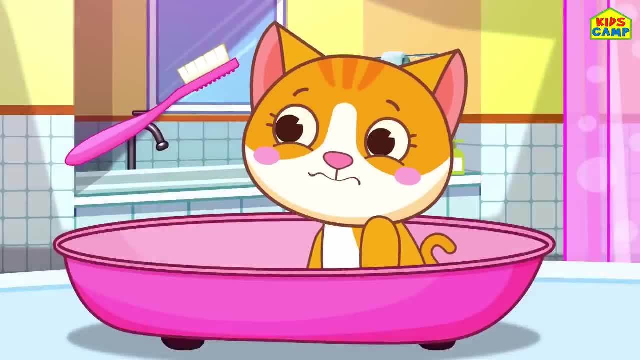 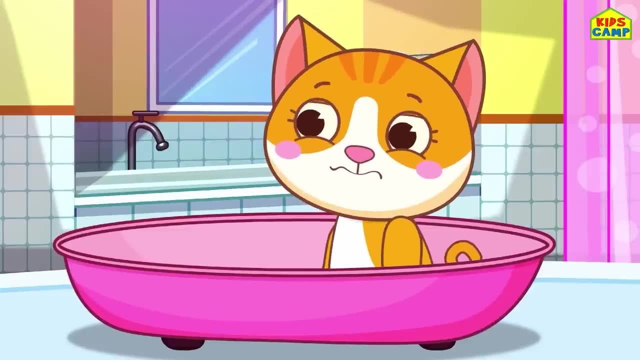 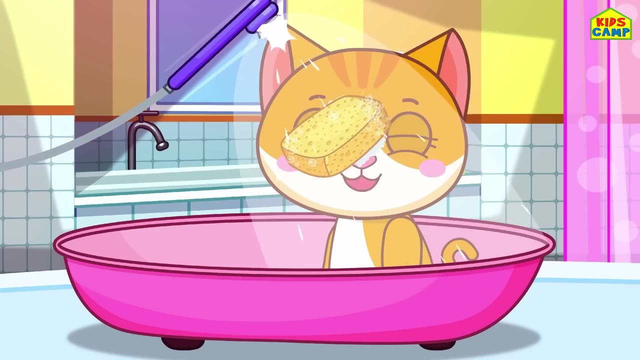 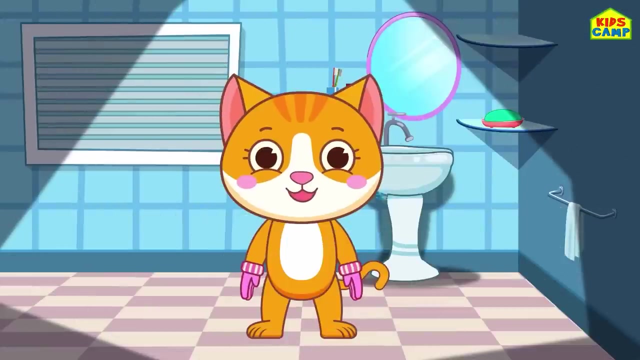 Now let's have a bath. What do we have a bath with This one? No, This one, Definitely not This one. Yes, Don't you love taking a bath? Wow, You're neat and clean, Kitty. Now let's have breakfast. 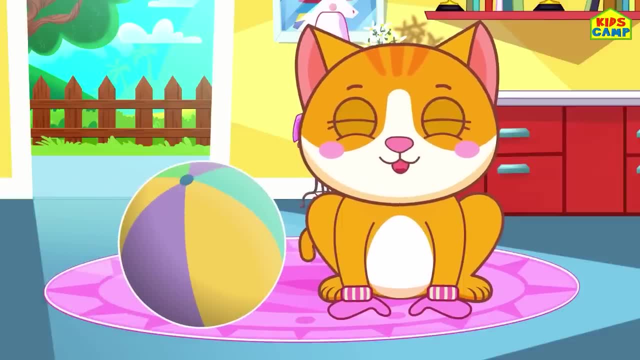 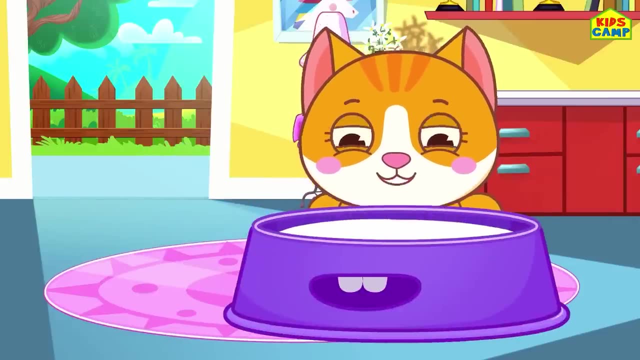 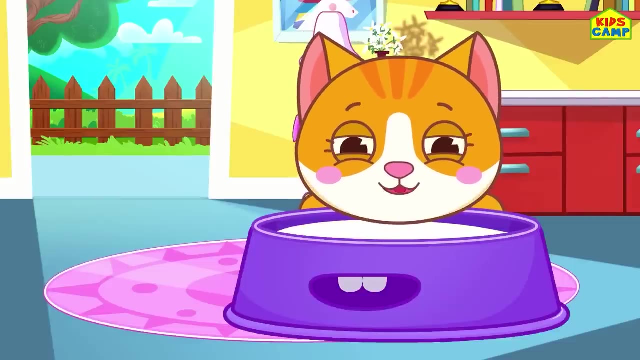 What do we have for breakfast? This one, No. This one, No, no. Then let's have milk. Yes, Milk is best Good, Don't you love drinking milk? Now let's play. What do we play with? 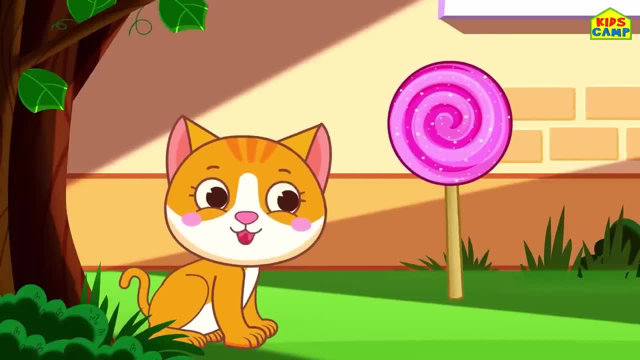 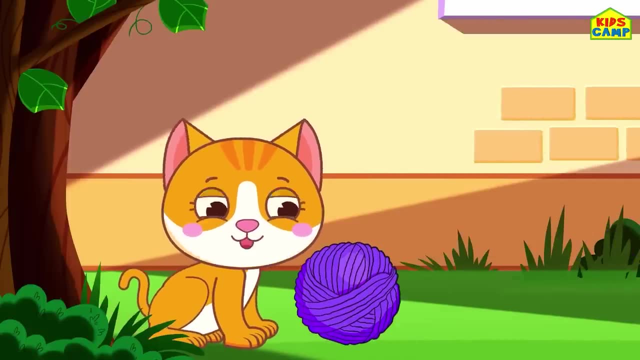 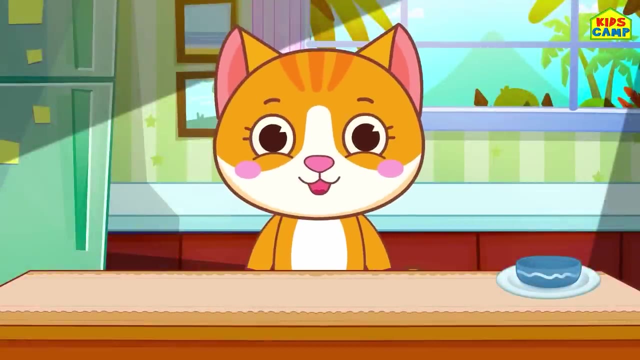 This: No, it's a broccoli. No, we can't play with this. It's a candy. Yes, we can play with this. It's a ball of string. Wow, So much fun. Now let's eat something. Are you hungry? 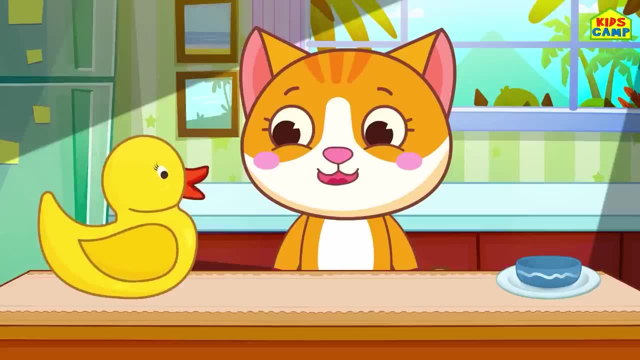 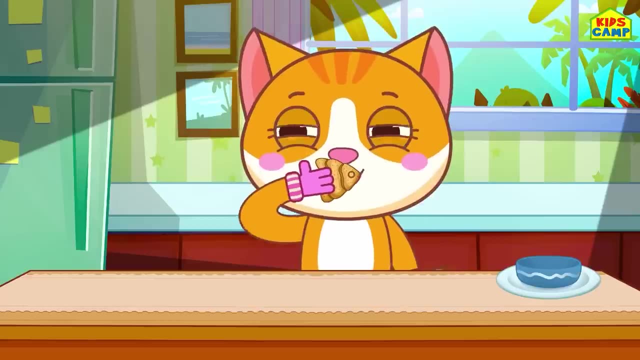 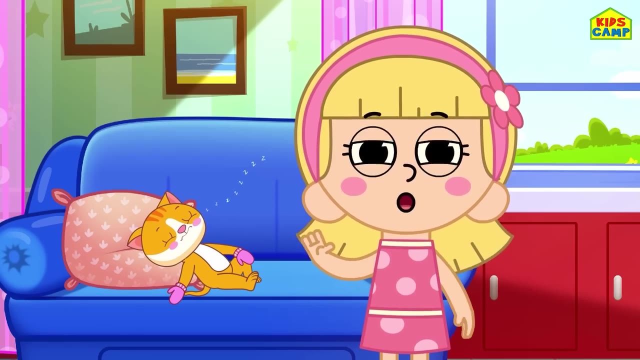 Can you eat this? No, Can you eat this? No, no, Yes, you can eat this. Don't you love the fish? biscuit, Yummy. Wasn't it a fun day with my kitten. See you soon. Bye. 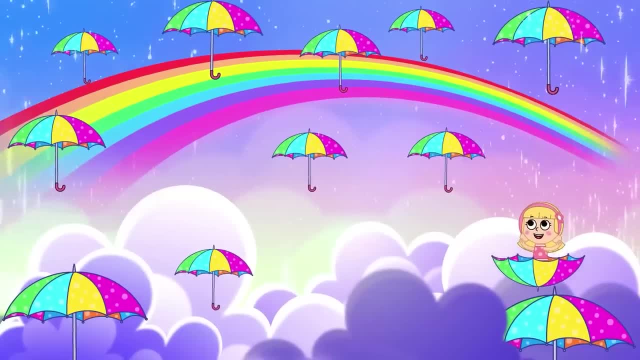 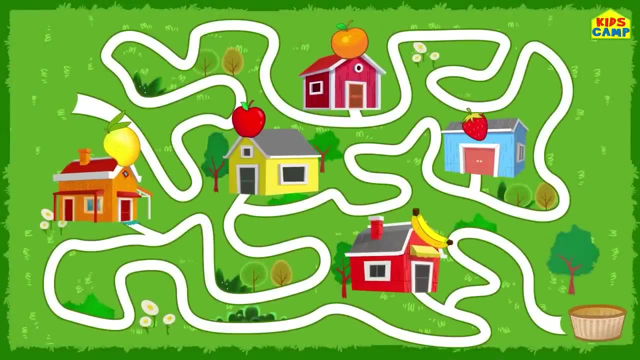 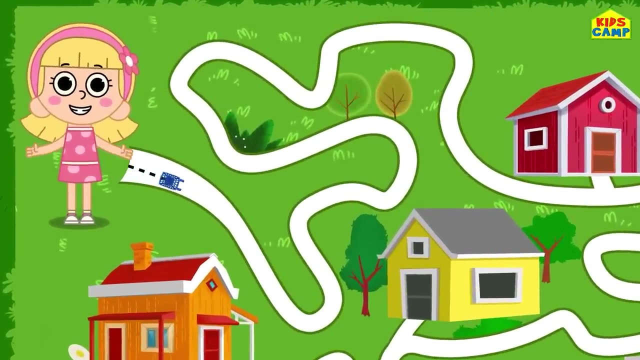 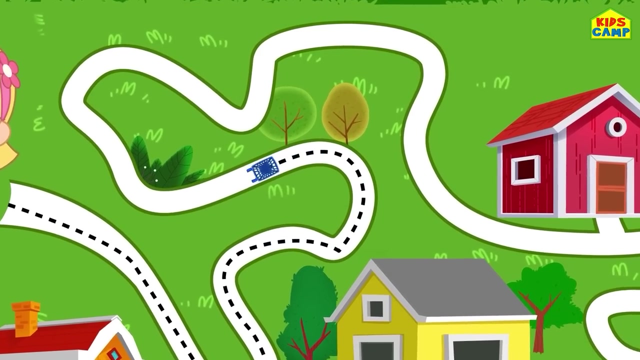 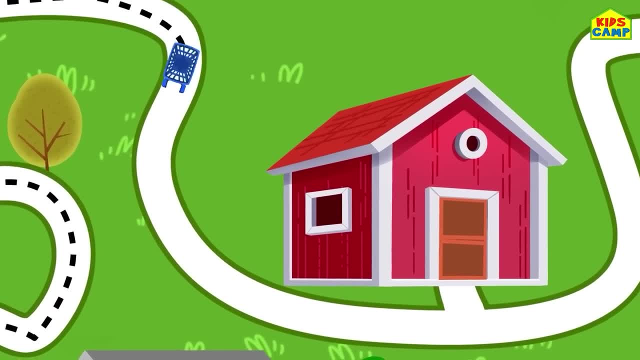 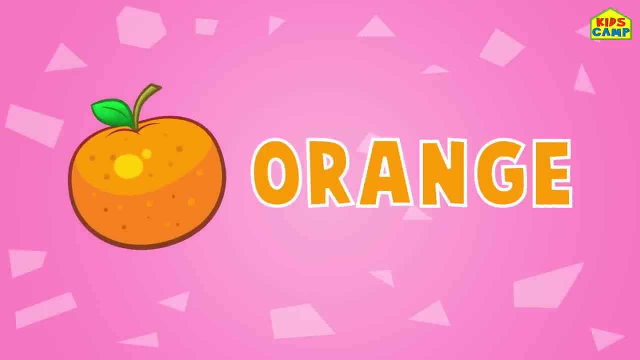 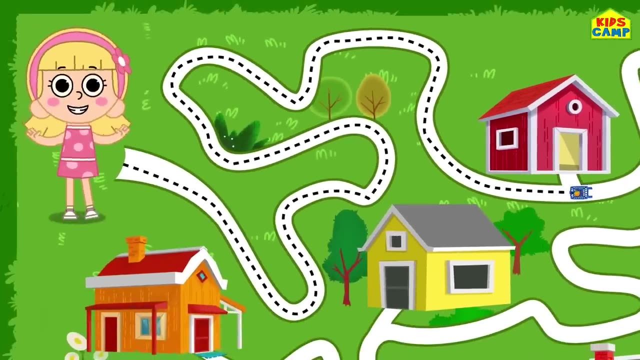 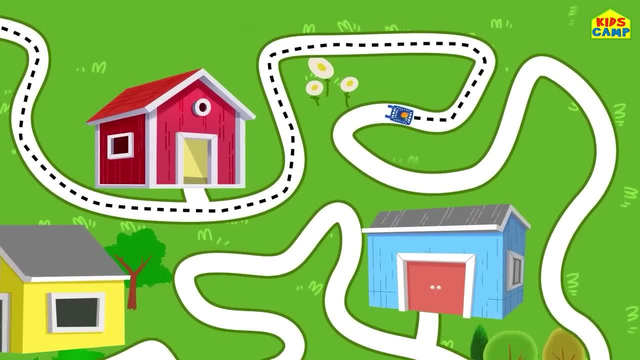 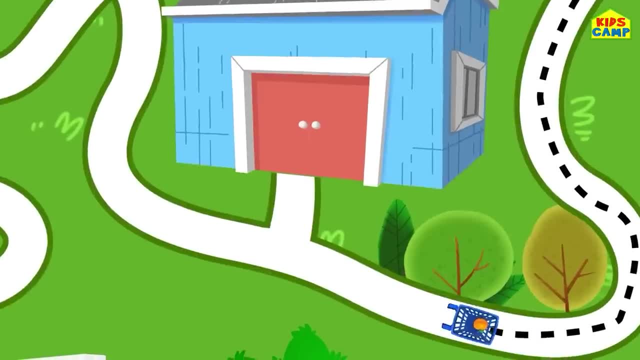 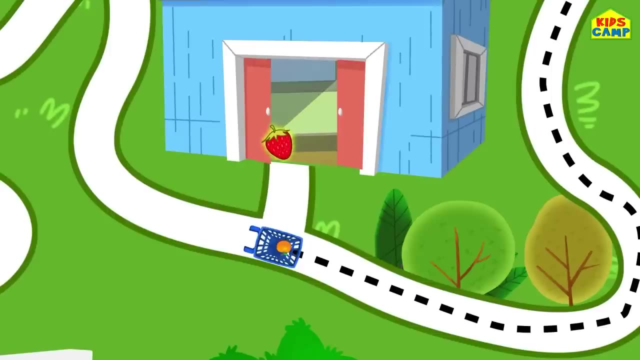 No, No, No, No, No, No, Knock knock. do you have any fruit? Aha, A strawberry Into the cart, Wonderful, Let's get going. Knock knock, Hi, Do you have a fruit? Oh, 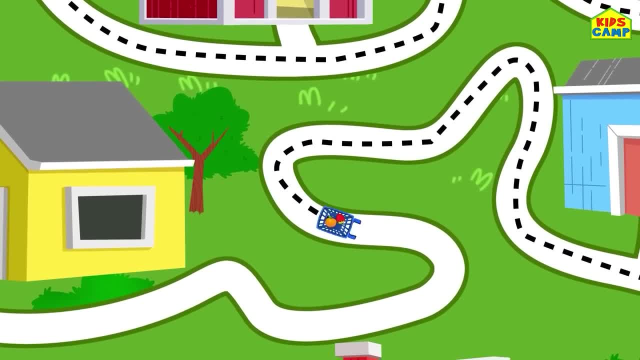 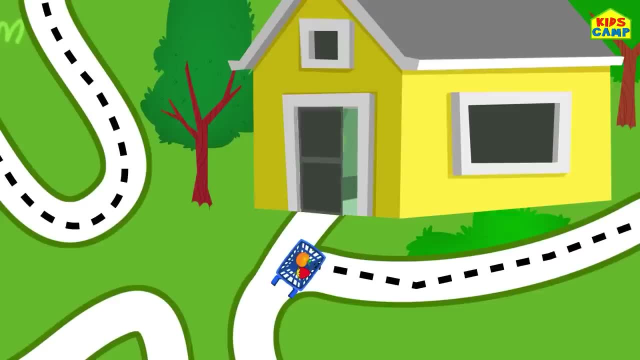 My favorite: An apple Into the cart. Yay, Let's keep going. Knock, knock, Do you have any fruit? There's a flower, Yes, there's a flower. Ooh, My favorite: An apple Into the cart. 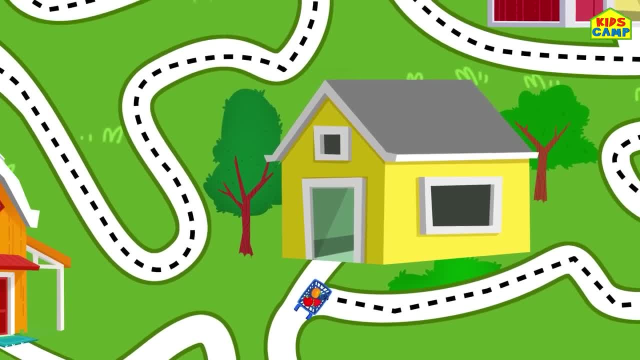 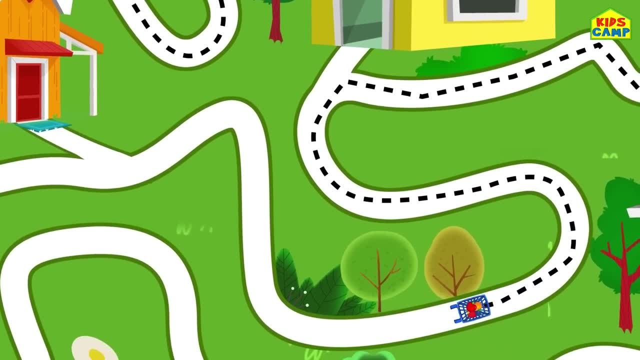 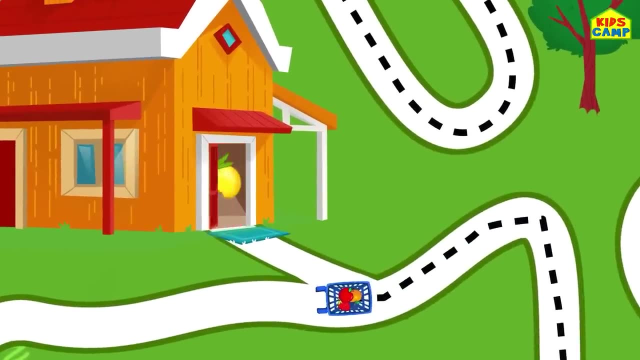 Yay, Let's keep going. Knock knock, Hi, Do you have a fruit? Ooh, My favorite, An apple Into the cart. Yay, Let's keep going. Knock knock, Hi, Do you have some fruit? 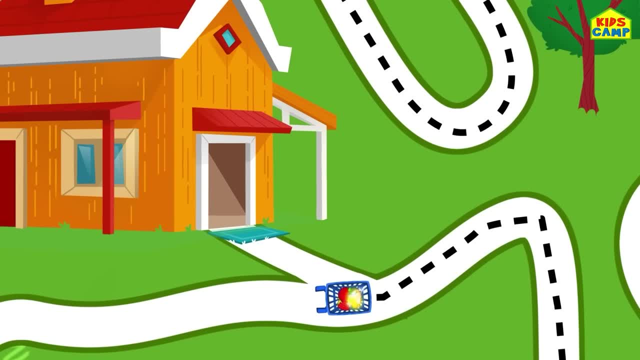 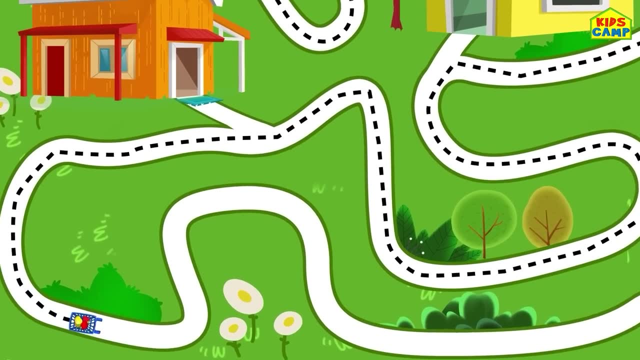 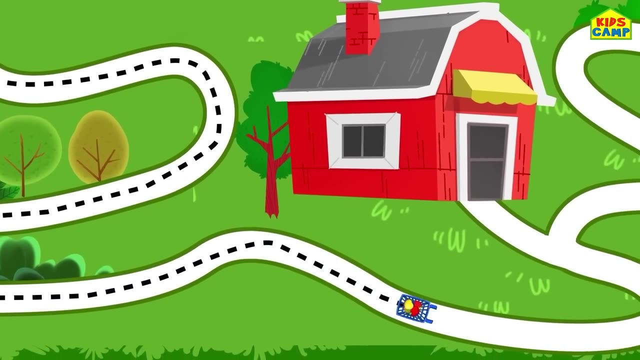 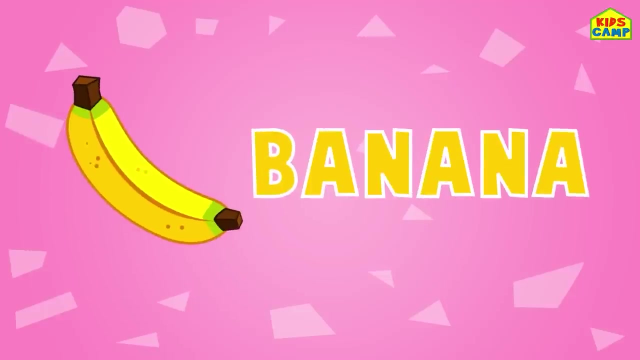 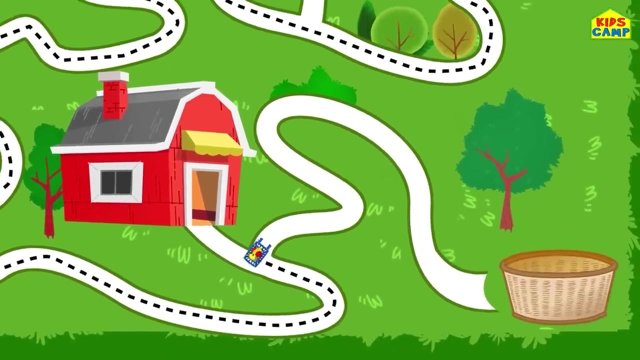 Ooh, a mango Into the cart, Let's get some more. Keep going. Knock, knock, Hi. Do you have some fruit? A banana, Yay, Into the cart, Let's keep going. Yay, We've collected all our fruits. 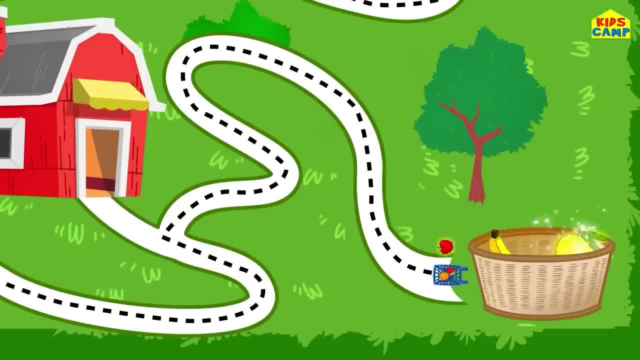 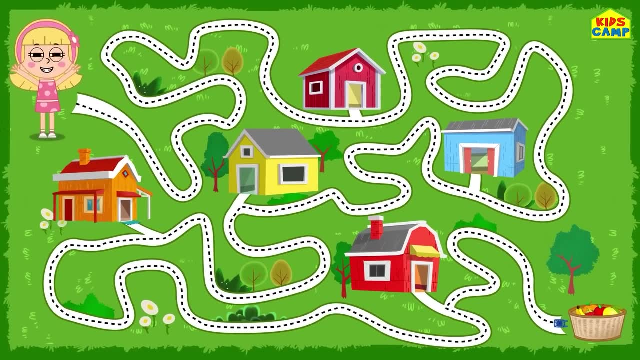 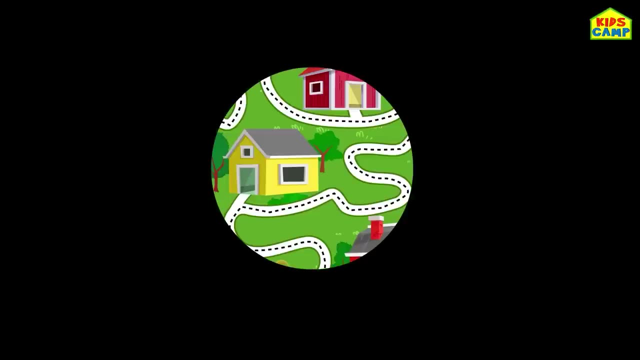 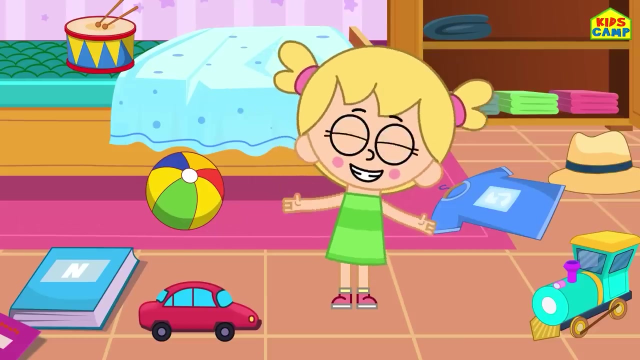 What did we get? A banana, a mango, an apple, a strawberry and an orange. Good job, Thank you so much for helping me find my fruits and collecting them in my basket. Thank you, Hi friends, I'm Ellie and this is Eva. 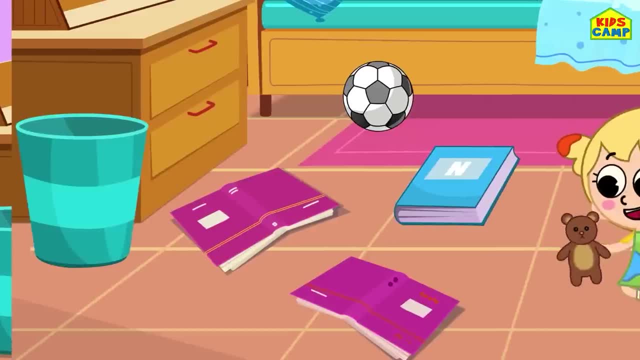 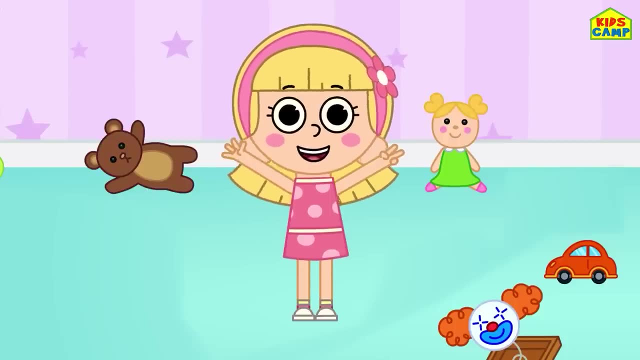 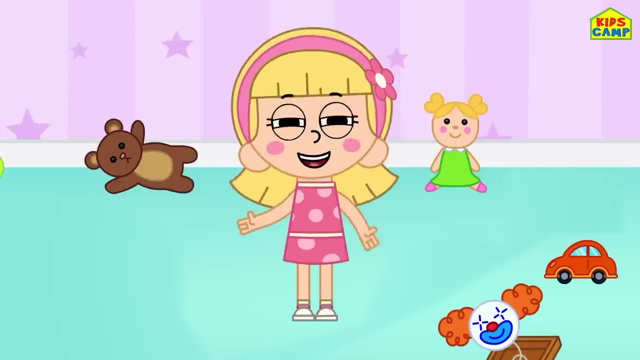 Eva, Look at your room. You have to clean the room now. I know a fun way to clean our room: Let's find the objects and put them where they belong. Eva, Let's clean our room. Let's do this, friends. 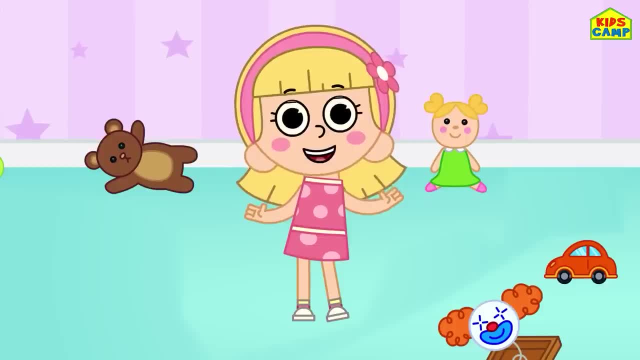 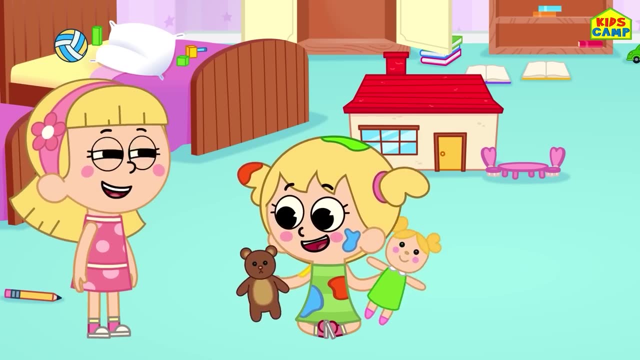 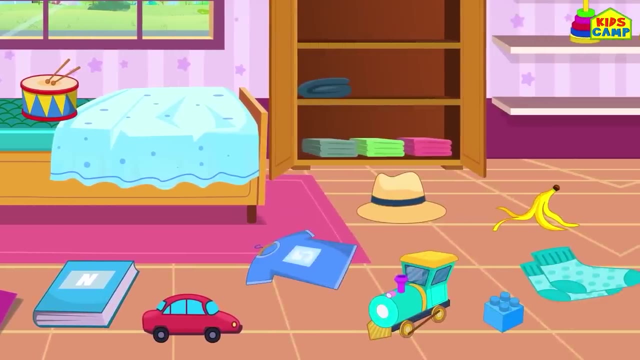 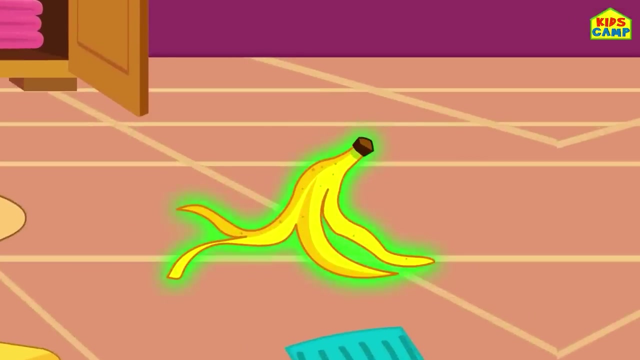 Ready, Let's get started. Yay, Come on, Eva. Eva, You know what you have to do, That's right. Yay, Let's get started. Let's get started, Let's go, Let's go, Let's go. 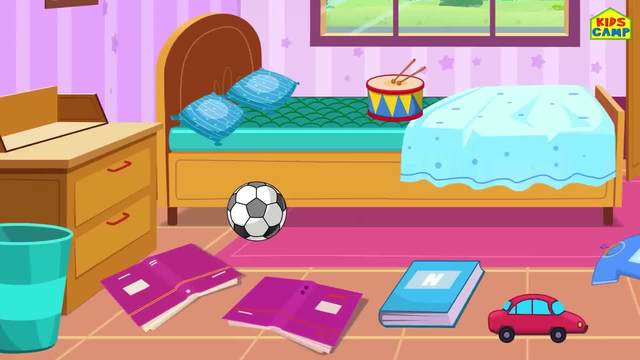 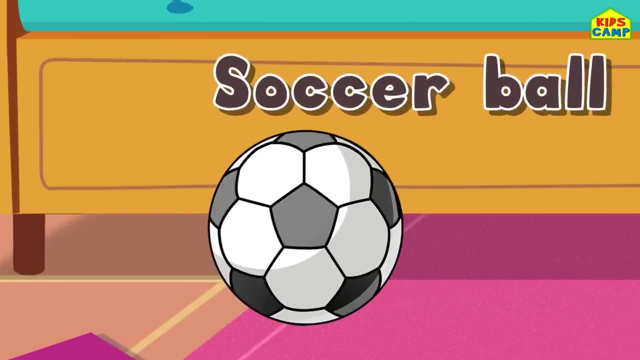 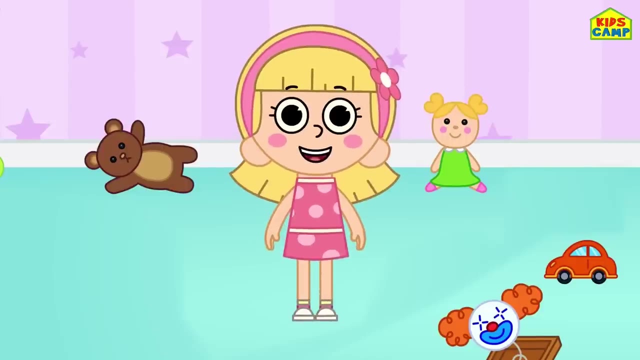 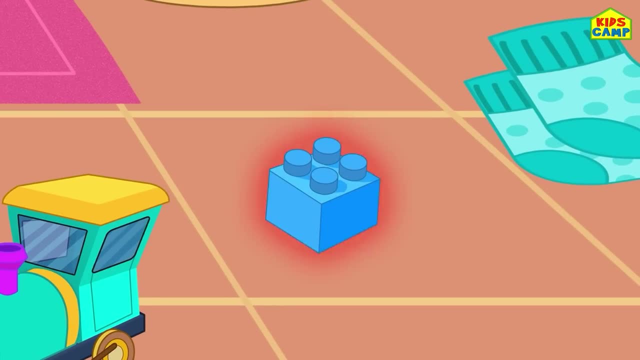 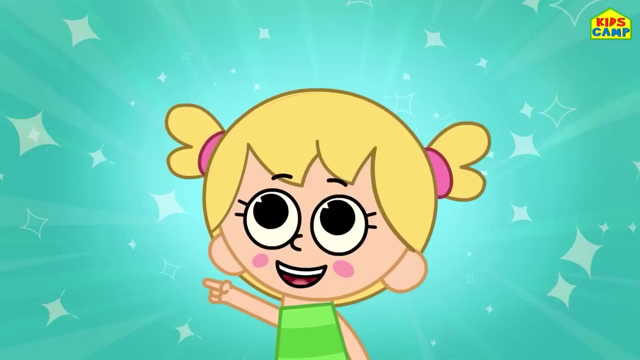 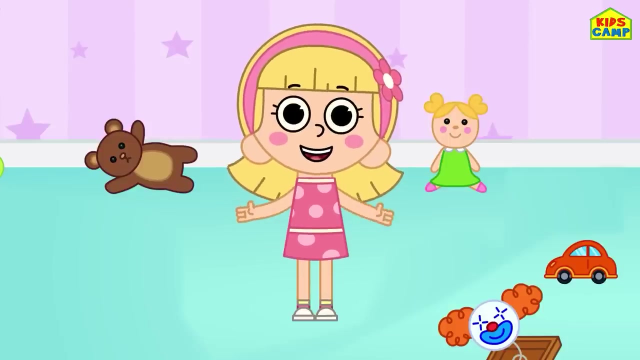 Let's run around. Wow, A parece ipango. It's my favorite robot here. It's real, Make us laugh. Yeah, A, Come on, Eva, We should wash our hands. Yeah, Onto the shelves. Good job, Let's clean some more. 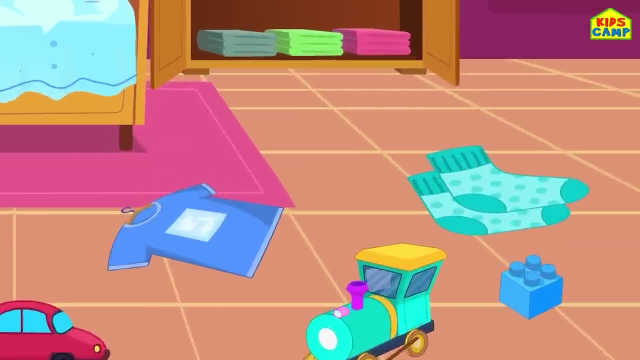 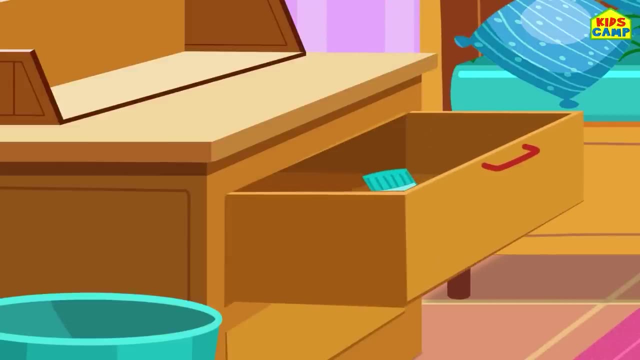 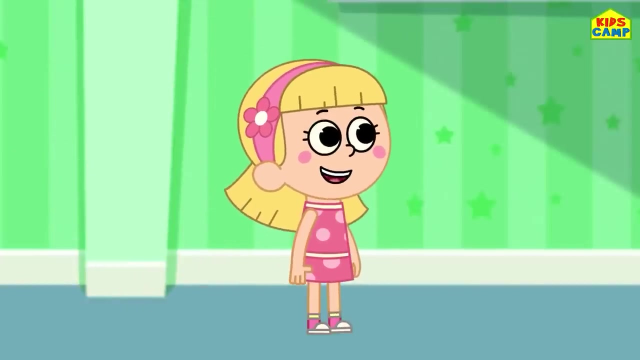 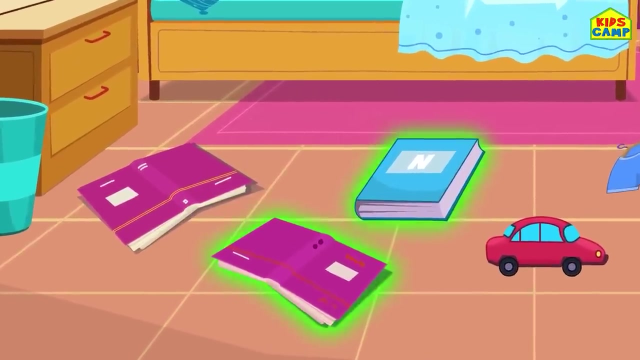 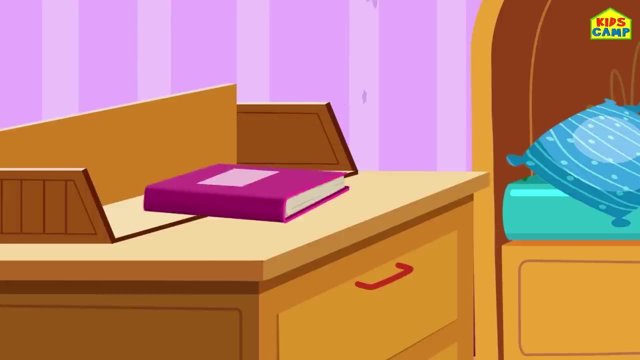 Now, let's look for The socks. That's right Into the drawer. Wonderful, Very good, Eva. where are your books? Look for them. That's right. Here are the books. Let's pick them up. Very good. 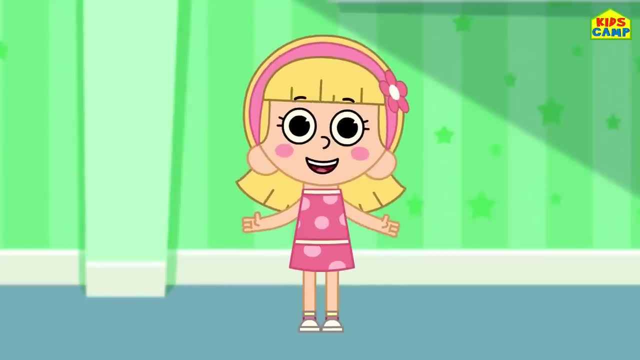 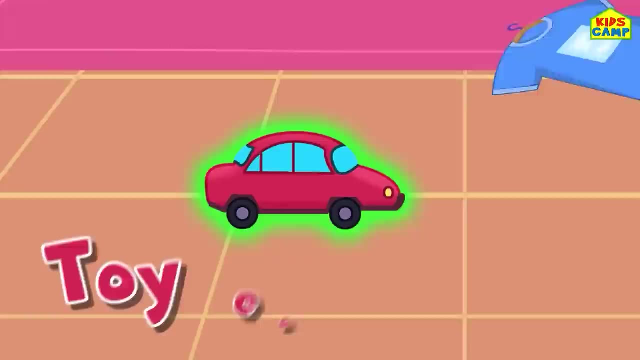 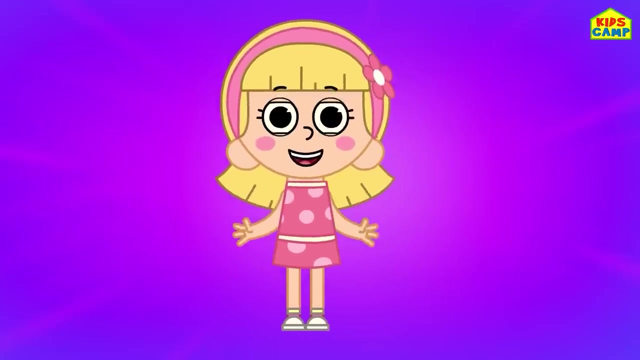 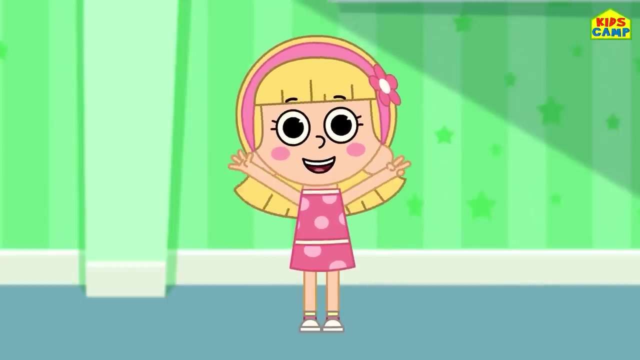 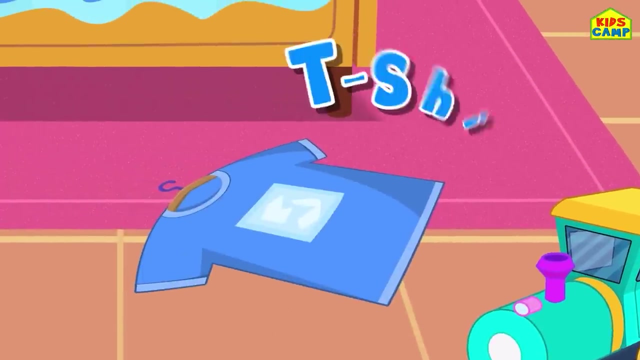 Stack them together. The room already looks clean, Wonderful. Now let's look for the toy car. That's right, Amazing- Onto the shelf. Good job, Eva. Let's clean some more: The block And the t-shirt. 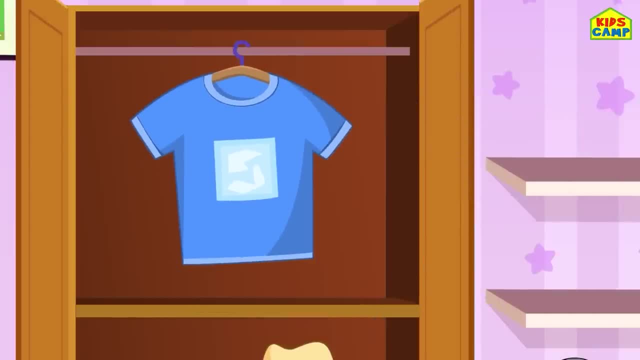 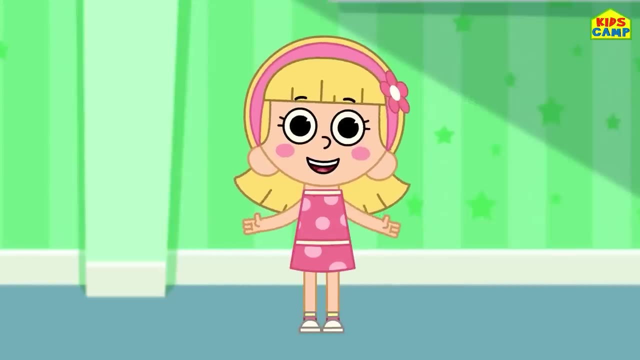 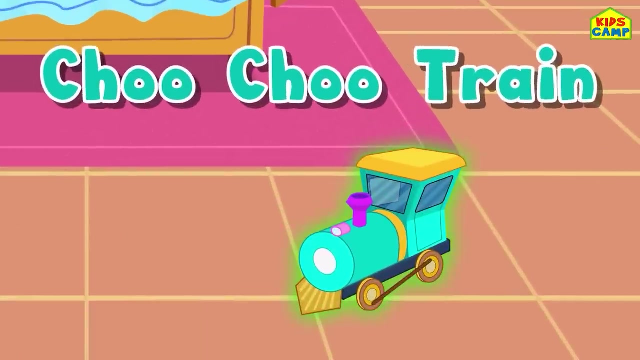 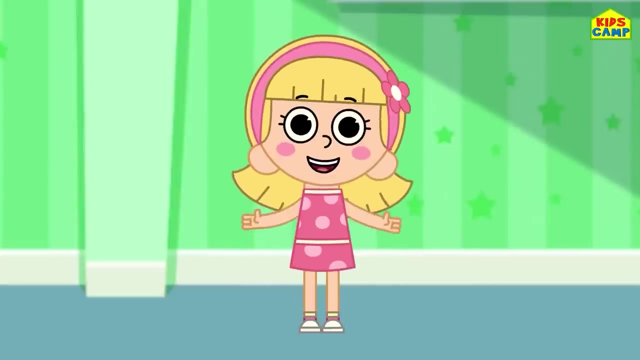 Eva, let's pick them up Into the cupboard And on the shelf. Good girl, Wonderful, Let's clean some more. The juju train Onto the shelf. We did it, We're almost there. Good job, friends. 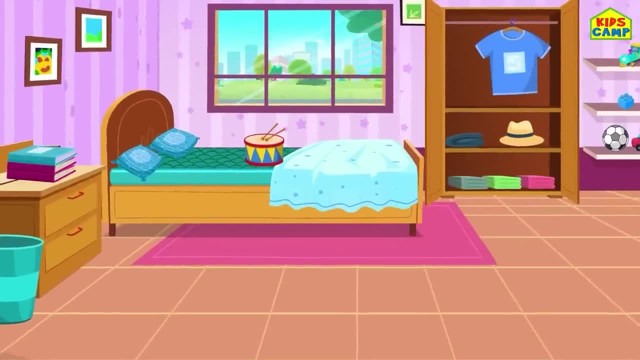 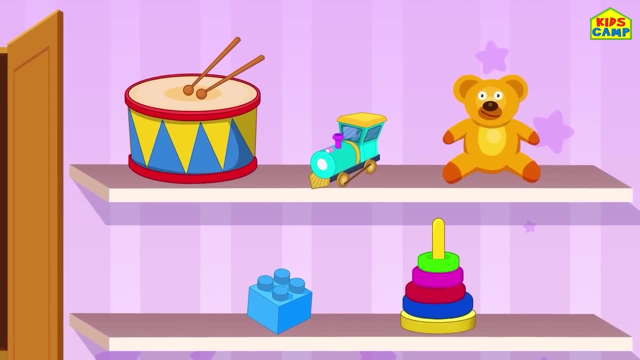 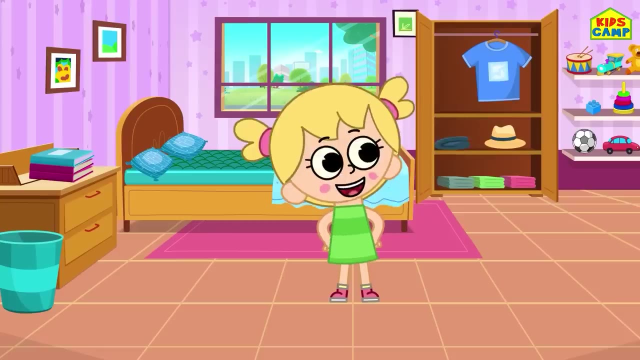 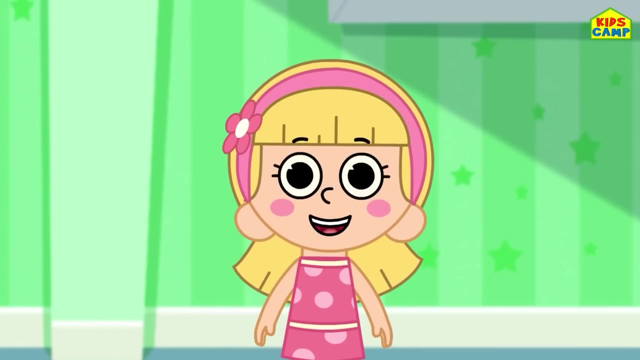 Wonderful, The toy drum. Let's pick it up And put it on the shelf. That's right, Our room looks clean. Yay, Good job, Eva. Wonderful, That's how you clean your room. Wasn't that fun kids. 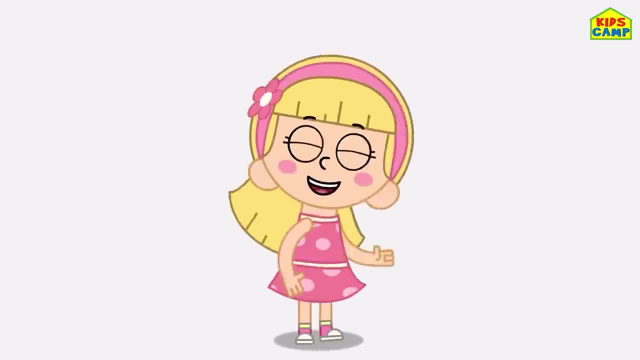 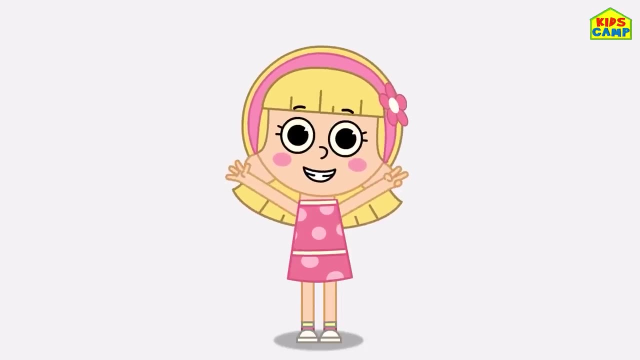 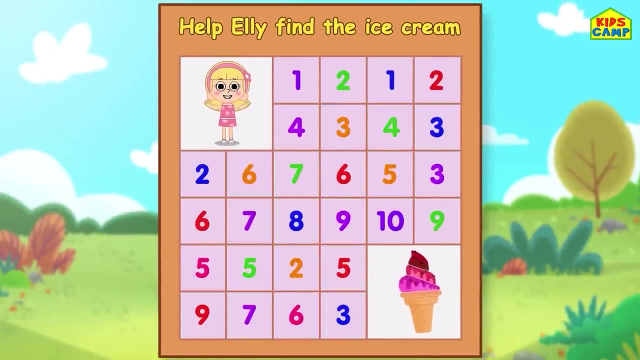 Bye, Hi friends. I'm Ellie. Would you like to help me reach the ice cream? Yes, Then let's get started with this amazing number maze. Yay, Let's get started. Let's start with the number one. Yes, 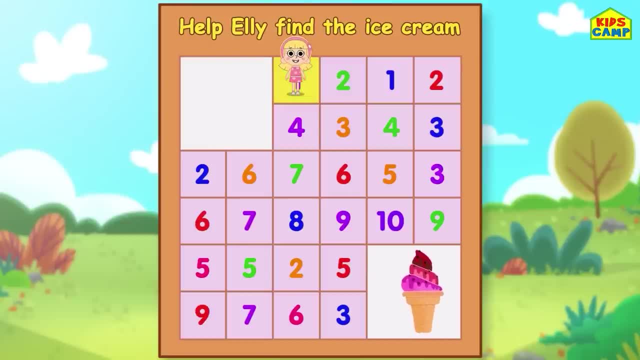 I'm on number one. Let's go to the next, number Two: Yay, Ooh, That's not right. Aha, That's right, That's three. Let's go to the next one, Number four: Yay. 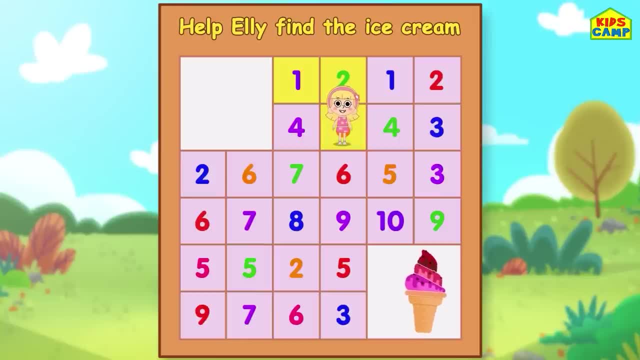 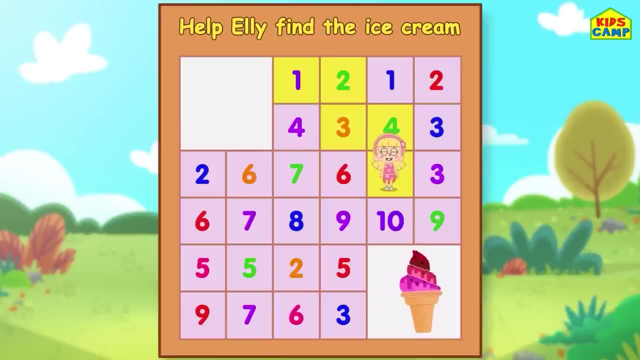 Yay, Yay, Number five, Good job friends. Oops, That's not right. The next number is six. That's right, Wonderful. Next Seven, We're almost there. Andeight, Yay, Uh, oh no. 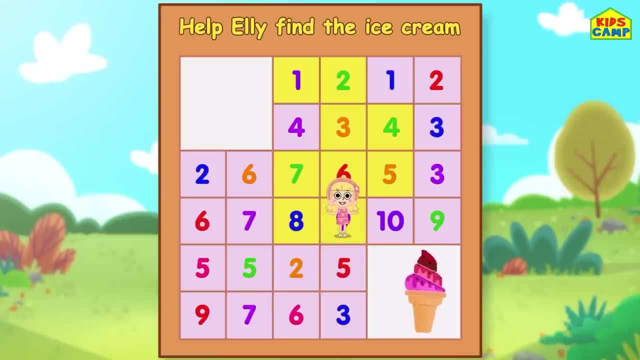 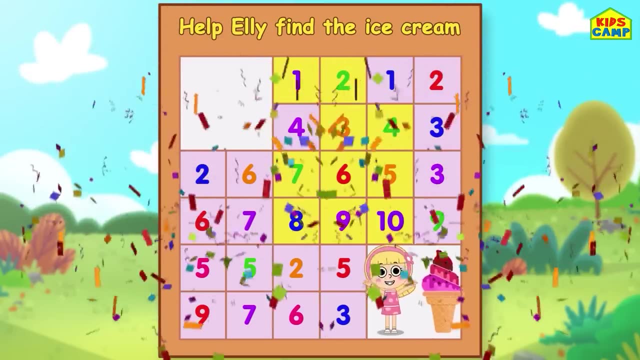 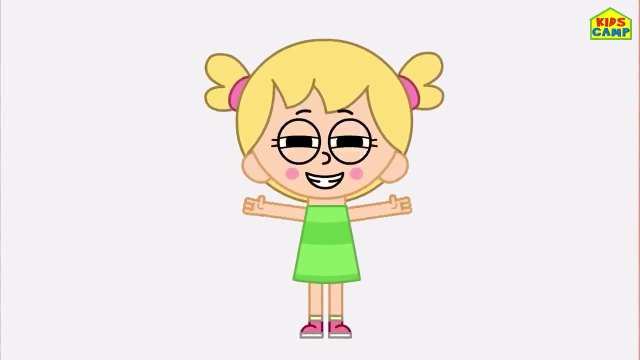 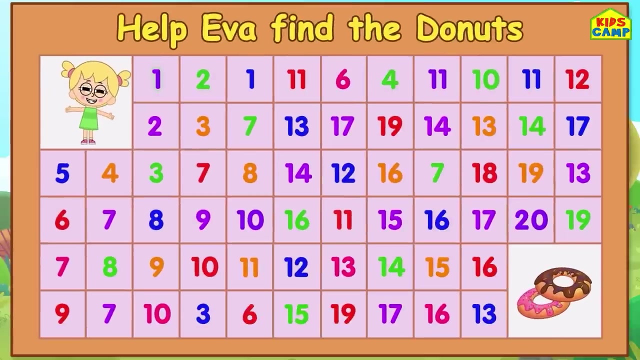 That's right. Nine And ten. Yay, We did it. You helped me reach the ice cream, Thank you. Oh, it's Eva's turn now. Can you help her reach the donuts? Let's get started. Yay, Let's start with number one. 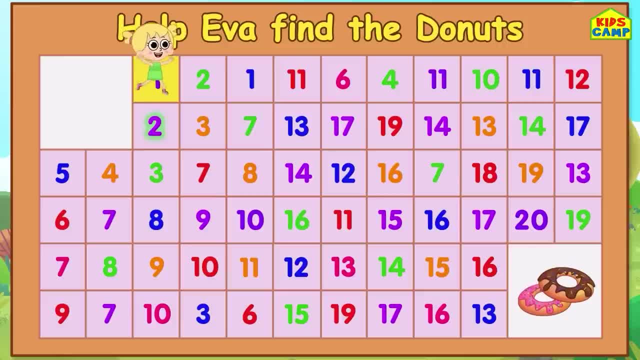 One, two, three, good four, uh-oh, no, no, no, that's right. number five, good six, keep going. seven, eight, yay, Oops, That's not right, That's right: Nine. 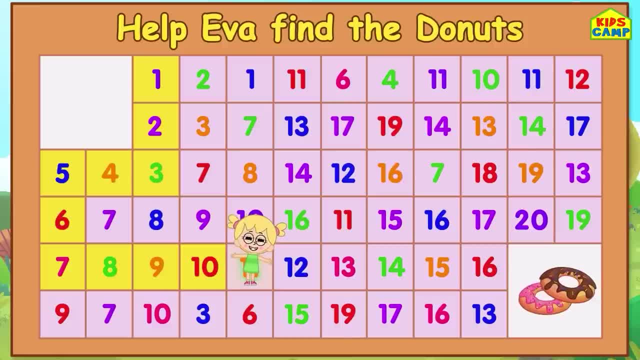 And ten, Eleven, Keep going. Yay, We're on twelve. What comes after twelve? Uh-oh, no, not that one, That's right. Thirteen And fourteen. Next is fifteen. Woohoo, Only five more to go. 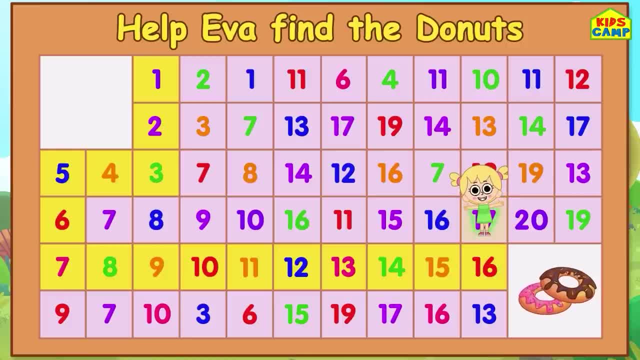 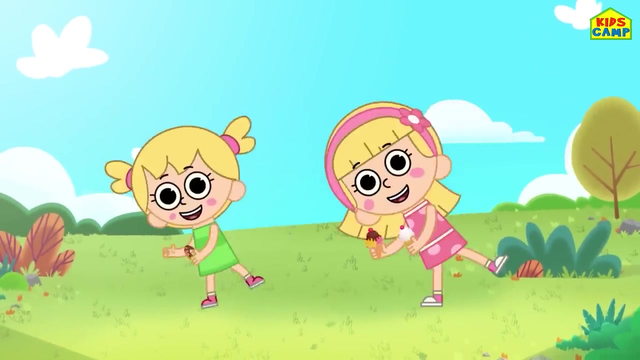 Sixteen, That's right. Seventeen. Next is eighteen, That's right. Nineteen, We're almost there. And twenty, That's right, We did it. Woohoo, Woohoo, We helped Eva find the doughnuts. 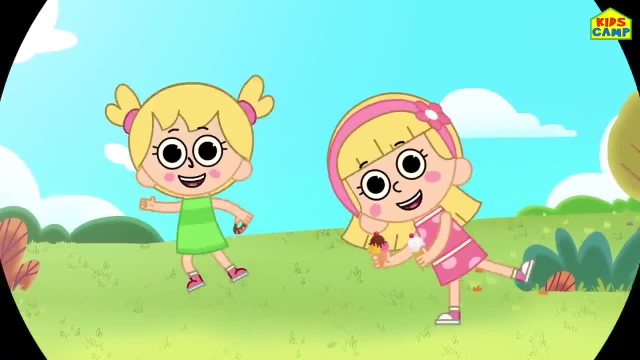 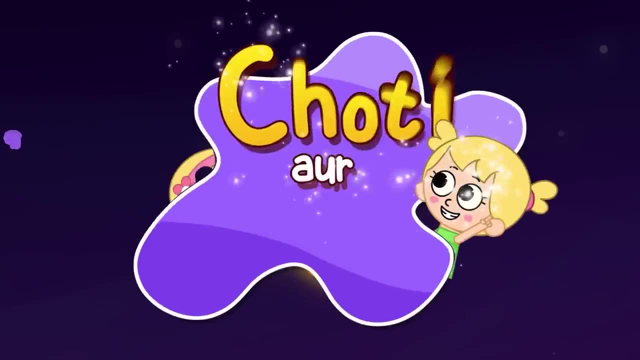 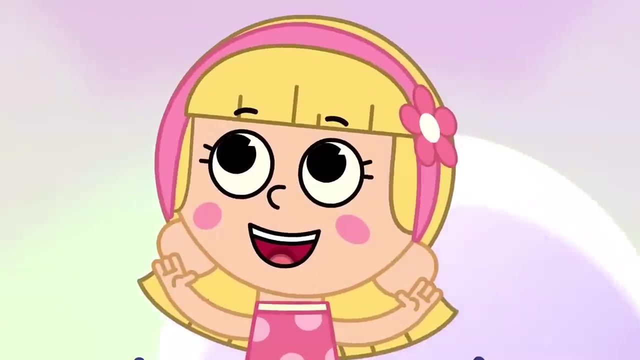 Good job, friends. Bye Up next. Baarish Aai By Choti Aur Badi Baarish Aai. Baarish Aai Chum Chum Chum, Lekar chhata saith nikle, hum, hum. hum. 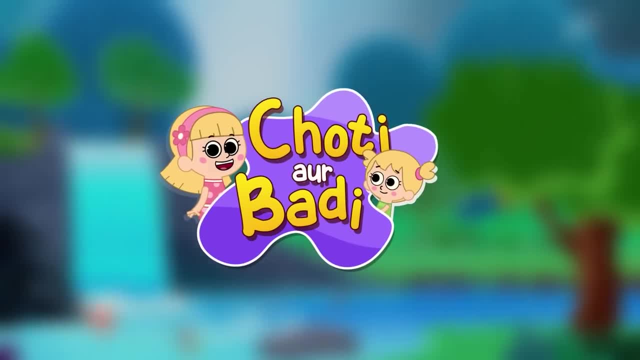 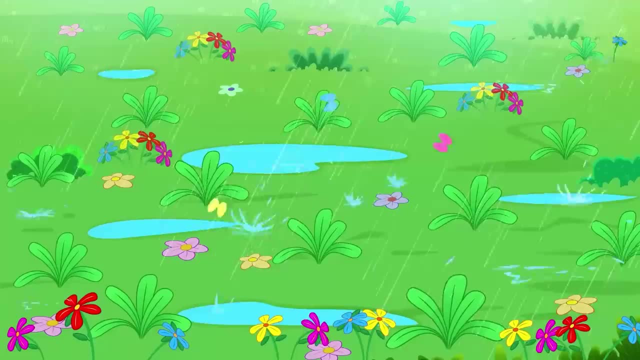 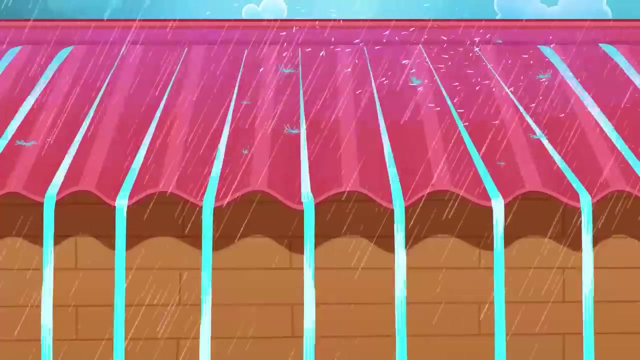 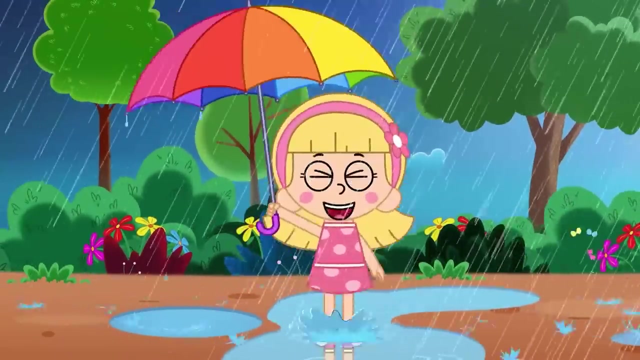 You're listening to Baarish Aai by our YouTube channel: Choti Aur Badi. Baarish Aai, Baarish Aai, Chum Chum, Chum, Lekar chhata saith nikle, hum, hum. hum. 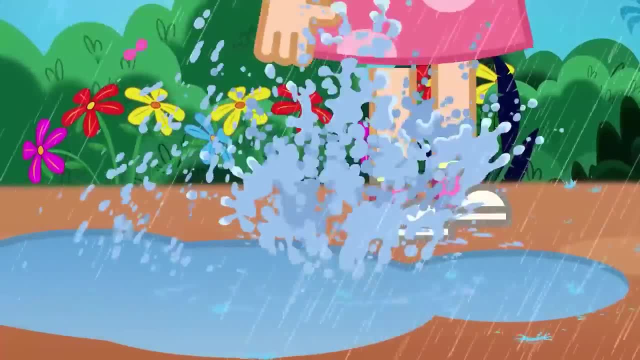 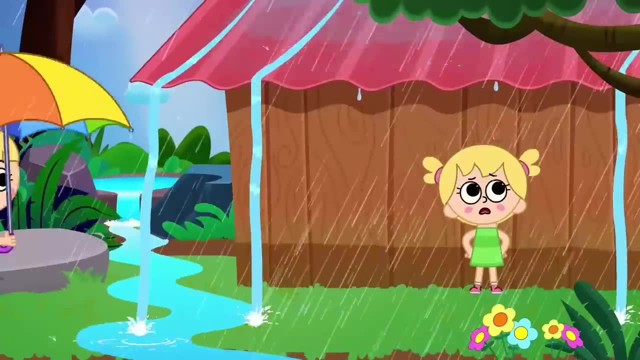 Baarish Aai. Baarish Aai Chum Chum Chum Lekar chhata saith nikle hum, hum, hum, YeY DeKho dekho Baarish Aai. 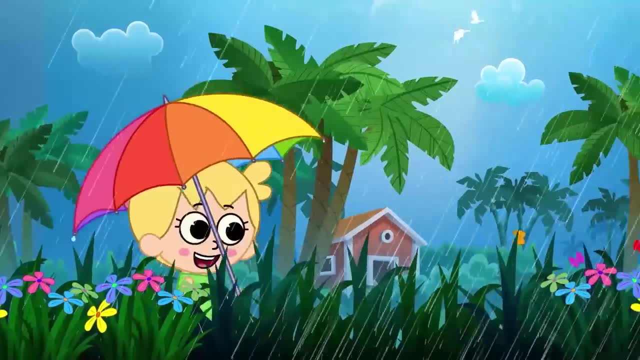 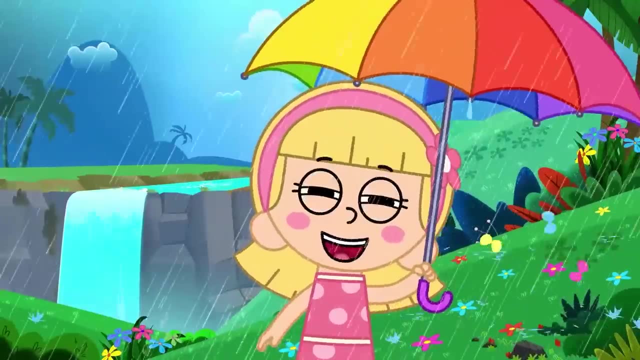 Har jag haun khush haun illay Ye Dekho, dekho, Baarish Aai. Har jag haun khush haun illay Kheto me raunak Aai. Every place has a beautiful green shade. 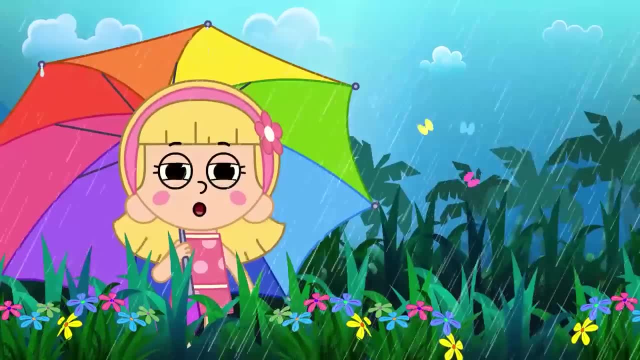 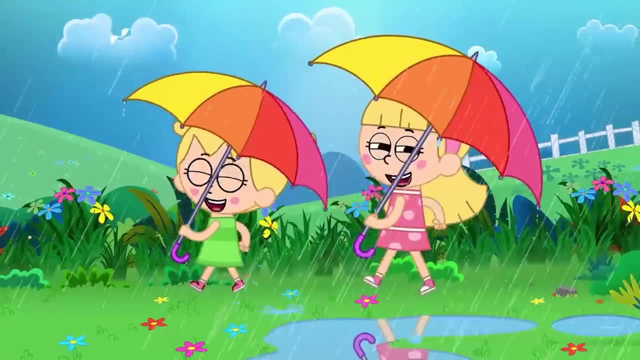 Wow, So much happiness has been brought by the rain. Let's all sing this song together: Yay, The rain has come. the rain has come, Chum, chum, chum. With the umbrella we came out together. Hum, hum, hum. 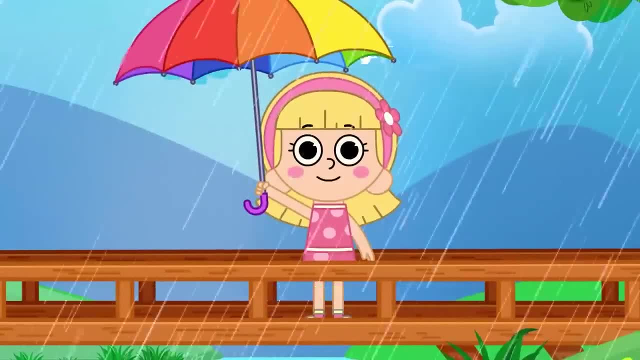 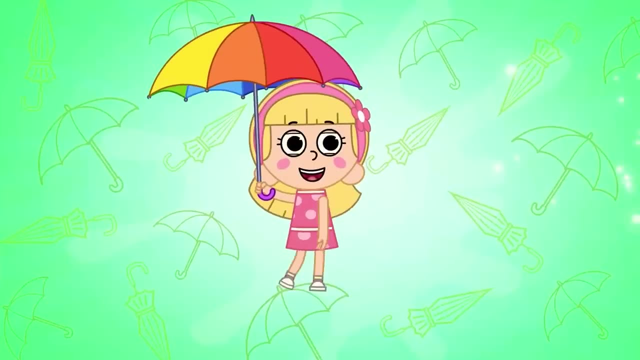 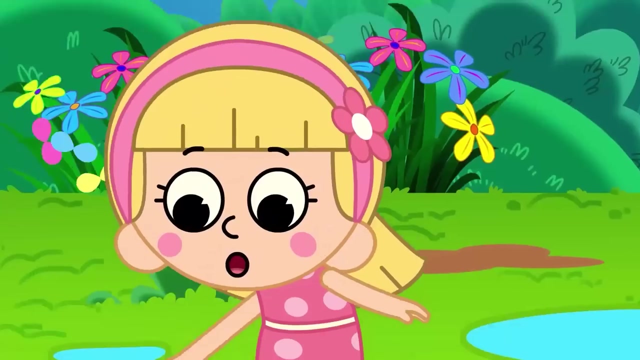 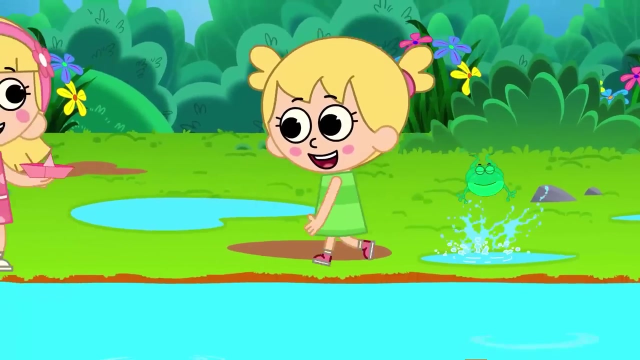 The rain has come. the rain has come. Chum, chum chum. With the umbrella. we came out together. Hum, hum, hum, Come, come, you also come. Let's make our own boat. Wow, Choti, come, you also come. 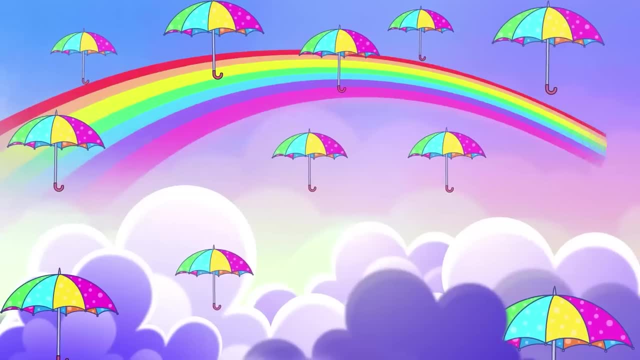 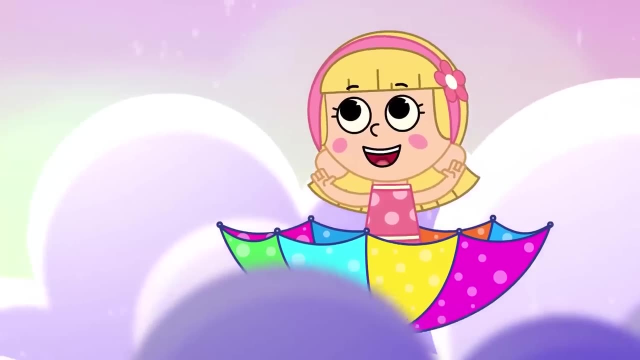 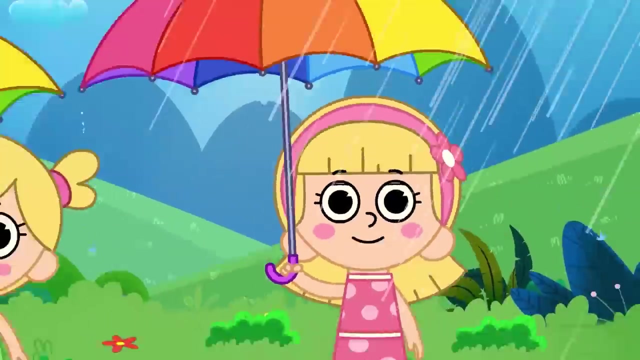 Come, let's make our own boat. Take care of the seven-coloured Indra Dhanush in your eyes. Wow, So much happiness has been brought by the rain. Let's all sing this song together: The rain has come. the rain has come. Chum, chum, chum. 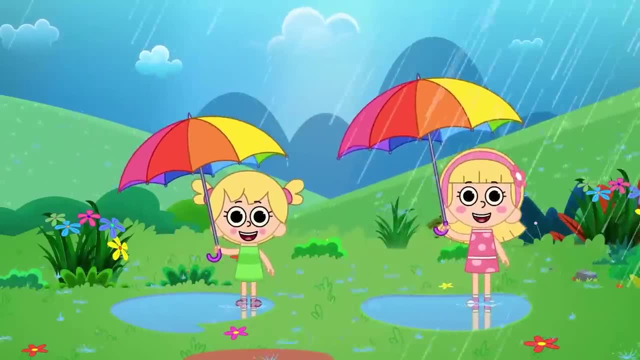 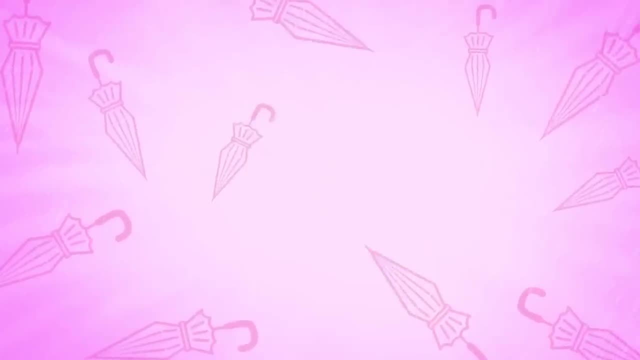 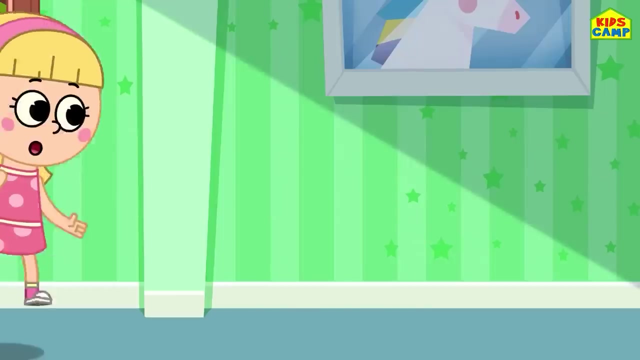 With the umbrella, we came out together. Hum, hum, hum. The rain has come. the rain has come, Chum chum chum. With the umbrella, we came out together. Hum, hum, hum. Hi friends, I'm Ellie, But I can't find my cat. 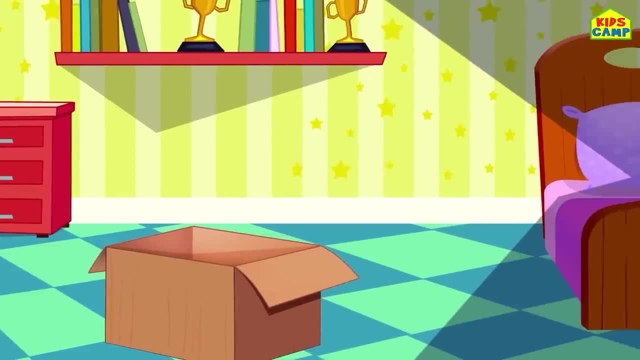 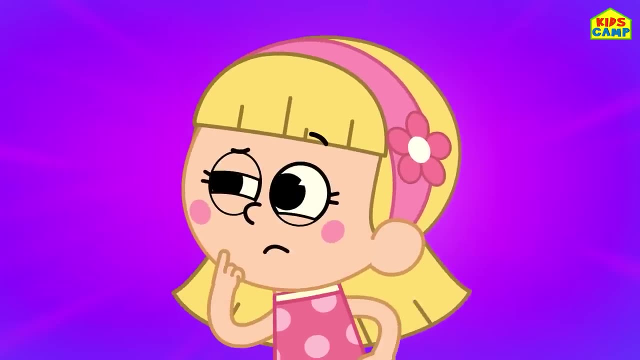 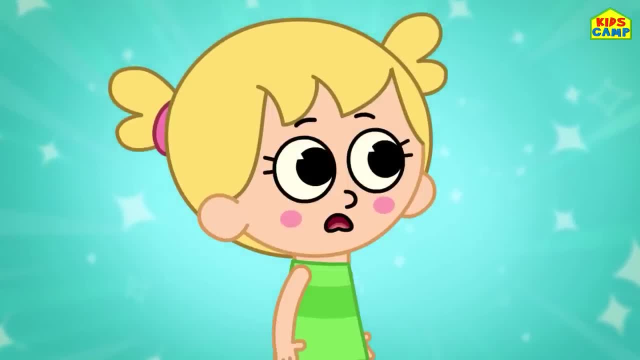 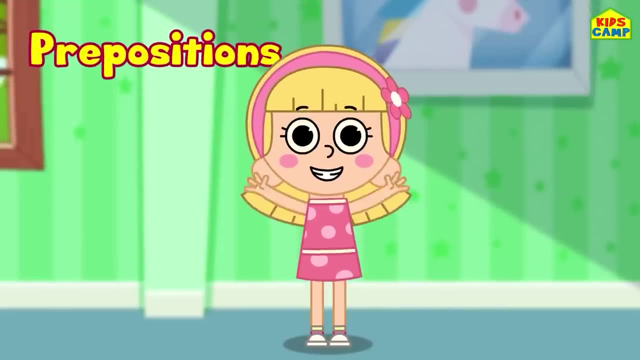 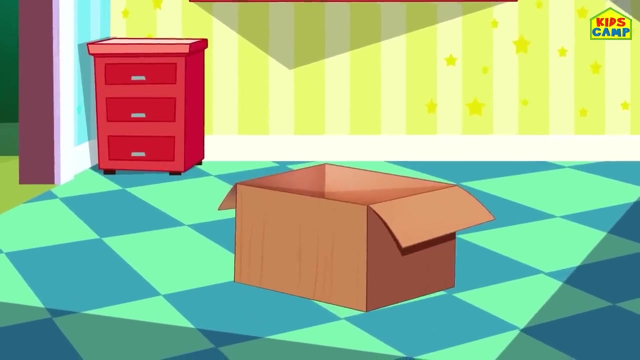 Eva seems to be confused. Don't worry, today we are going to learn Prepositions And how and where to learn Prepositions And how and where to use them. Ready, Let's start. The first preposition is In. The cat is in the box. Do you see that, Eva? 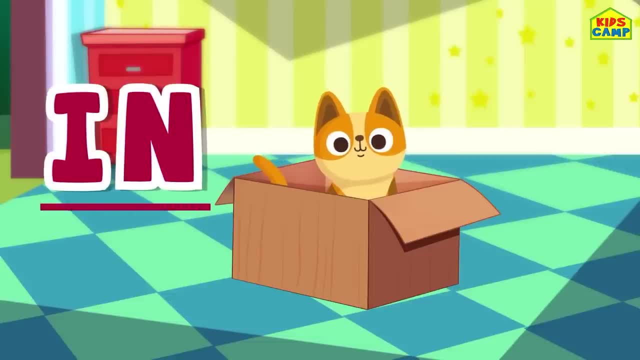 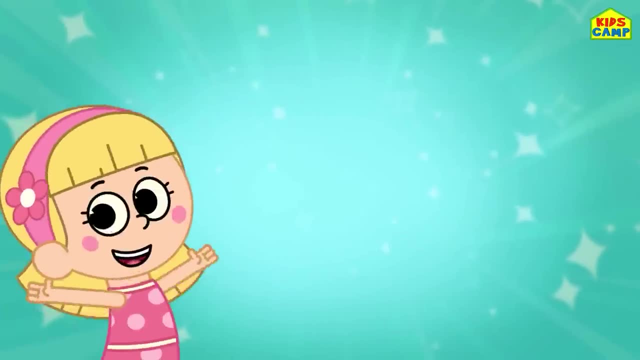 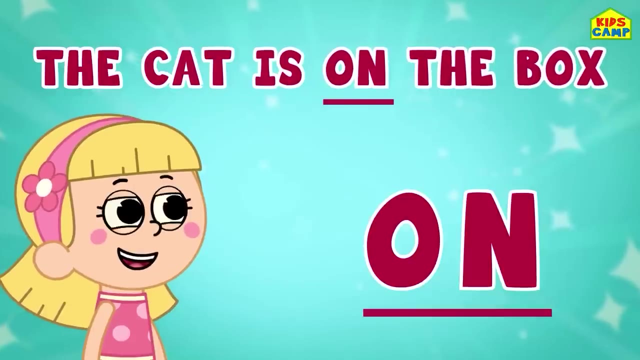 She's in it. In is the preposition, And this is how we use it To show the position. The next one is On. That's right. The cat is on The box. Yay, this is easy, Isn't it? This is how we use the preposition. 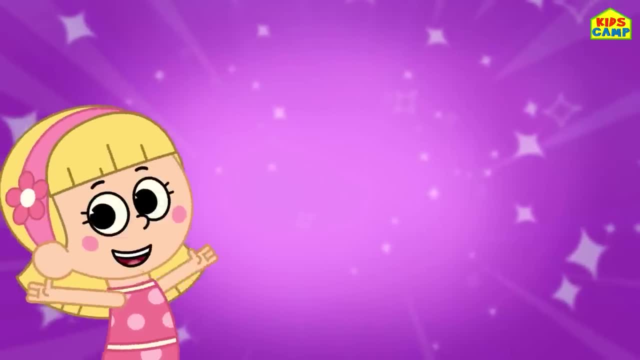 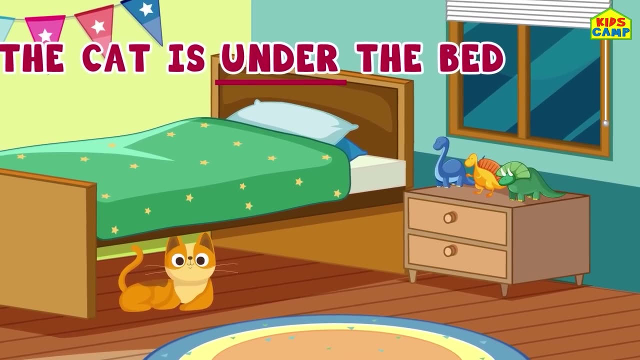 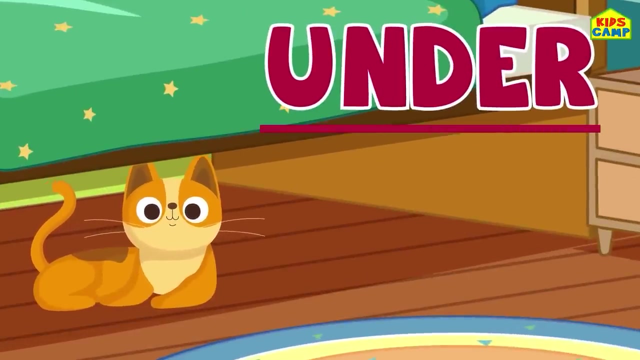 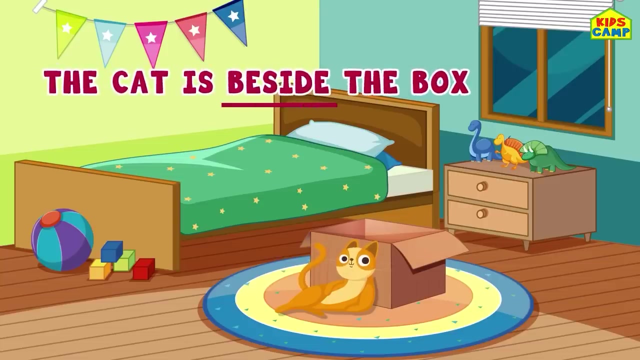 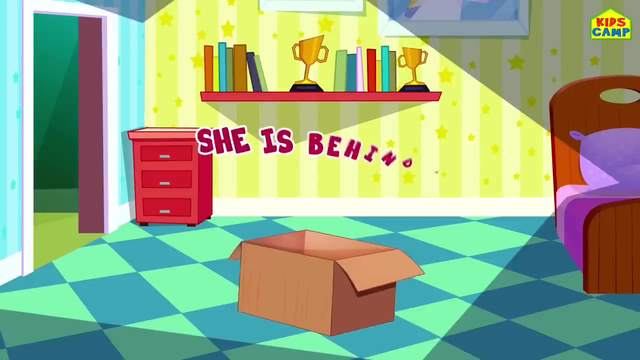 On. Next is Under or beneath. The cat Is under the bed. There she is. We found her. Good job, friends. Where is the cat now? The cat is Beside the box. She is beside it, Right. Where is the cat now? She is Behind the box. There she is. 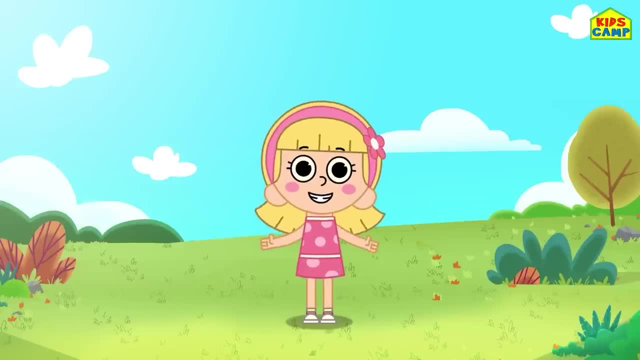 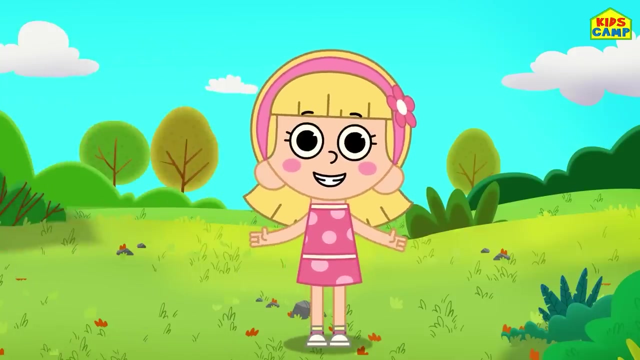 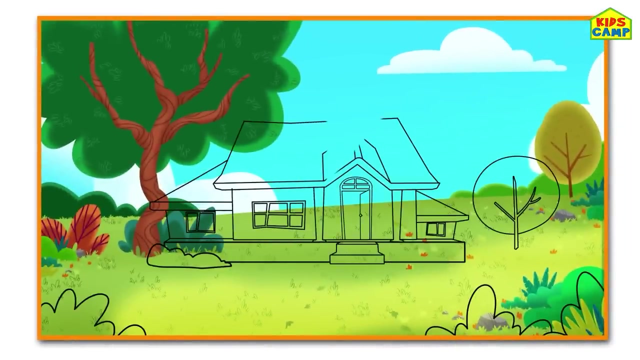 Yay, Come back for more games And keep watching Kids Cam. Until then, bye, bye, Hi friends, I am Elly And today we are going to Build a house. Excited So am I. Let's go. Oh, that's the outline. Let's fit the different Parts of the house. 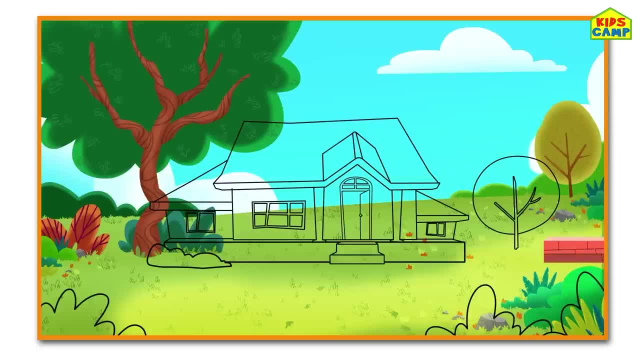 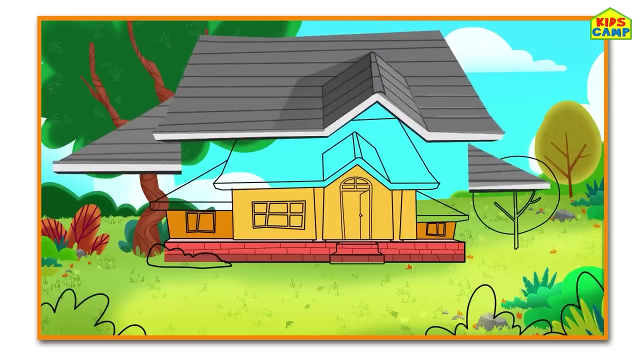 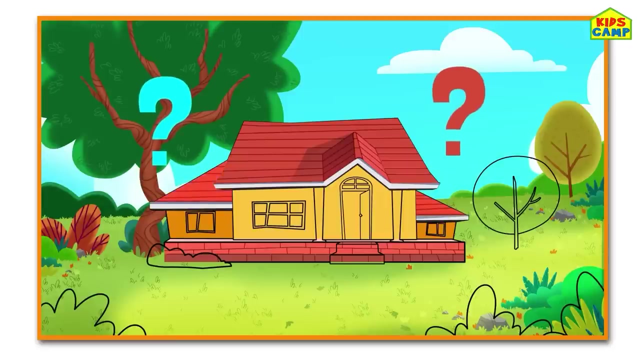 Right there, Let's figure out what goes where. First, the foundation, The base. Oh, that was easy. Now let's add the walls. I love yellow paint on my walls. This looks great. Next, let's Add the roof. Perfect, It's starting to look Like a house. What's missing? 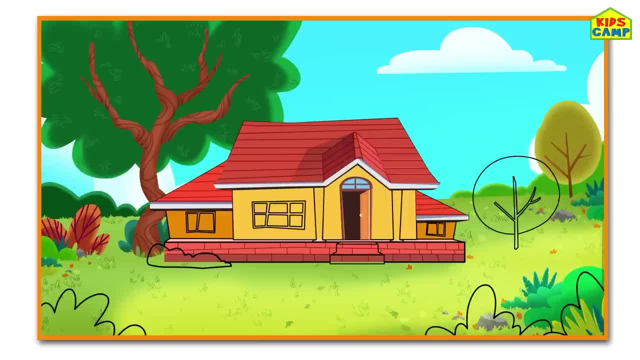 That's right. a door, Yes, And Lovely windows To look outside And for sunshine to come in. Next we need Steps- Perfect, And now Let's add the pillars. Going good, This is such a beautiful house, But what else is missing? Let's add color to my garden, Wow. 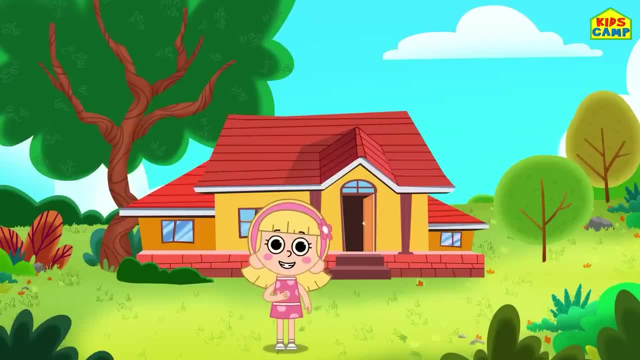 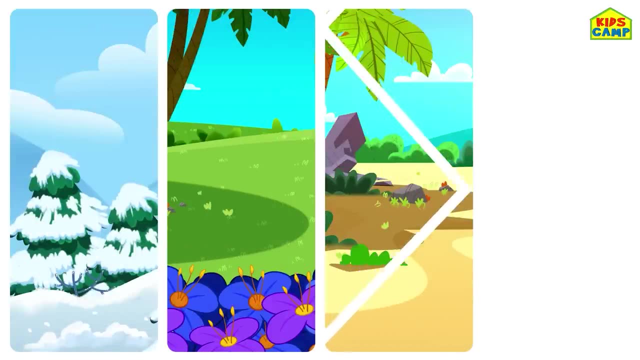 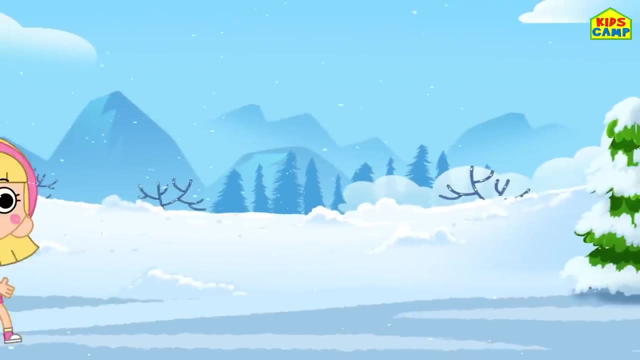 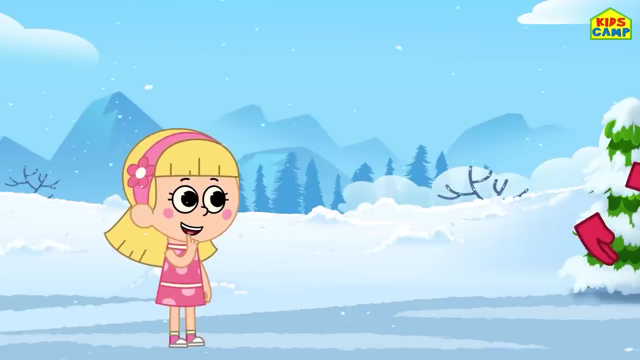 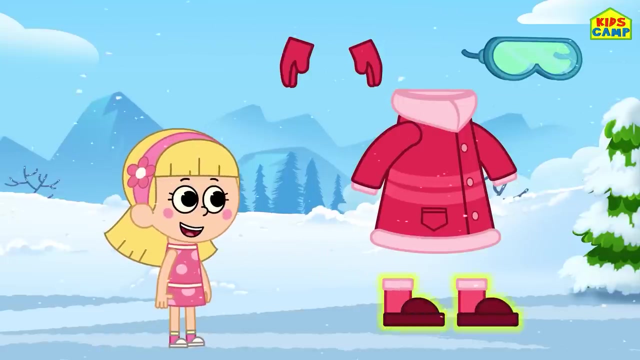 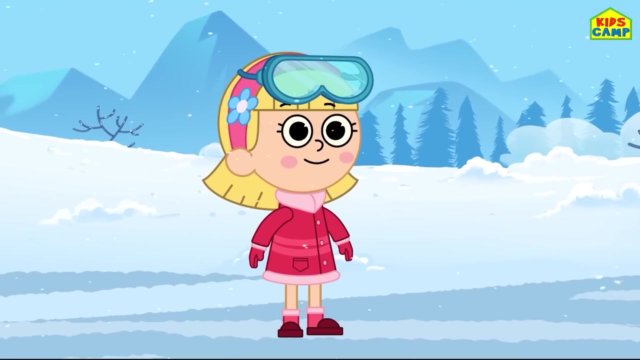 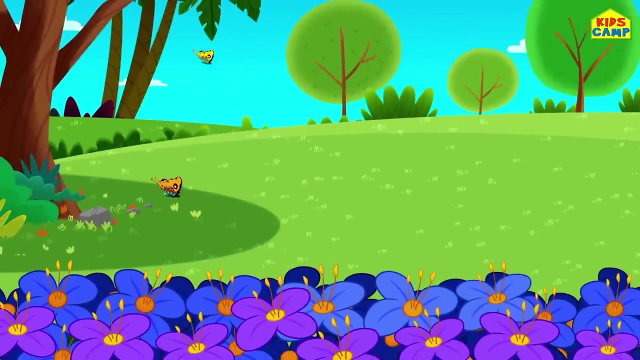 It looks beautiful. Ok, friends, I am going home. See you, Bye Seasons with Elly. What season is this? Winter Gloves, No, goggles, Coat, Boots, Yay, Woohoo, What season is this? It's spring. Flower headband, Flower headband, Flower headband. Wow, Look at the flowers bloom. 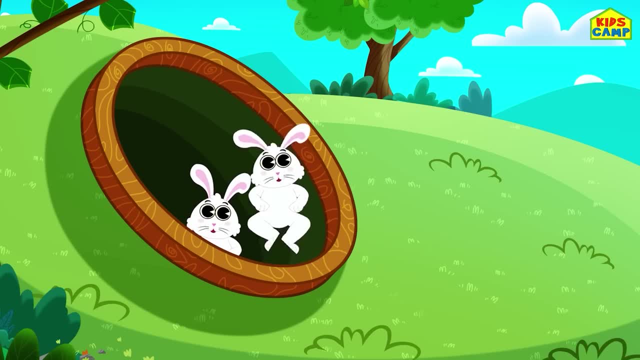 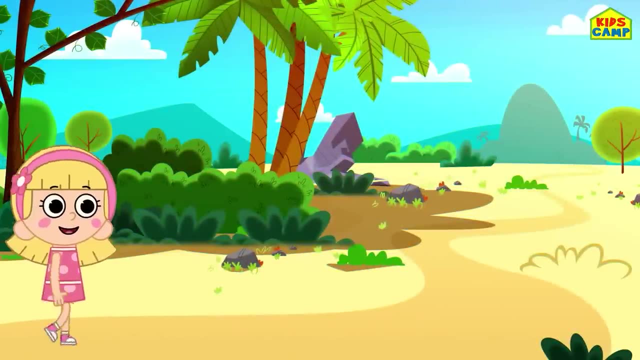 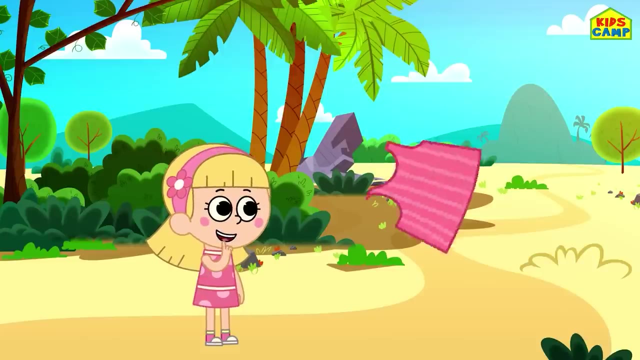 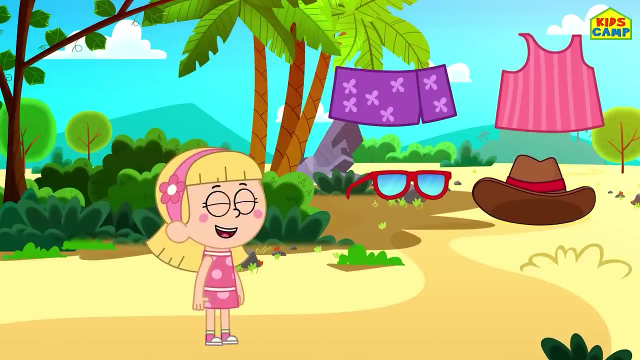 Look at: the flowers bloom And the birds sing, The bunnies have come out to play And the sun is shining bright. And the sun is shining bright. What season is this? It's summer. It's summer- Swimsuit, Sarong, Sunglasses, Hat, Yay. 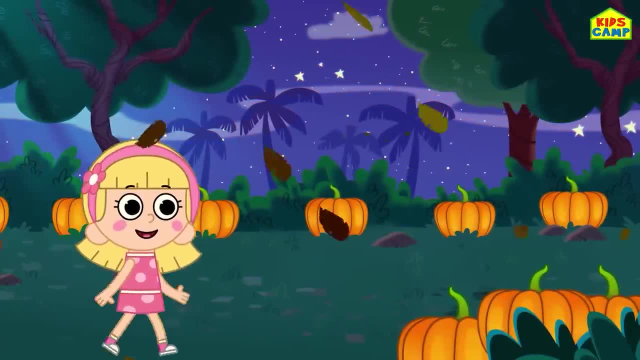 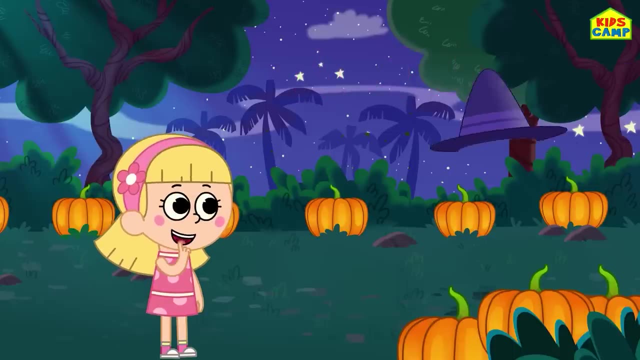 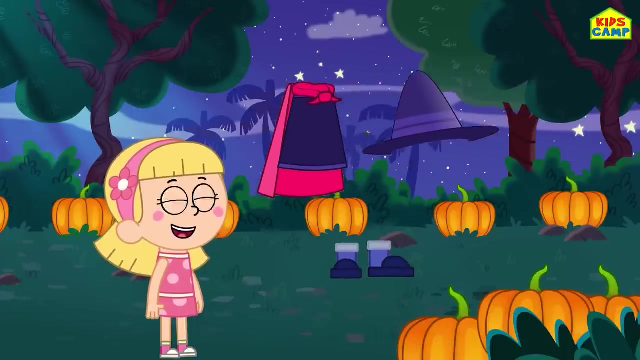 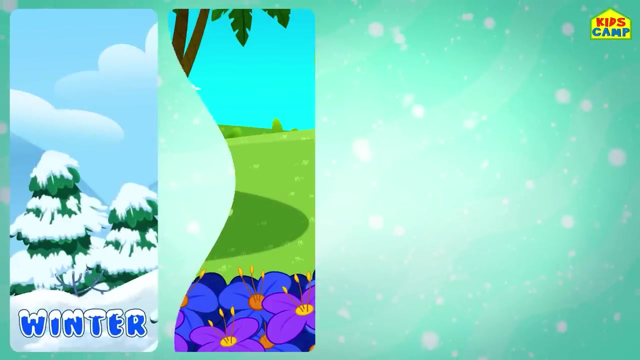 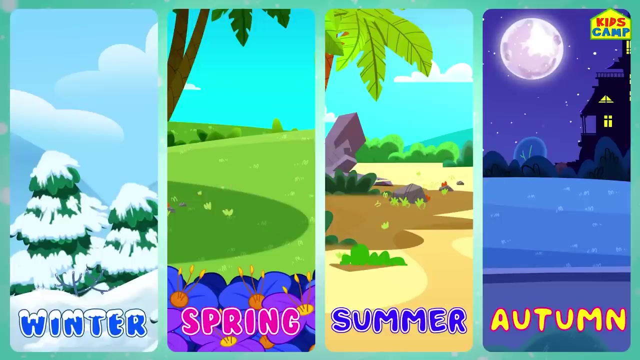 We are ready to go to the beach. Oooh, It's nearly Halloween. That means it's Autumn. A witch's hat, A dress with a cloak And witch's shoes- Yay, I am a witch. Today we learned our seasons: Winter, Spring, Summer And Autumn. Woohoo. 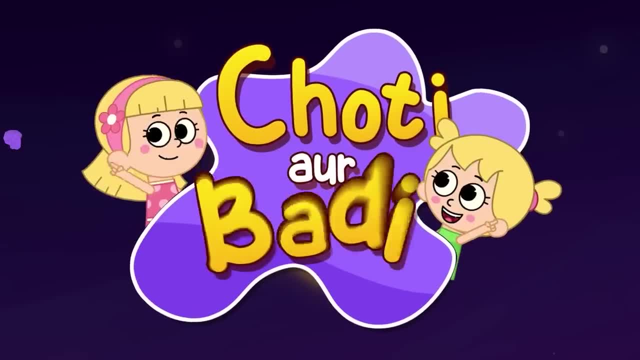 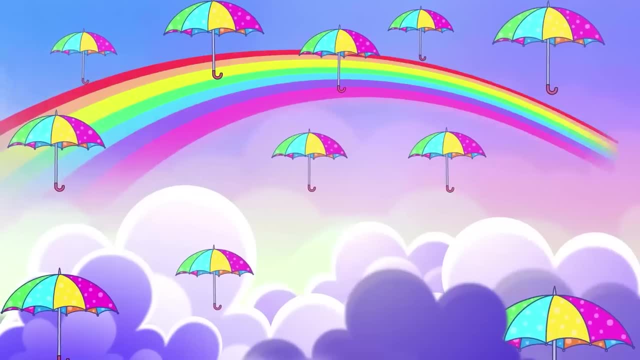 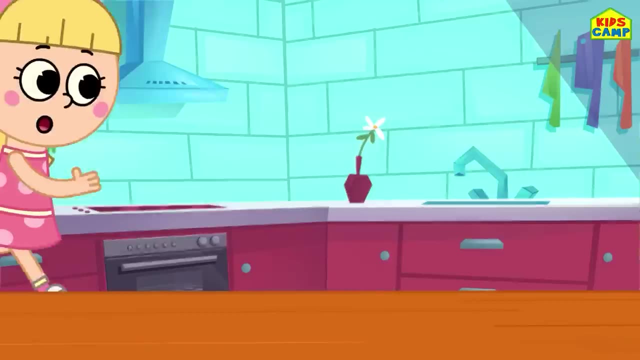 Coming soon is Parish Aayi By Choti Aur Bari. Parish aayi, Parish aayi Cham cham, cham Lekar chhata saith nikli, Hum, hum, hum, Hum, hum. Hi friends, I'm Ellie And I love jelly beans, Don't you too? 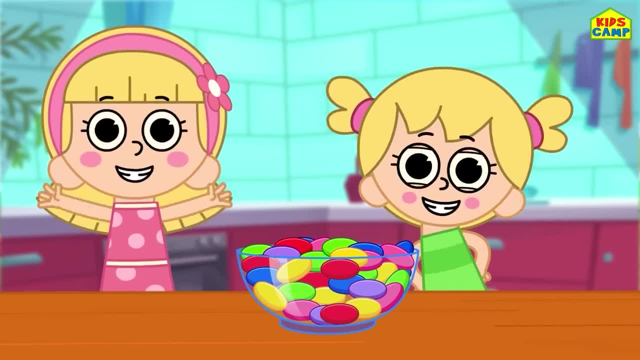 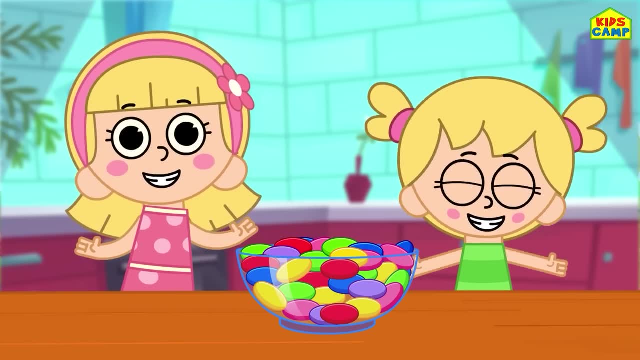 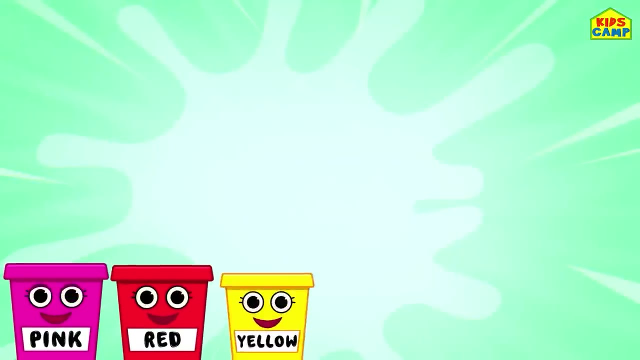 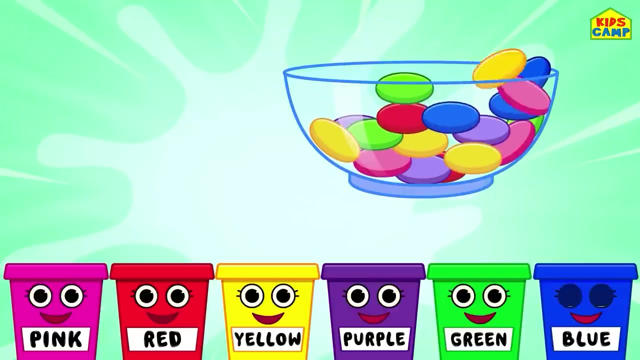 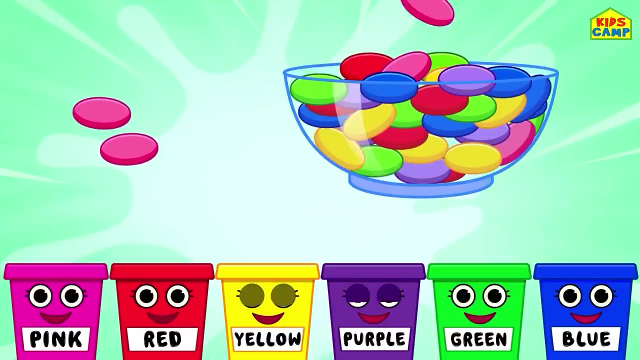 That's right, And this is Eva. We have to sort the jelly beans By their color. That's easy. Yay, Will you help us? Let's get started. Let's get started. Ooh Jelly beans, Ooh Jelly beans. Ooh Jelly beans. Let's sort the pink jelly beans. 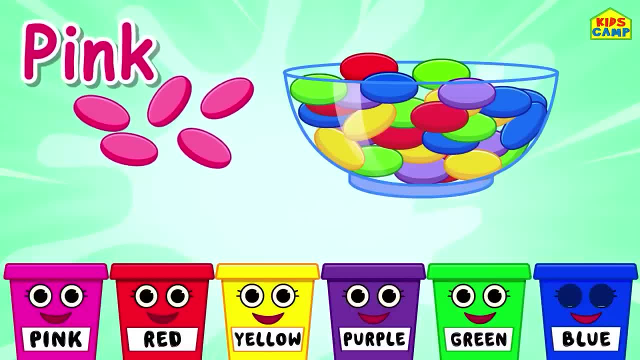 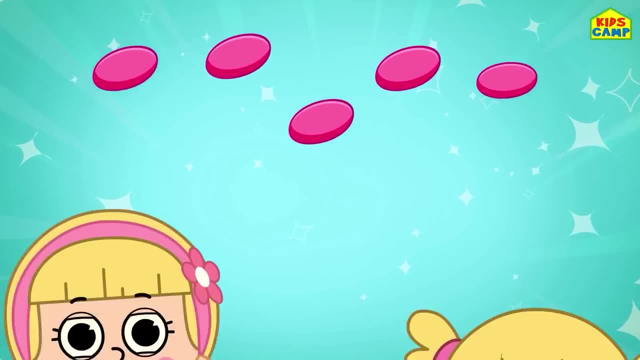 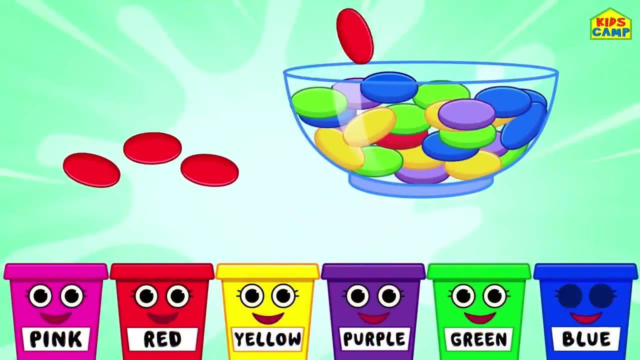 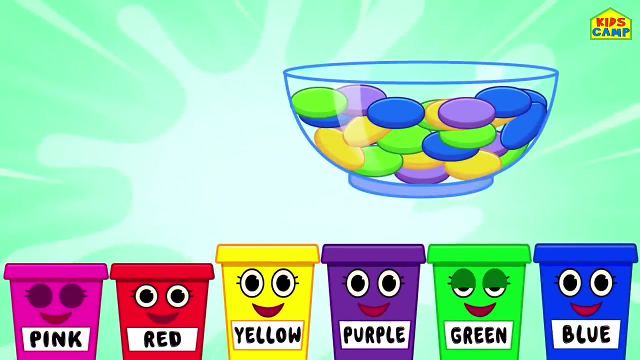 Let's sort the pink jelly beans- Yummy, Into the pink bucket. Into the pink bucket. Wonderful, Yay. Next up is Red. Let's sort the red jelly beans- Woohoo, Into the bucket, Yummy. Next up is the color yellow. Yummy, Let's sort all the yellow jelly beans. 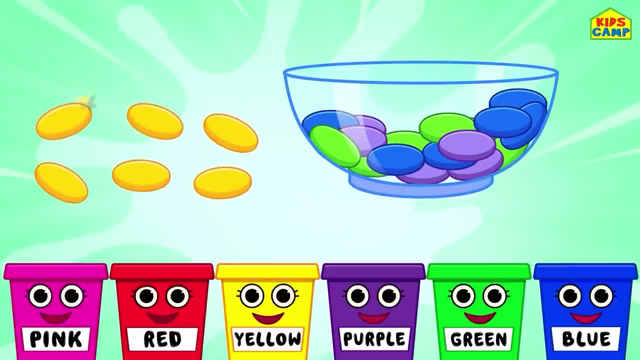 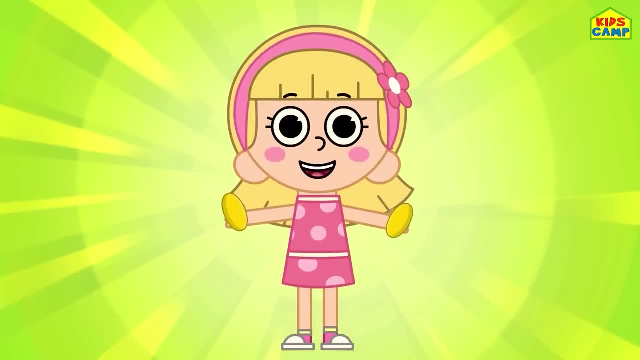 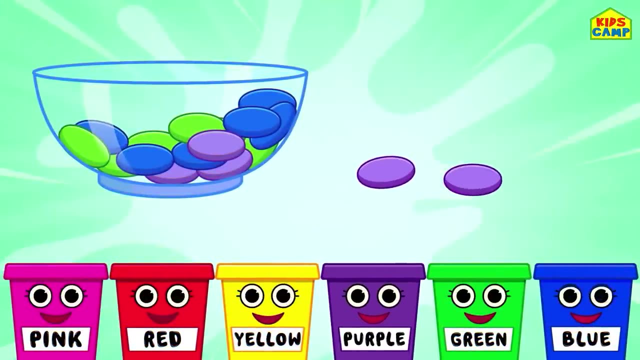 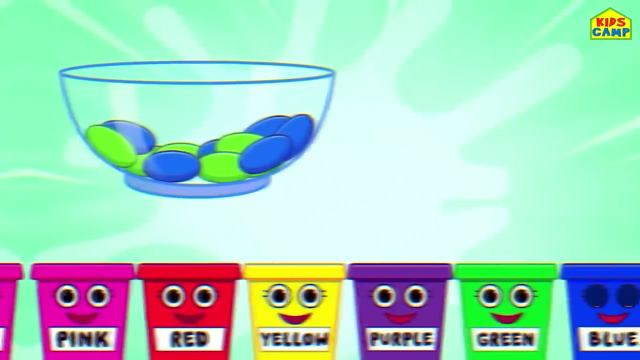 That's right Into the bucket. Wonderful, I love yellow. Next is purple. Look for all the purple jelly beans. Yes, That's right Into the bucket. Great job, friends. Wonderful. We all love jelly beans, don't we? 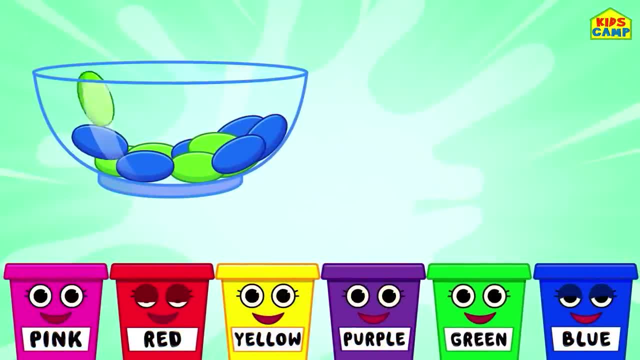 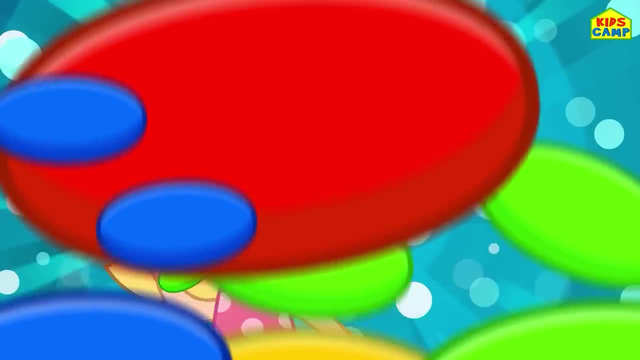 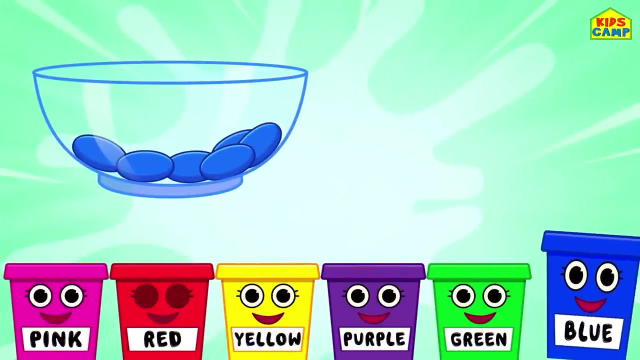 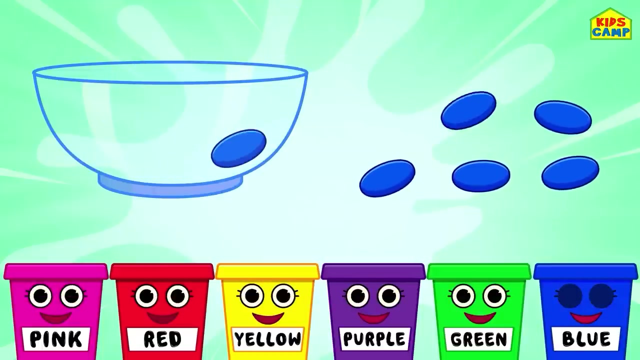 Next is green. Let's sort all the green jelly beans Yummy Into the bucket. Wonderful Yummy. And the last one is blue. That's right, We have only the blue jelly beans remaining. That's right Into the blue bucket. 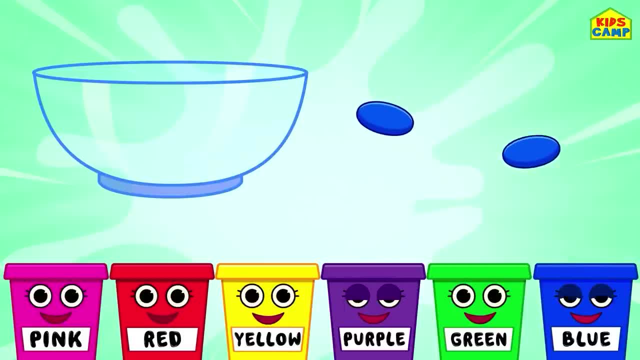 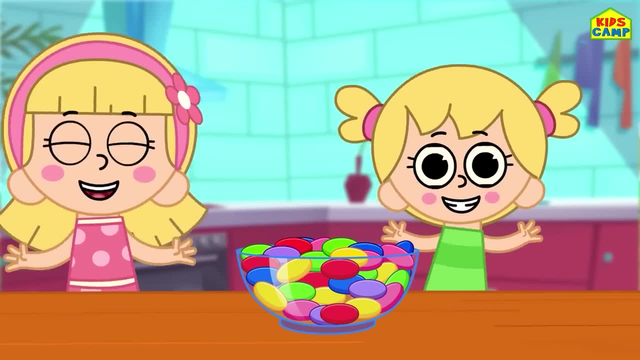 And we're done. Good job, friends. That was such a fun time sorting the jelly beans. Come back for more on Kids' Game. See you soon. Bye-bye, Hi everyone, What a beautiful day. I'm Ellie. 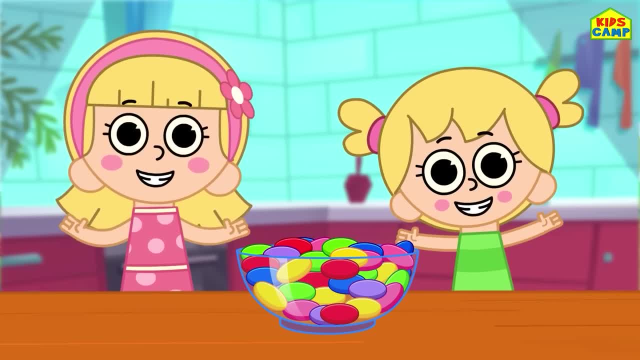 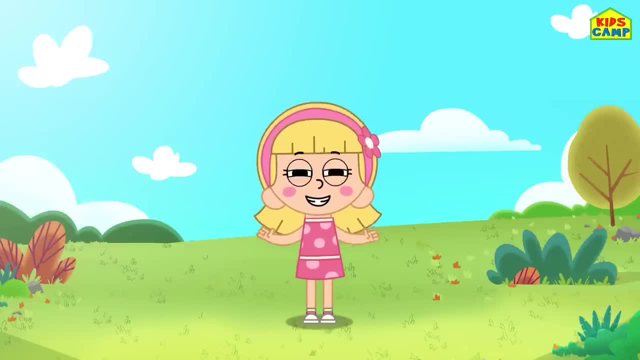 And we are going to play a new game called Fun with Ellie. And we are going to play a new game called Fun with Ellie. And we are going to play a new game called Fun with Ellie. And we are going to play a new game called. 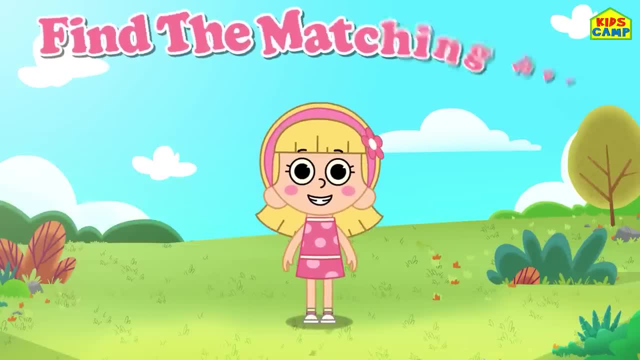 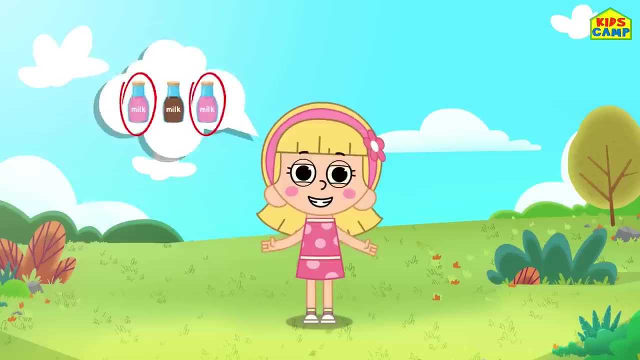 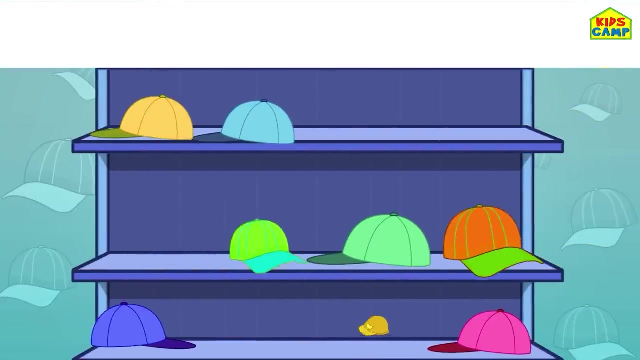 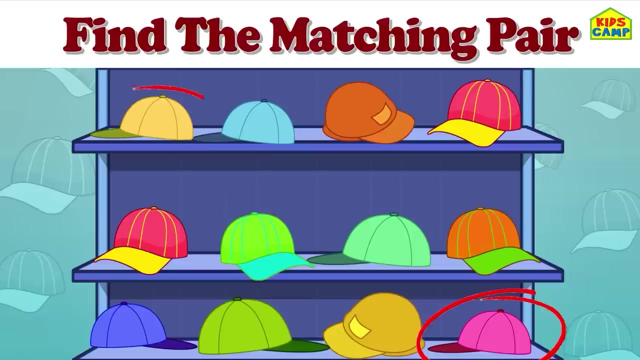 Find the Matching Pair. That's right. We have to find two similar objects, And that's the game. That's simple, Ready, Let's get started. Find the matching pair. Can you spot two identical caps? No, they're not identical. 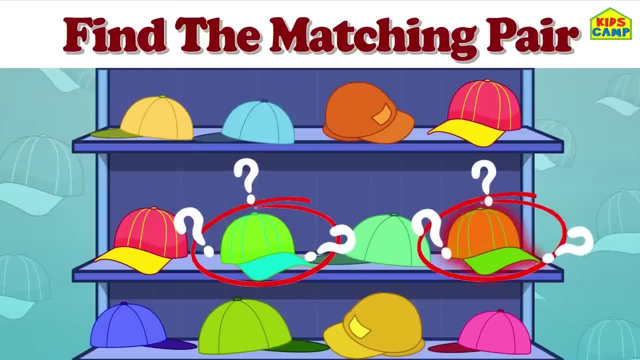 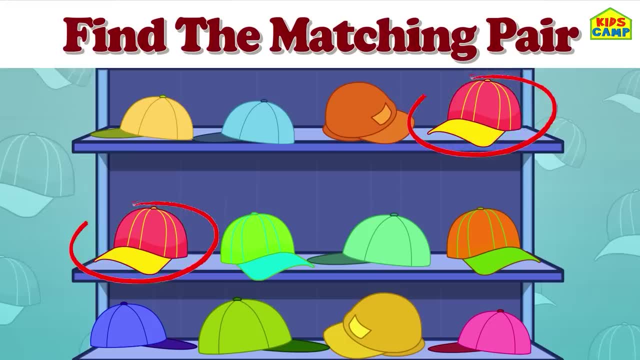 No, Yes, Yay, We found them. They are two identical cups. Good job, Let's find another pair. Find the matching rockets, Can you? No, Not this one. No, Not this one. No, Not this one. 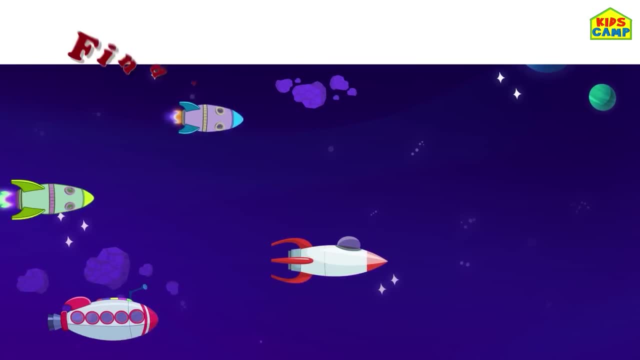 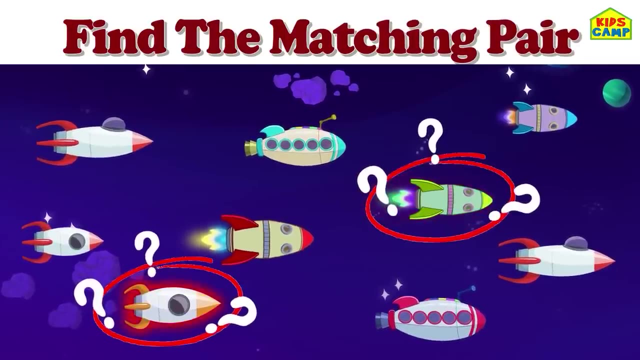 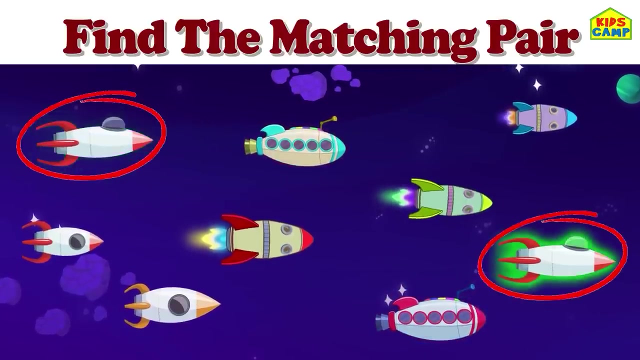 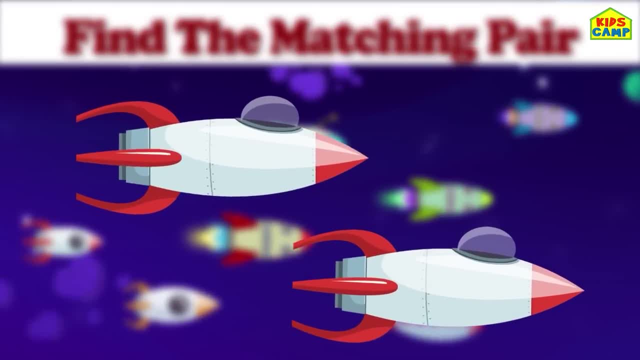 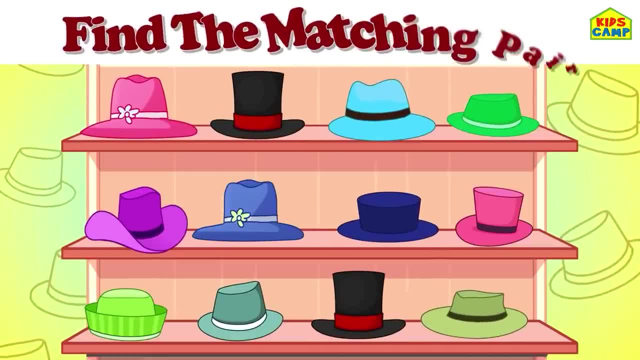 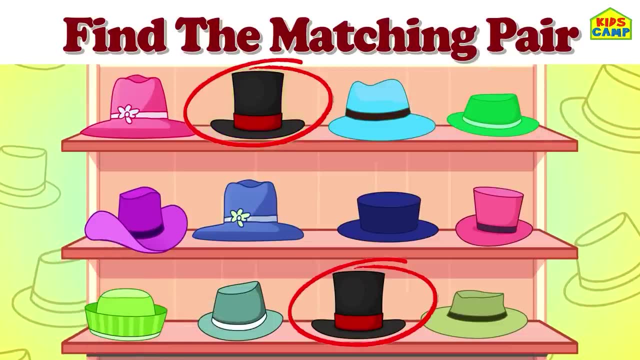 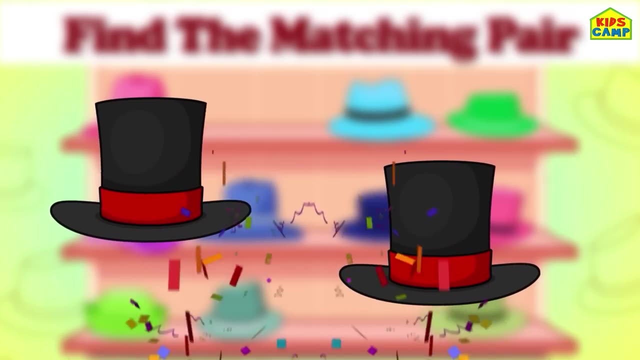 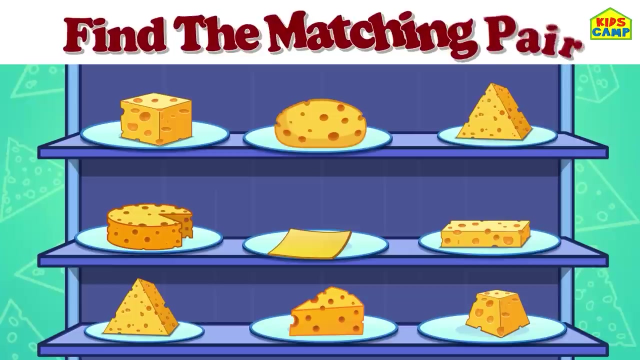 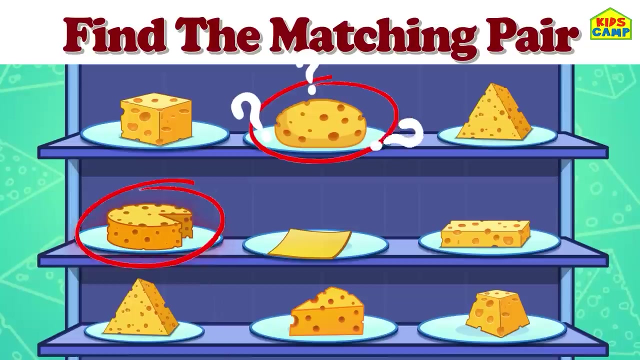 No, No, Not this one. No, Not this one. No, Yes, They match Perfect. We found them, Yes, We found them. Perfect pair. Good job, friends. Can you find the matching cheese? No, Definitely no. 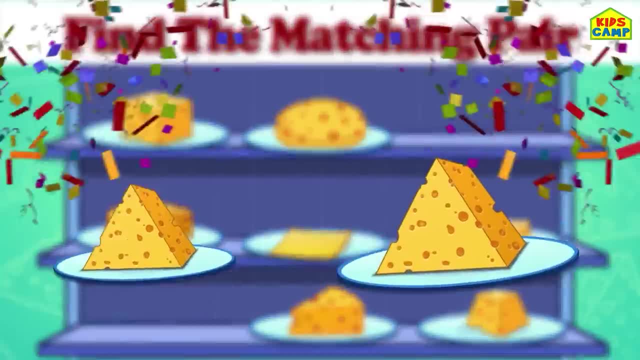 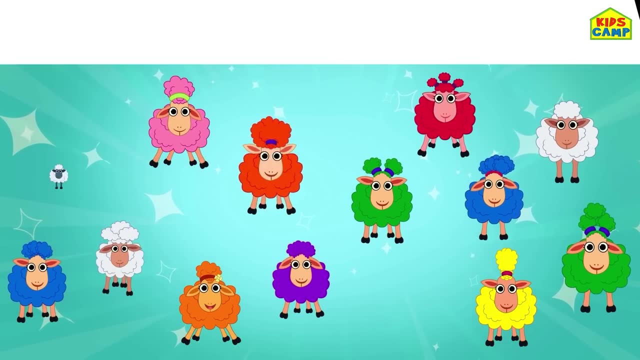 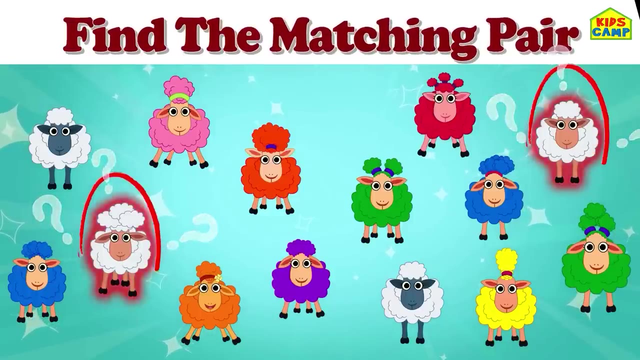 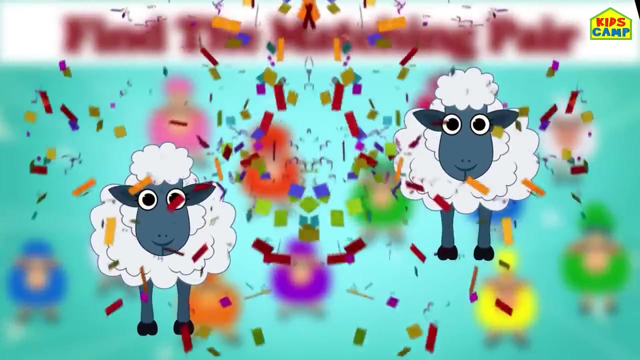 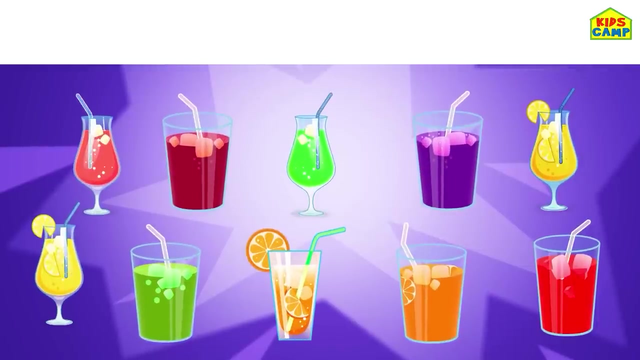 That's right. These match Perfect. Good job. Can you find the matching pair here? No, They are not identical. Yes, They match. That's right. These sheep match Perfect Perfect. Find the matching coolers. Do these match? 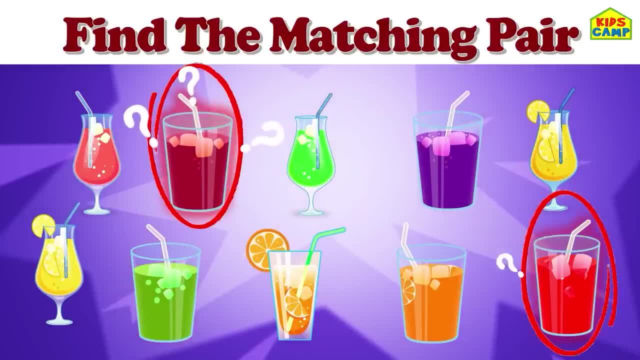 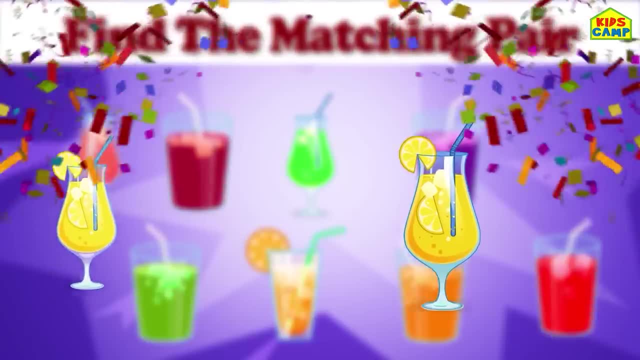 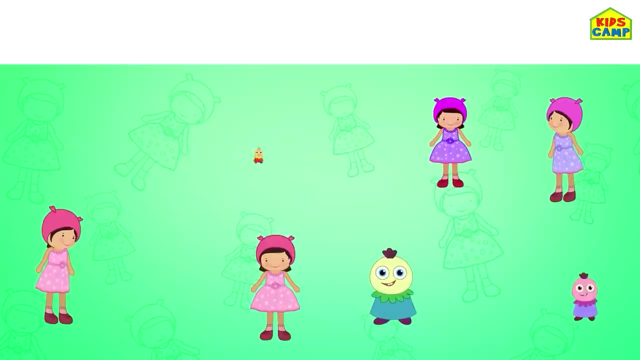 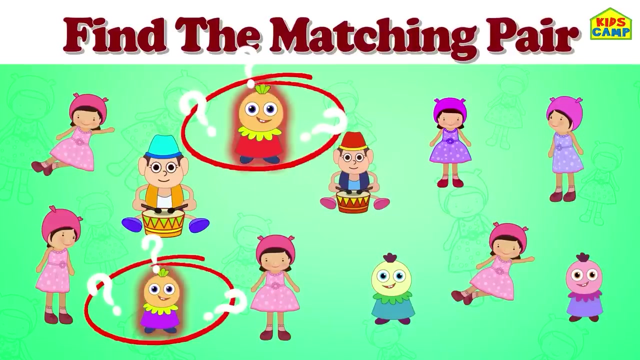 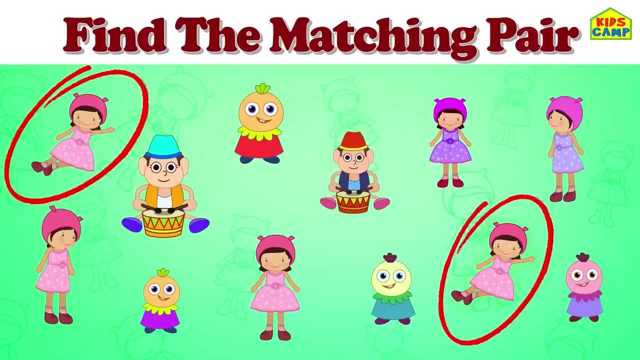 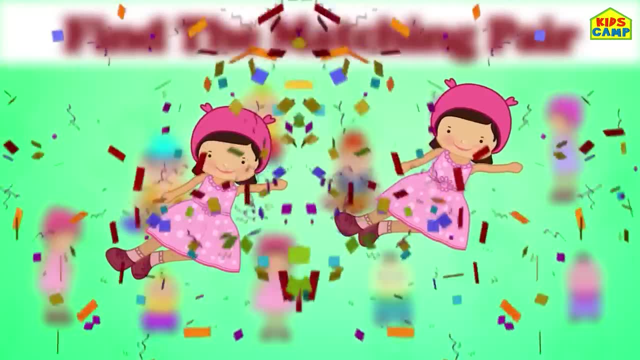 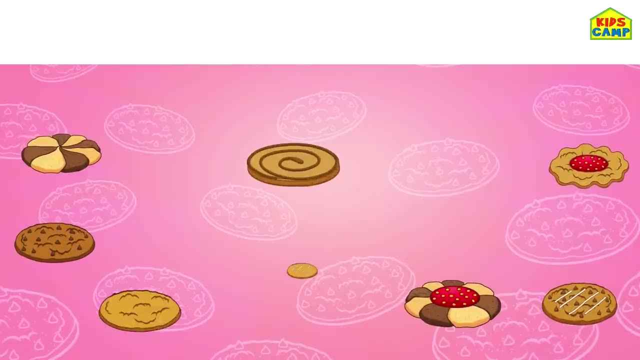 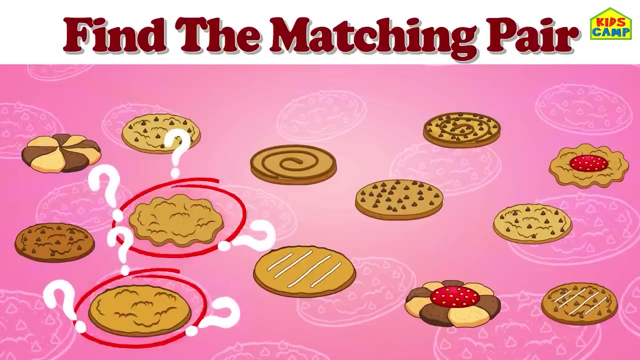 No, No, No, No, No, No way, That's right, We found the pair. Yay, Good job, friends. This game is so much fun. Oh, Cookies, Find the matching pair. No way, Yes. 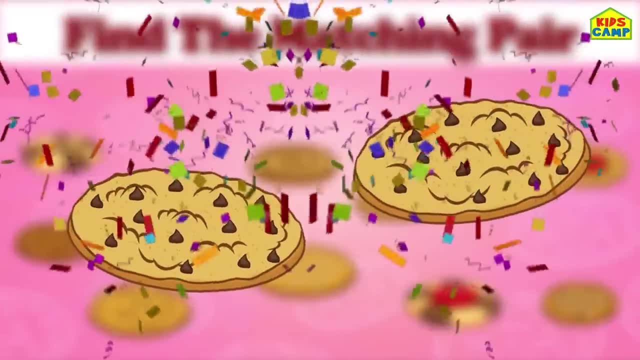 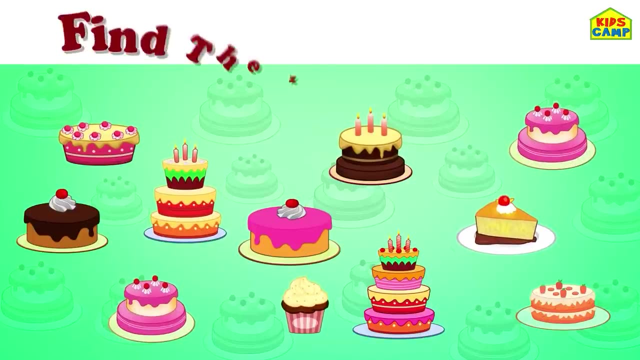 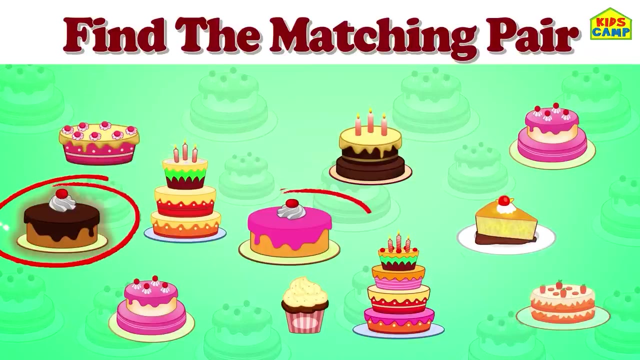 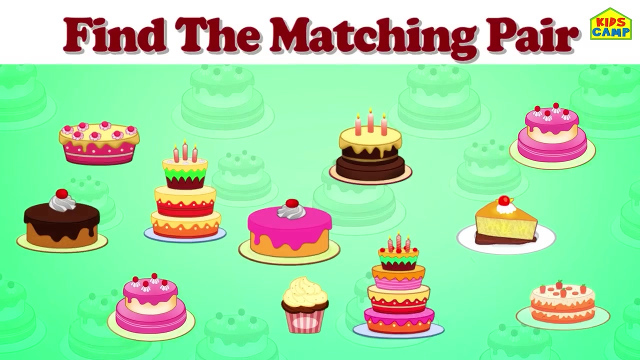 We found them. No, No, No, No. I love cookies, Yummy. Let's go to the next one, Hmm, cakes. Find the matching pair. No, No, Yes, That's right, The matching pair of cakes. 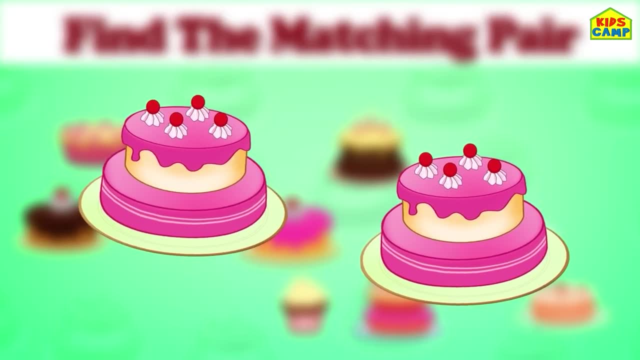 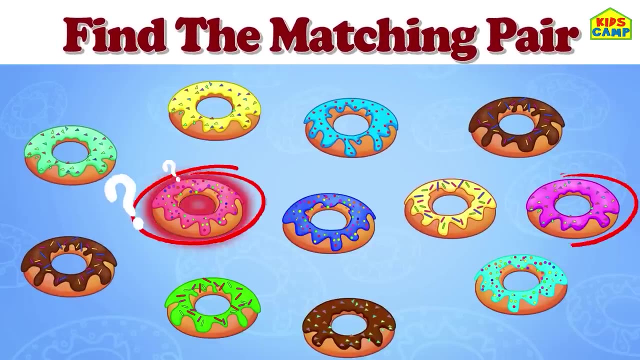 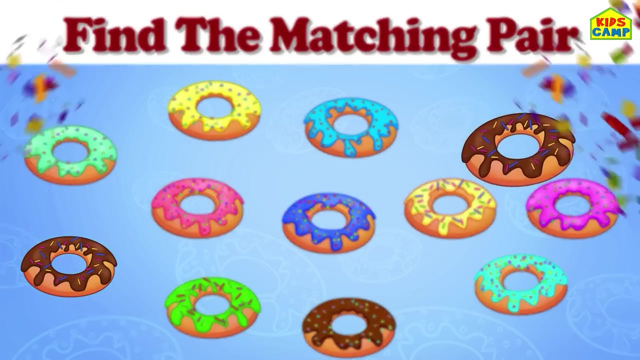 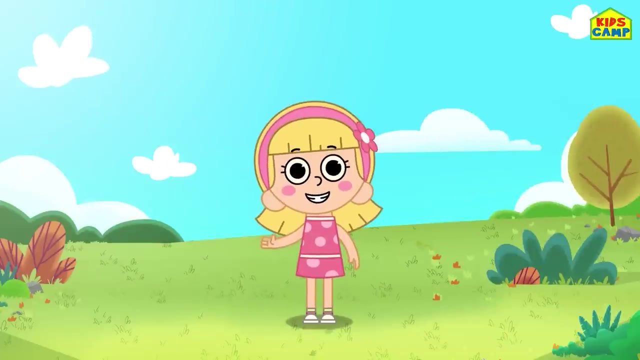 Yummy, Wonderful Ooh donuts. Find the matching pair. No, no, Yes, We found the matching pair. These match. This was such a fun game, friends. Keep watching Kids Camp. Bye-bye, Hi friends. 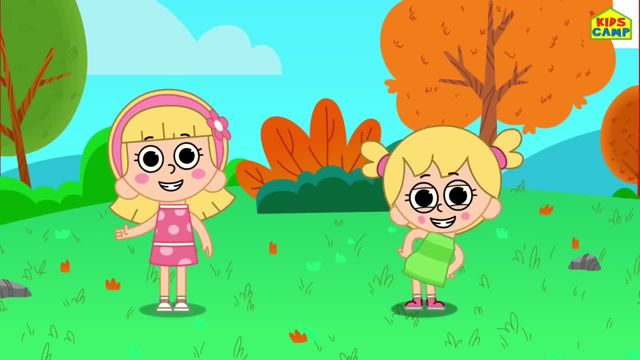 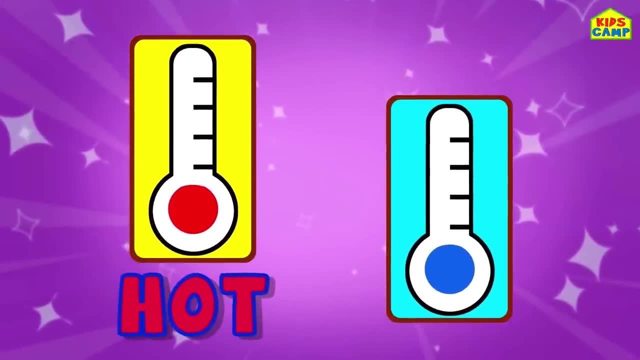 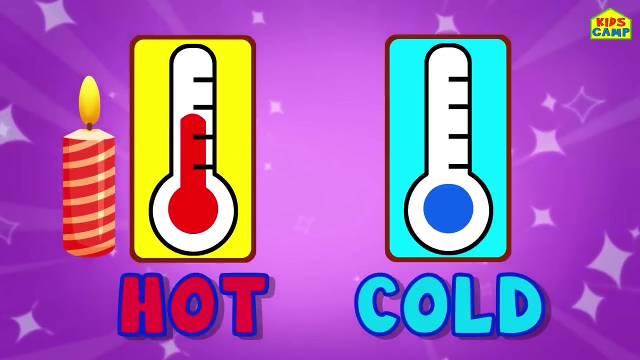 I'm Ellie and this is Eva. Today we're going to play a fun game of hot and cold. That's right. We have to sort according to what is hot and what is cold. For example, a candle is hot. That's right. 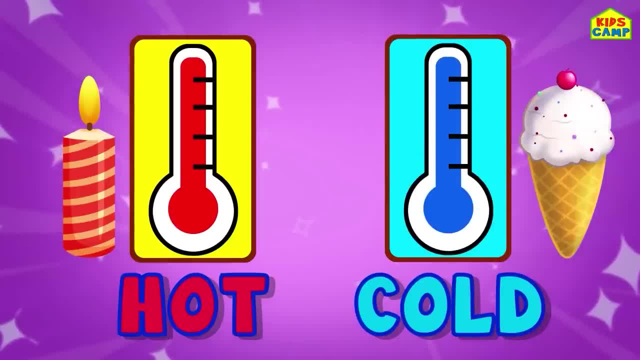 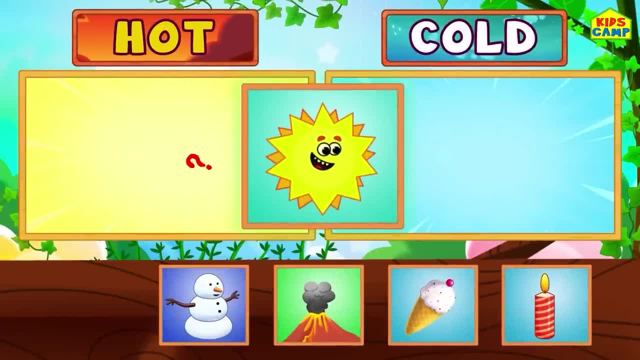 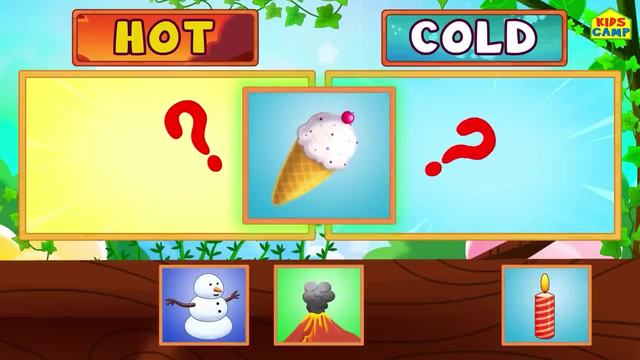 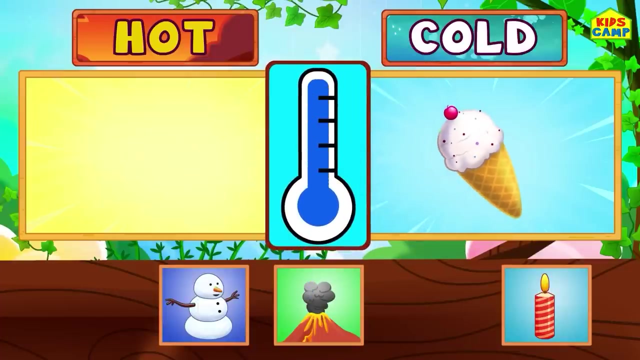 Let's get started. Hmm, Is sun hot or cold? That's right, Sun is hot, Very, very hot, That's right. An ice cream, It's Cold. Yummy, Yummy A candle. Hot or cold? 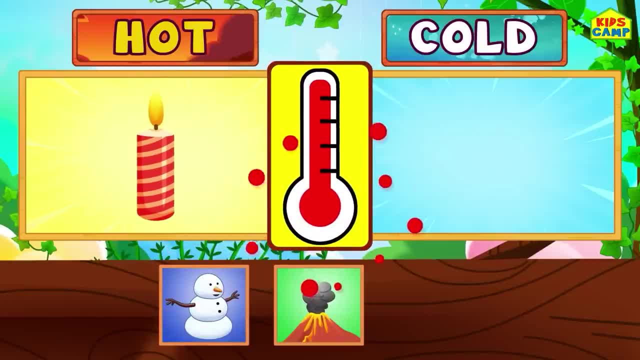 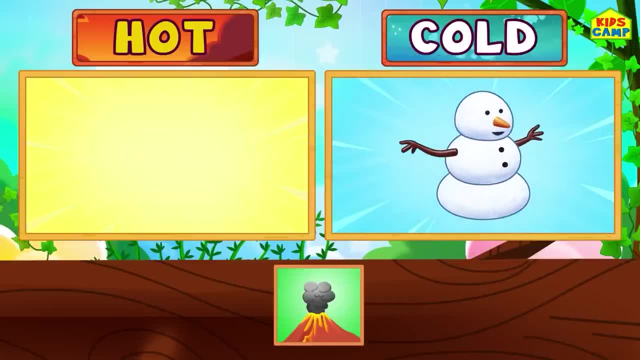 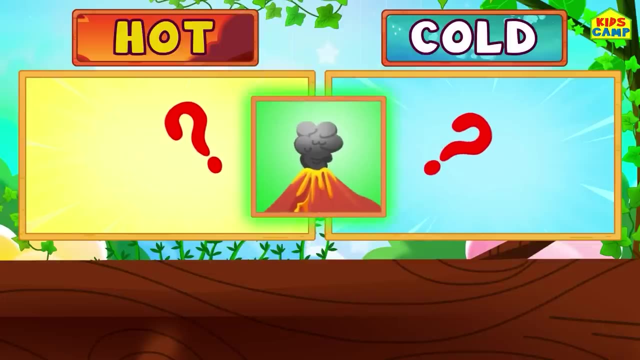 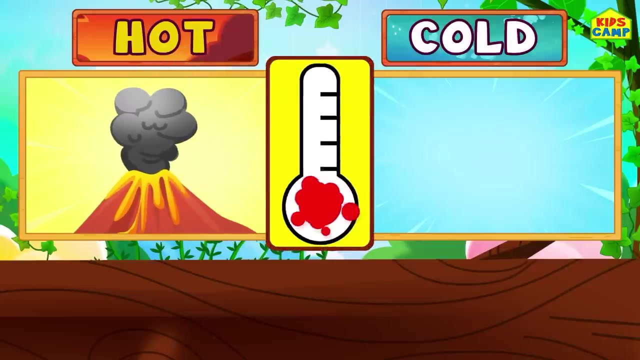 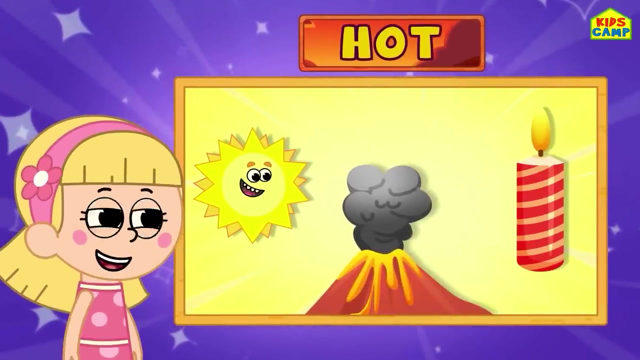 Hot, Good job, That's right. A snowman- Yes, Cold, That's right. A volcano- Hot or cold, It's Hot, That's right, Very hot. Yay, We found the hot objects: The sun. 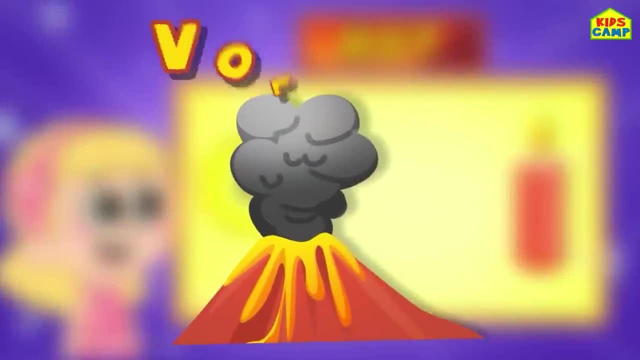 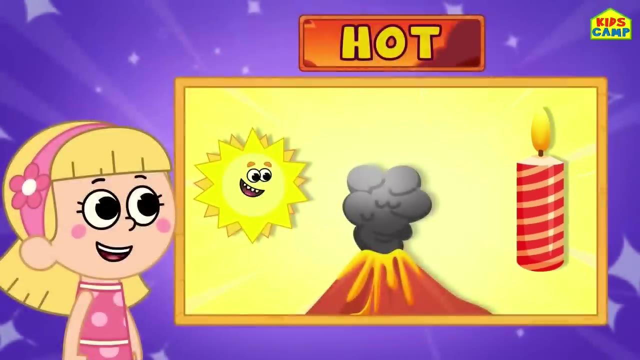 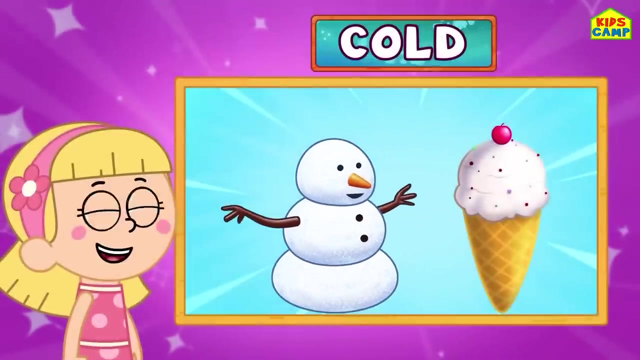 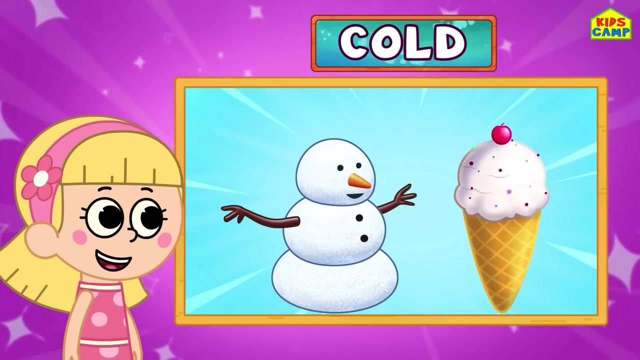 The volcano And the candle. And we found the snowman And the ice cream. All cold Yay. And we found the snowman And the ice cream. All cold Yay, All cold, Yay, All cold. 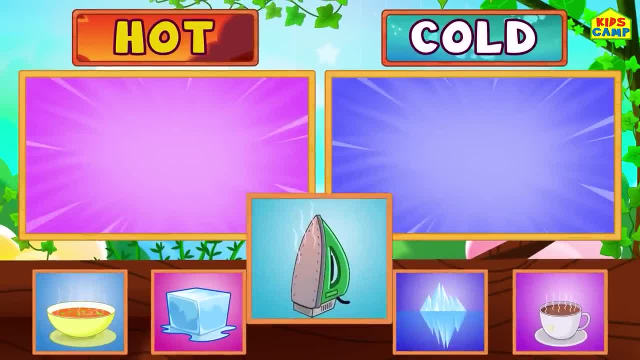 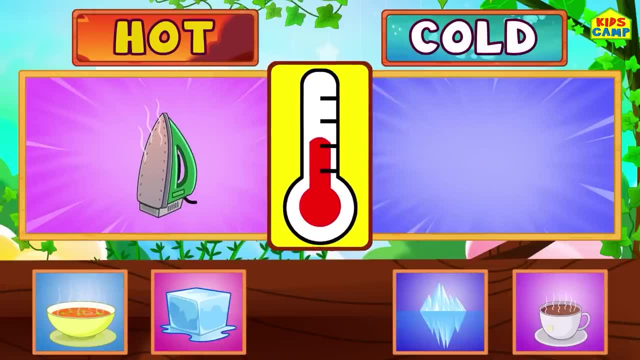 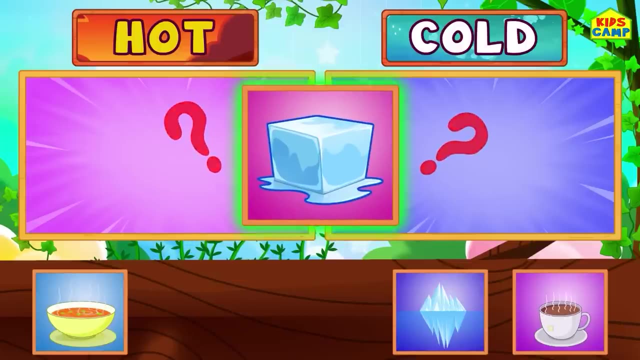 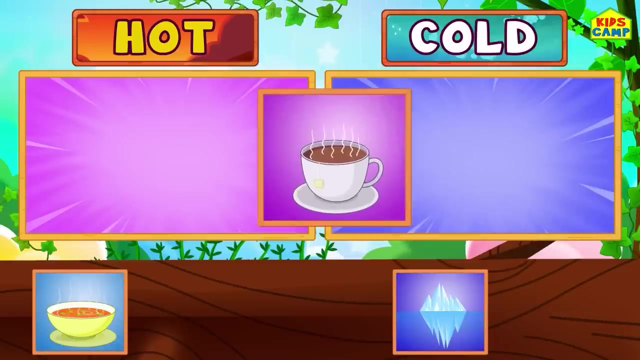 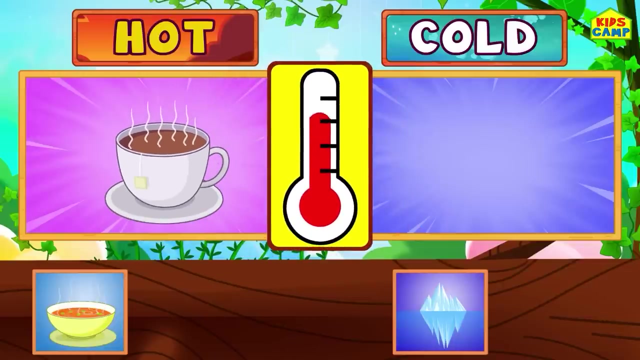 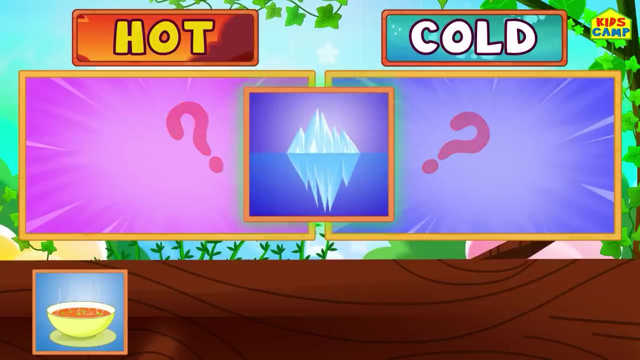 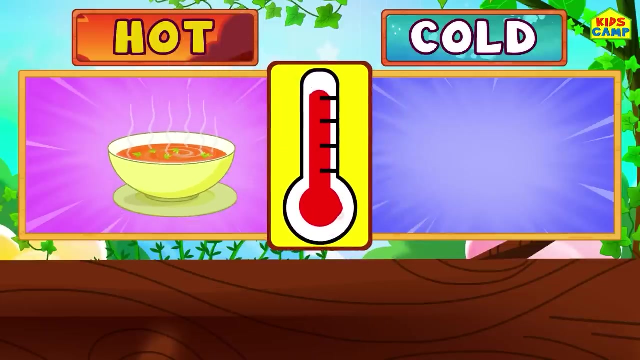 It's an ice cube. An ice cube, What's next? This is an easy game. An iron Hot or cold Hot, That's right, Hot. An ice cube, Hmm, Cold, Aaah, cold hot, that's right. an iceberg, its cold, good job. a bowl of soup? that's right, hot, wonderful. 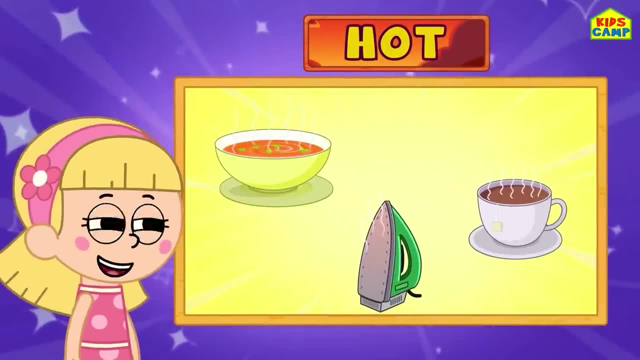 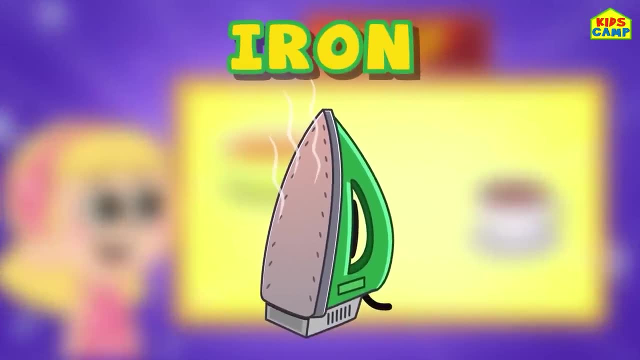 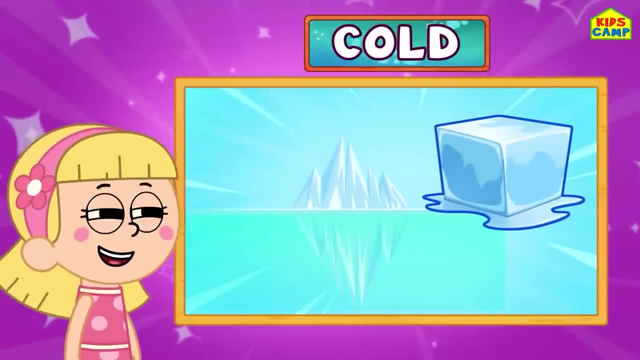 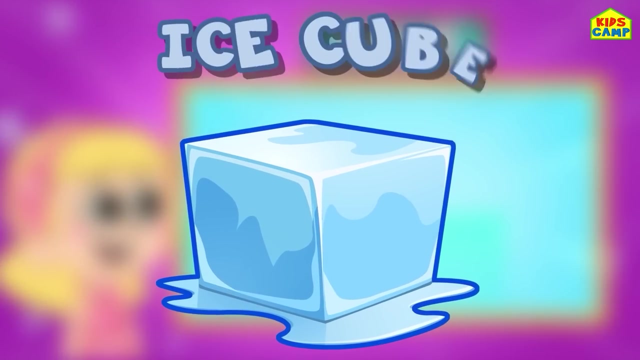 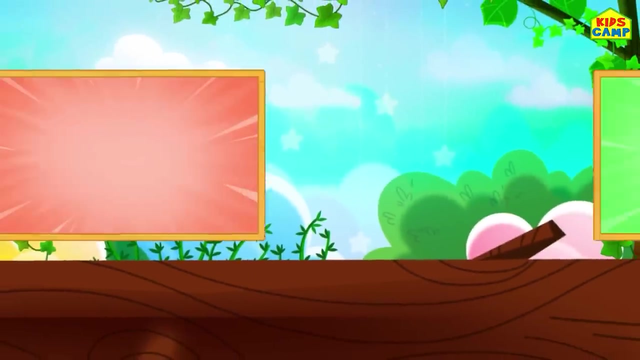 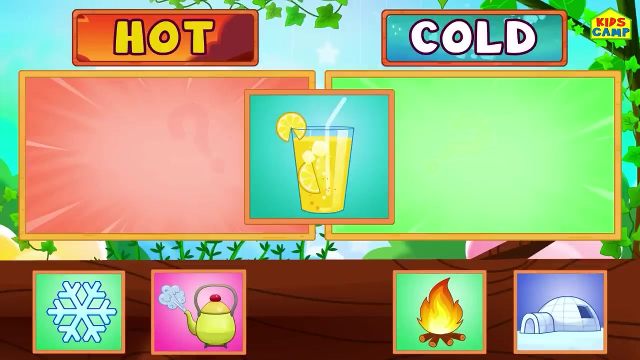 did we learn? a bowl of soup is hot and iron is hot, and the cup of coffee is hot as well, and iceberg is cold, and an ice cube is cold too. that's right. what's next getting good at this game? a lemonade. it's cold, definitely cold. 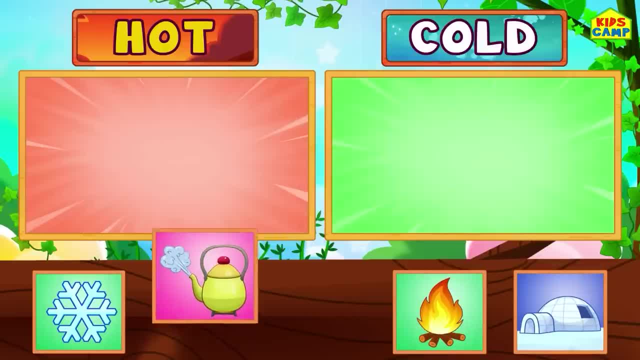 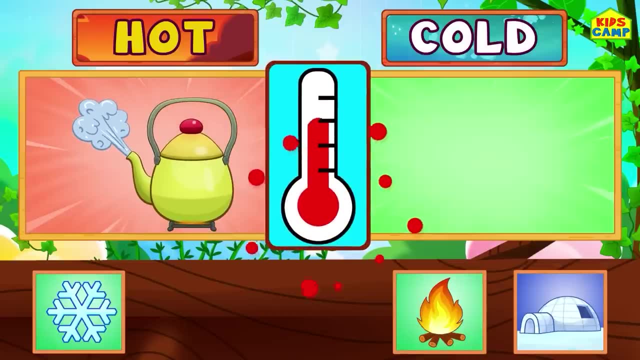 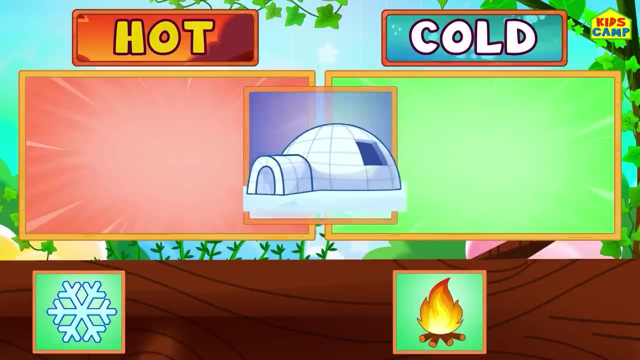 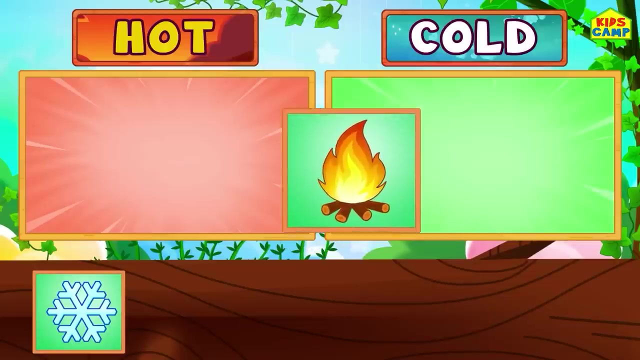 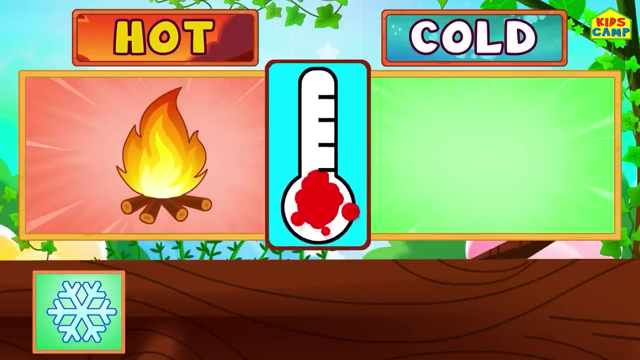 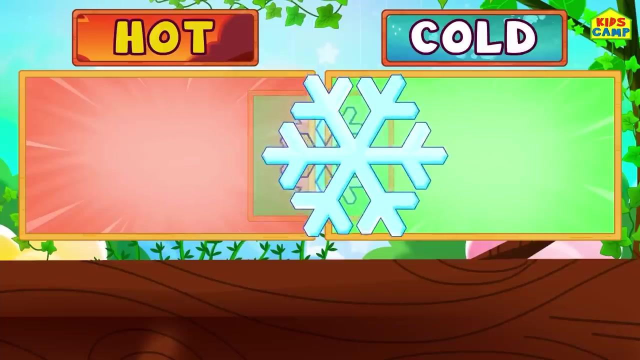 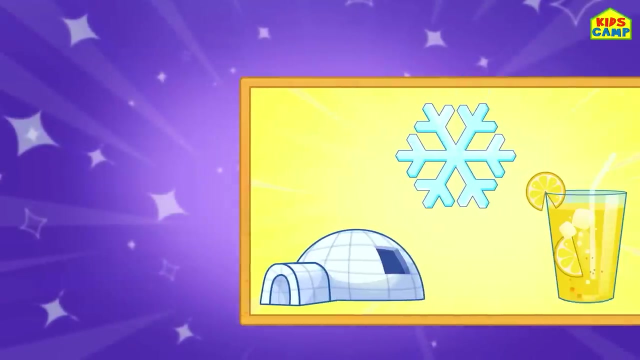 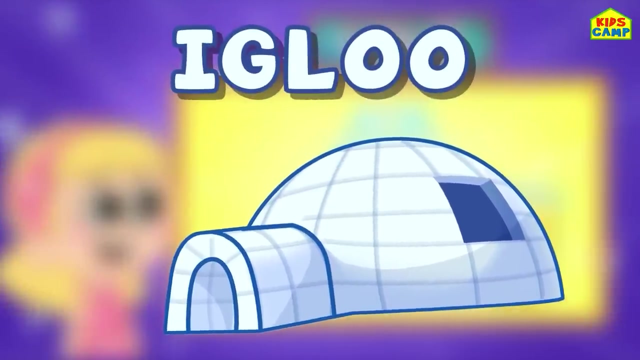 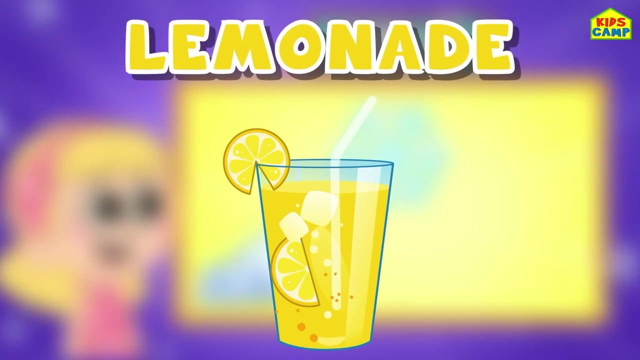 a kettle- it's hot, that's right, hot kettle. an igloo that's cold. fire, that's hot, definitely hot. good job, friends. and a snowflake that's cold. wonderful, what did we learn? an igloo is cold, a snowflake is cold and a glass of lemonade is definitely cold. 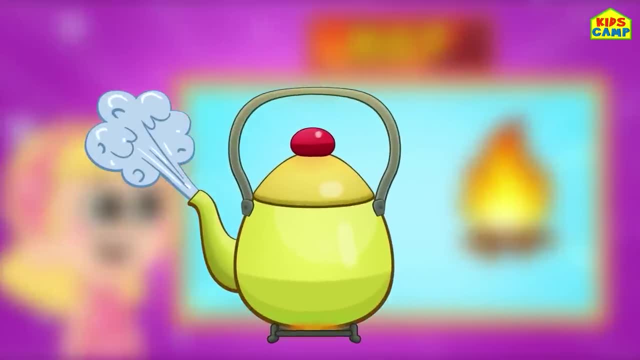 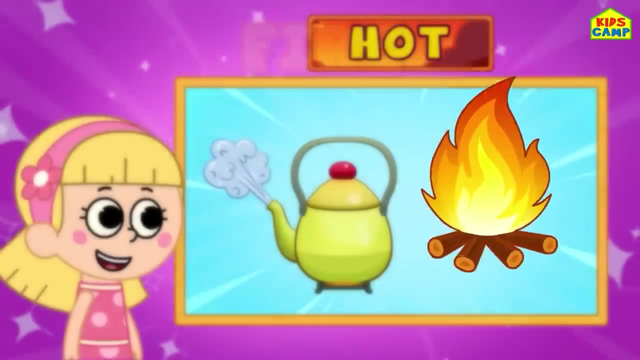 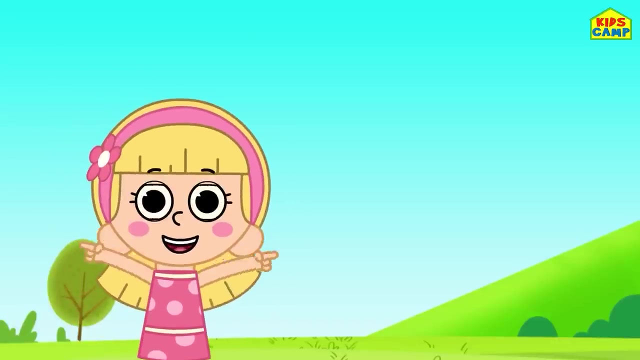 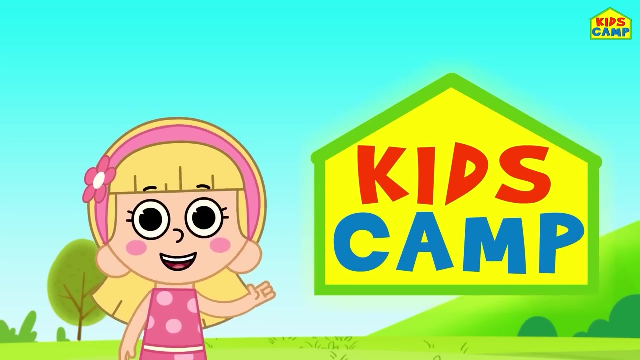 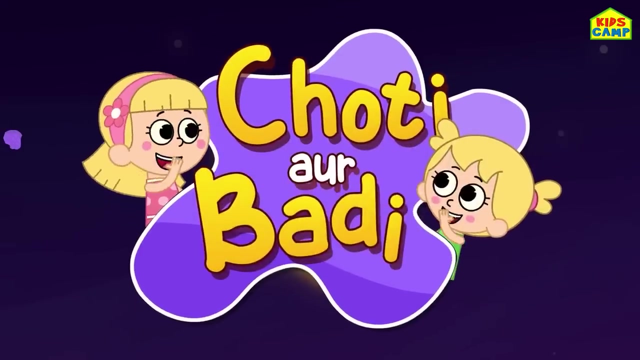 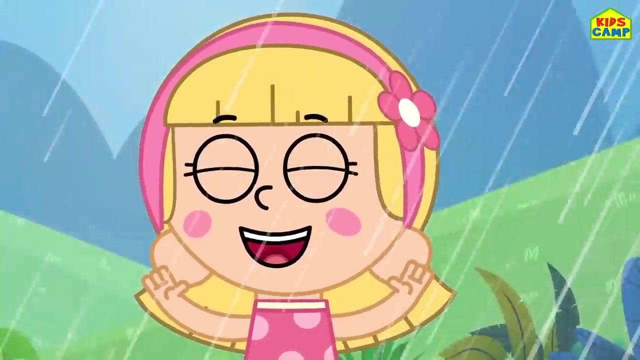 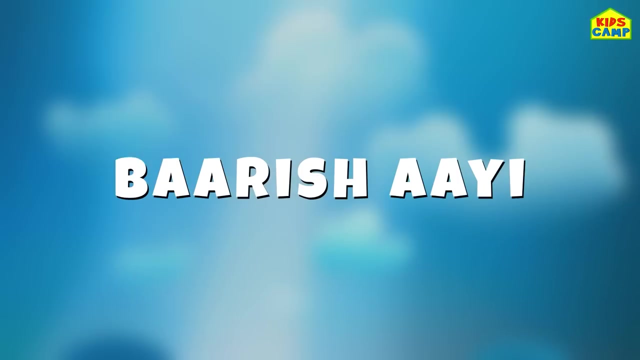 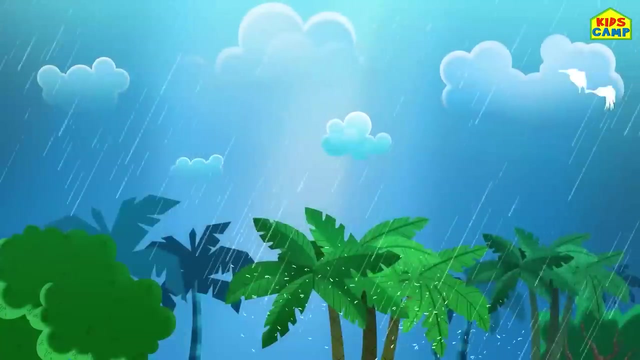 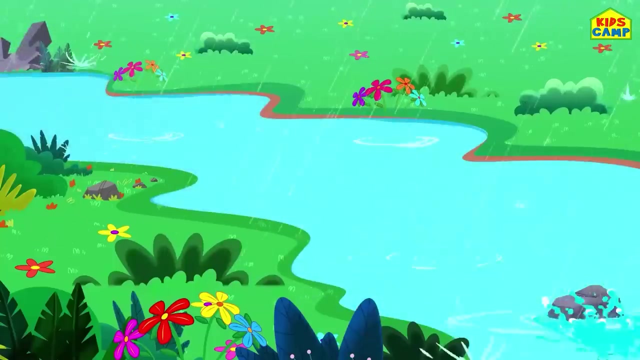 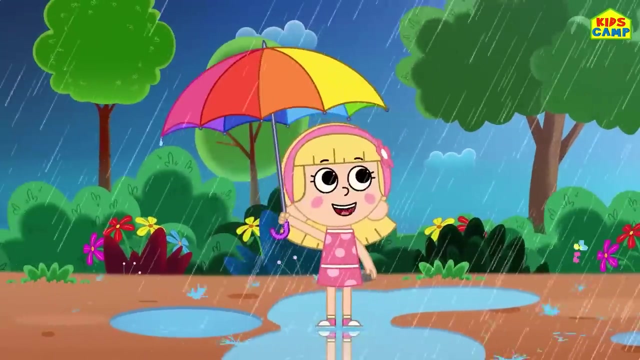 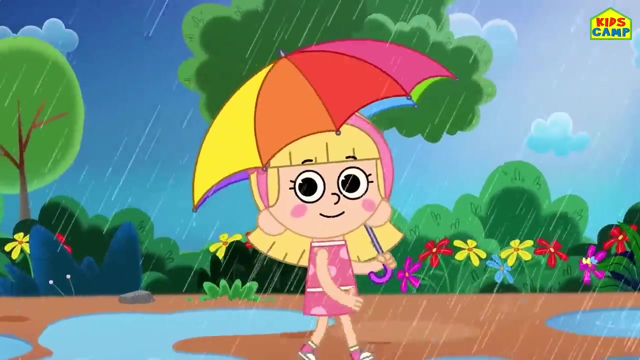 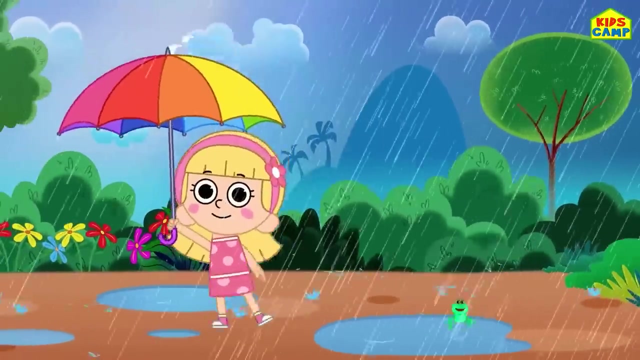 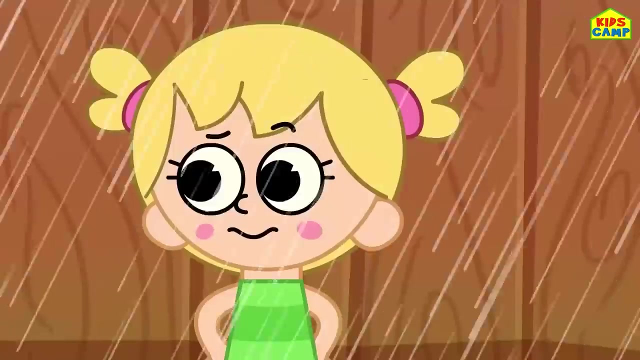 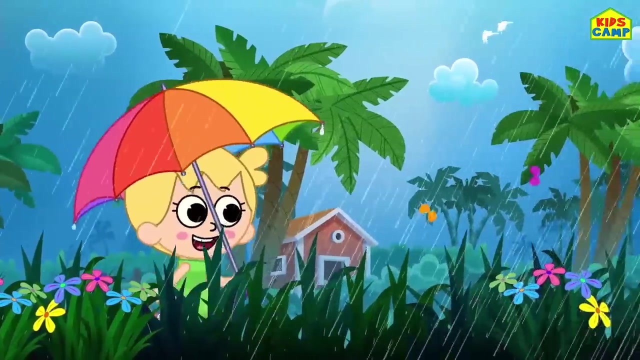 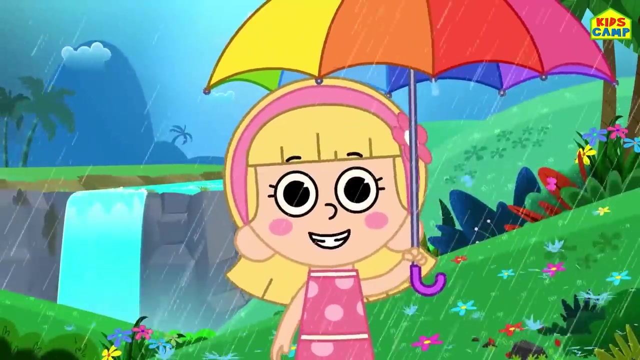 a kettle is hot and fire is hot. wonderful, yay, this is so much fun, much fun learning. Come back for more. Until then, keep watching Kids Camp. Bye, Bye, YouTube channel: Choti and Buddy. Bye YouTube channel- Choti and Buddy. 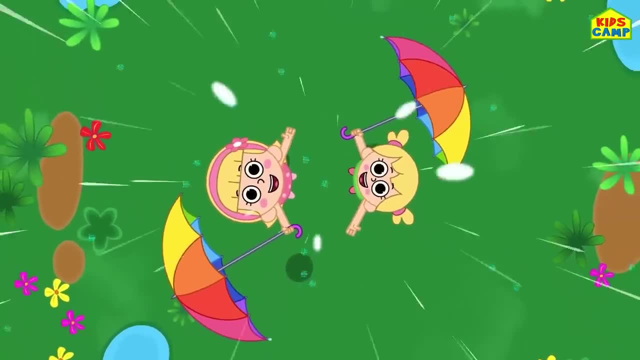 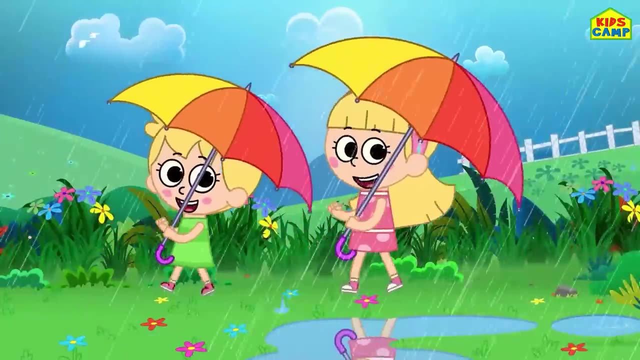 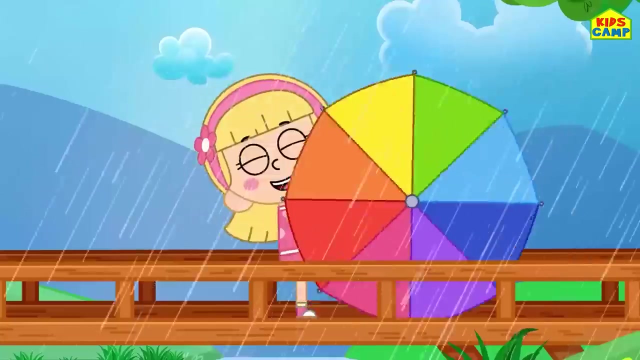 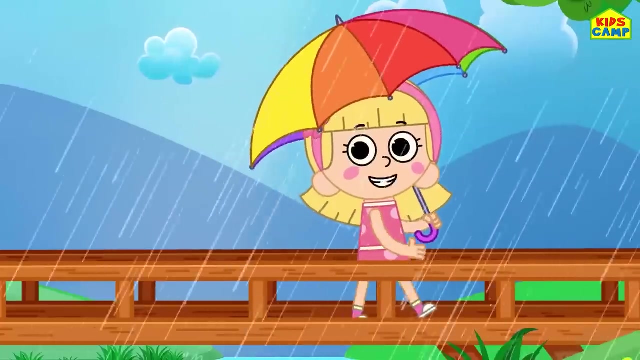 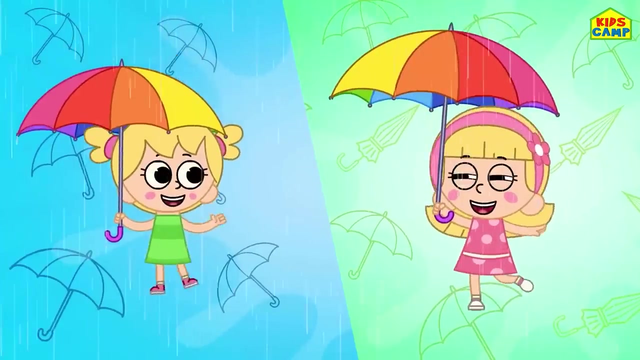 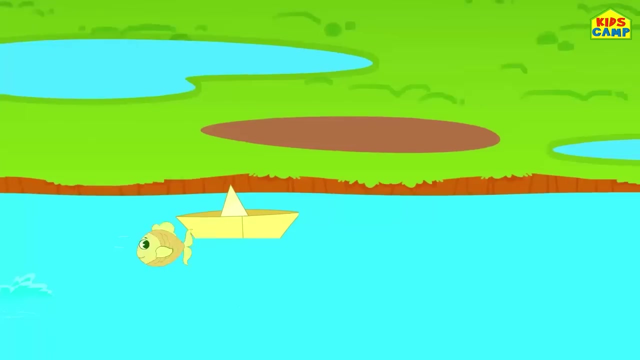 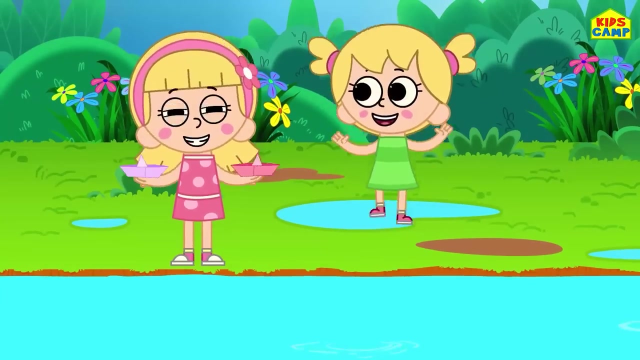 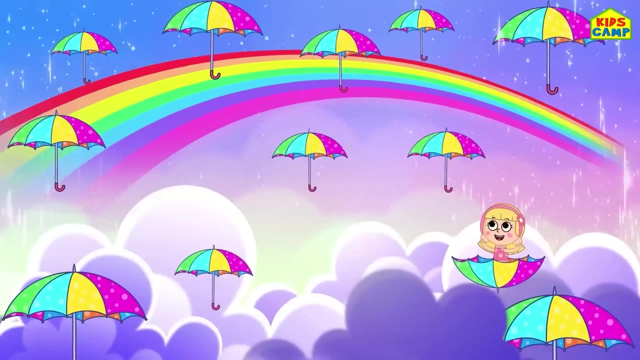 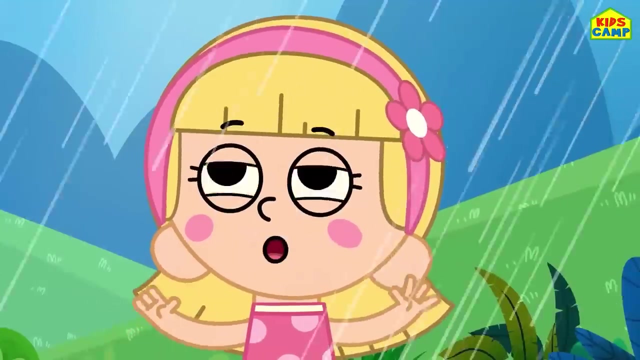 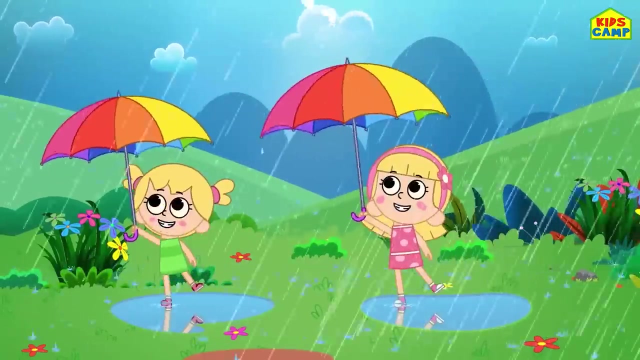 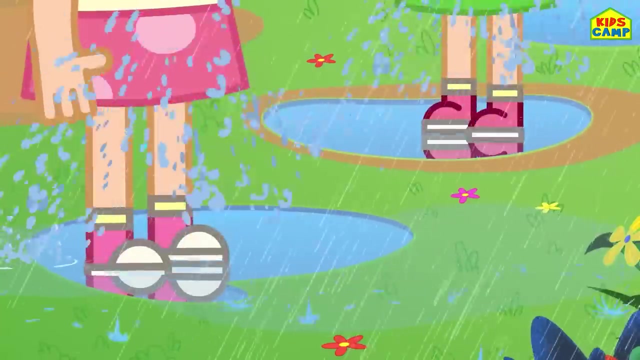